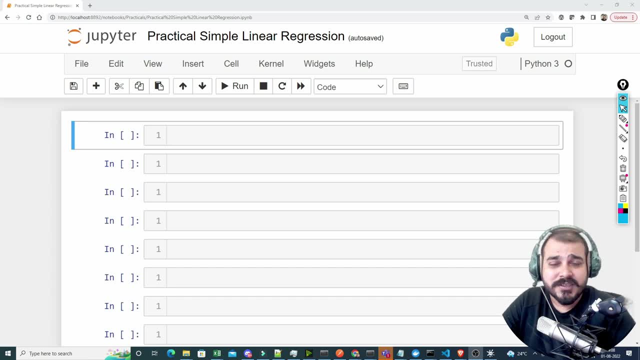 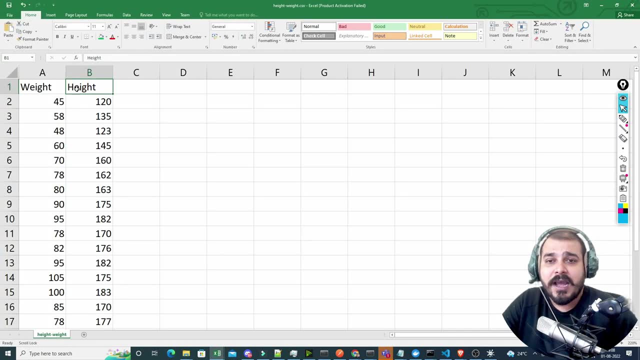 SKlearn implementation and OLS implementation. in this specific video. We will start with a simple project And for this particular project we are just going to take a dataset which has two features. One is weight and height, And here you can see based 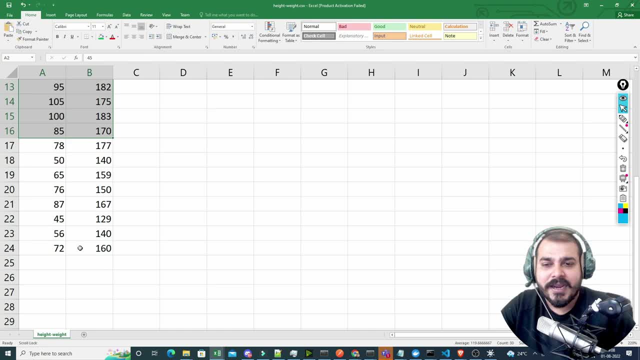 on some weight, there is some different heights, right, And this is my entire data, And I've just taken 24 records. In short, I've just created this dataset by my own And what we are going to do is that, on top of this particular dataset, we'll try to apply a simple linear regression. 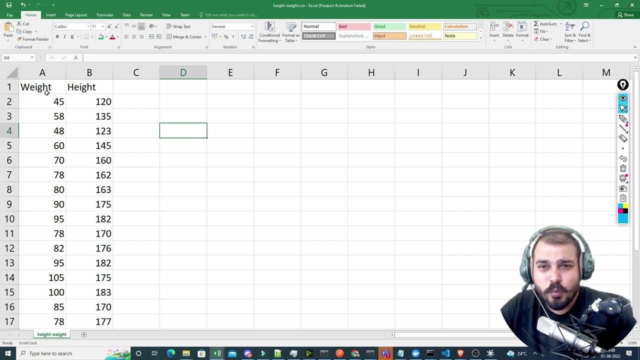 right. And why do I say simple linear regression? Because I just have one independent feature And one dependent feature. So here, weight is basically my independent feature And since I need to predict height, this is my dependent feature. Now, what I'm actually going to do over here is: 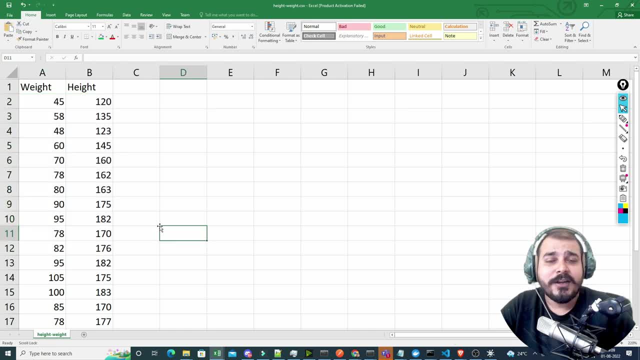 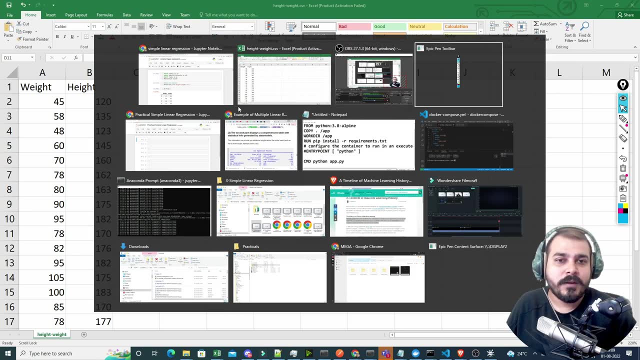 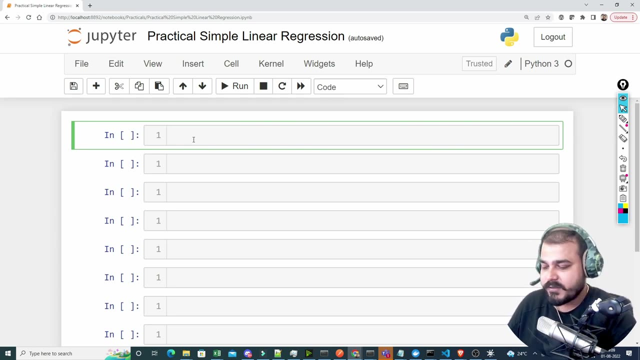 that I'm going to take up this specific dataset and we will try to implement it with using SKlearn. So let's go ahead without wasting any time. So here it is. I'll just open my file. So the first thing is that we will go and implement or import some of the libraries, right? So first of all, 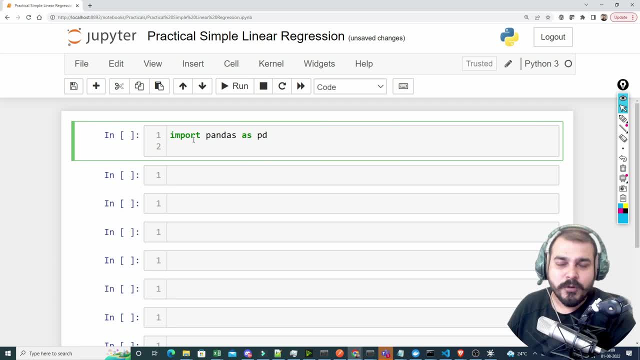 I'm going to import pandas as pd. Pandas is a library which will actually help you to read the dataset from different data sources like Excel, CSV sheet, overall right. And then I'm also going to import matplotlibpyplot as plt. This is for visualization purpose. Apart from this, I'm also 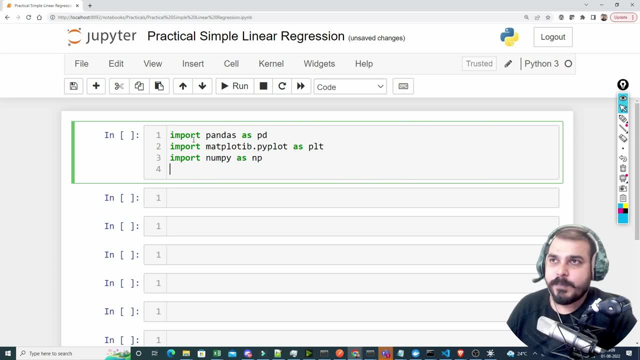 going to import numpy as np, okay, And guys, please remember one thing that if I probably make any mistakes right, I will not, you know, remove that part of the video. The reason is that I really want to keep all the things in this particular video should look like raw, because whatever issues you are going to, 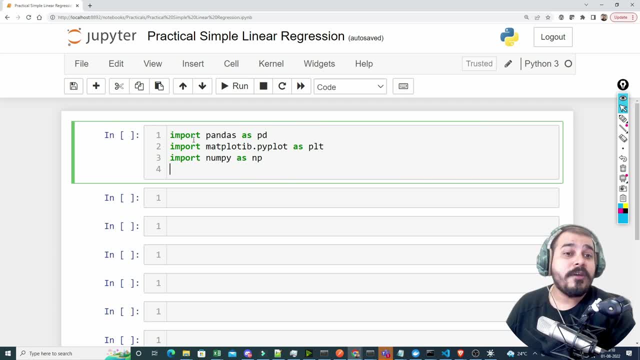 face. it is better that we fix it in front of you, because tomorrow you may be also facing that particular issue. So just a reminder, okay. So next thing, what I'll do, I'll do matplotlib And then I will also say inline so that I can display all my visualization graph within this Jupyter. 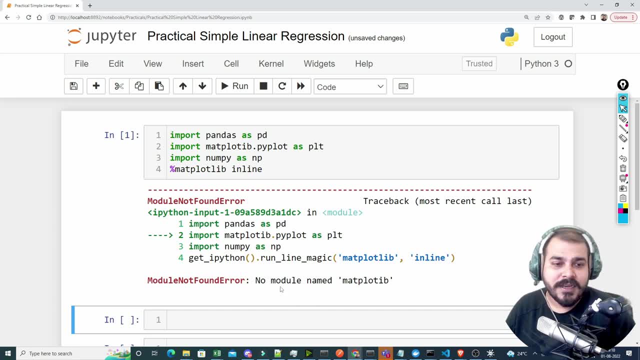 notebook. So let me just go ahead and execute. So it says: first error: no module named matplotlib inline, right? So here, if you see, what did I import? import matplotlibpyplot as plt, right? So let's see why this thing is not executing, okay. 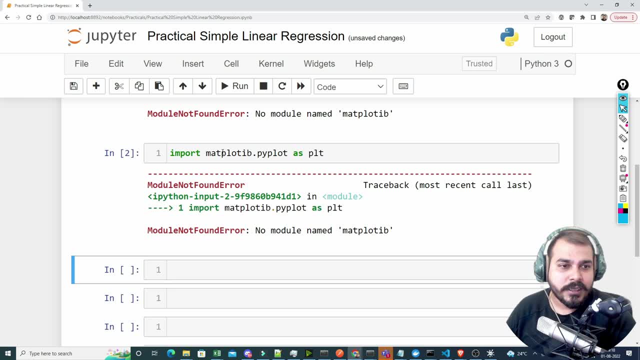 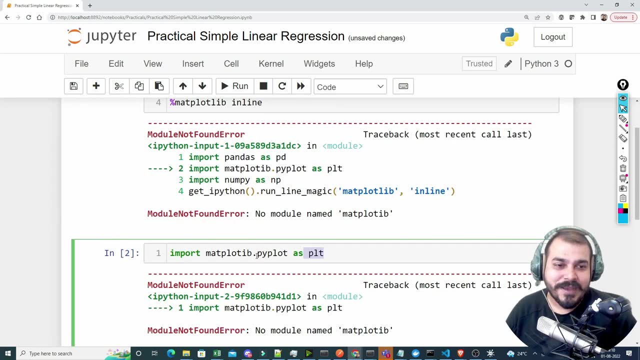 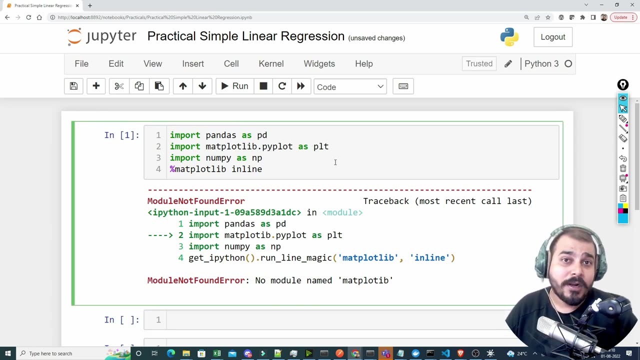 import matplotlibpyplot as plt, Because here you can see clearly I have made one spelling mistake. So that is the reason why I'm saying you, even though I face any kind of issue, I'm not going to remove any part of it, So I'll make it matplotlib. So this is the spelling mistake was. 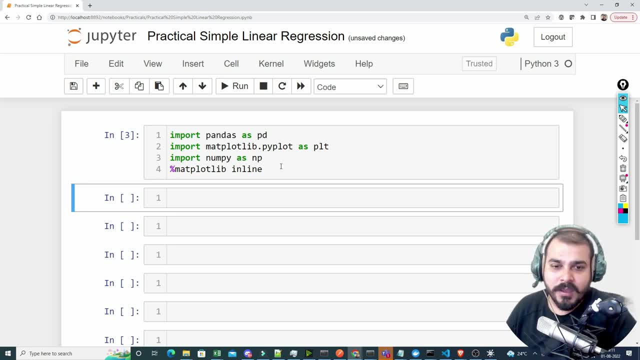 there in this library, So you may also face it. So I'm just going to execute it now. Now, the next thing is that what I'm actually going to do here is that I will be using- I will be reading the datasets Now to read the dataset. what I will do: I will write df And let me just open the. 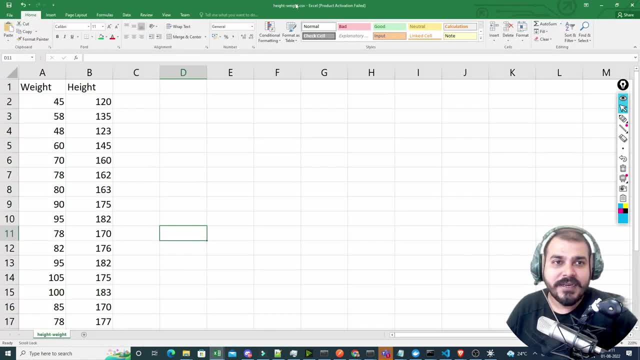 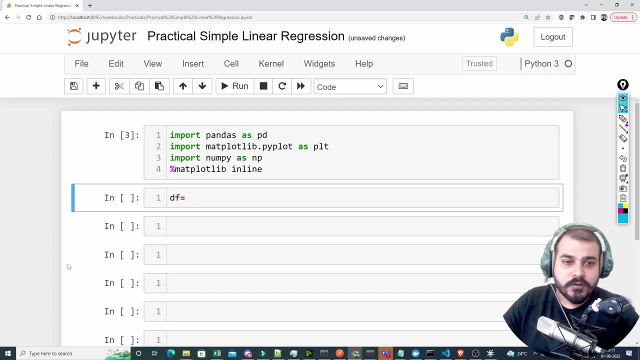 dataset over here And here you can see. the dataset name is height-weightcsv, And this is present in the same folder location where I'm actually working. Okay, So let's go ahead and read this dataset. So I'm going to write pdread underscore, csv And here I will be reading my 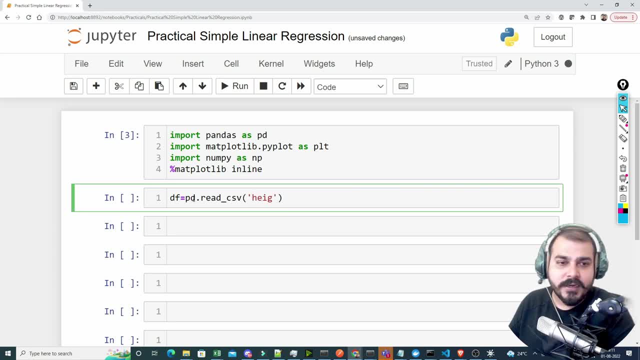 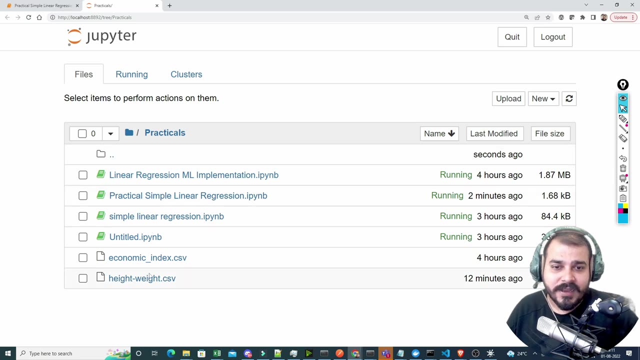 dataset, And my dataset is nothing but height-weightcsv. So if it is already present in this folder location, if I probably go and click on file and open it right, you'll be able to see this particular file. Let me just show you. So right now, these are all the files that I 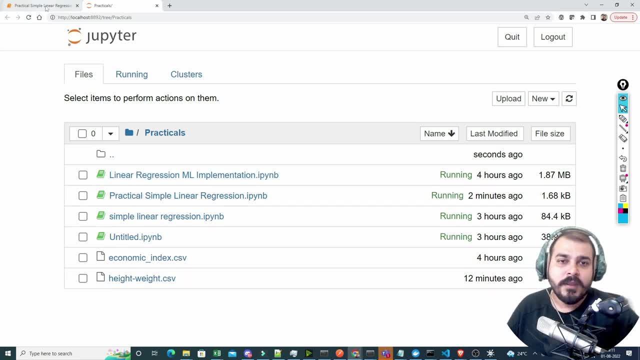 created inside this And here you have height-weightcsv. Okay. So if you are starting this project after you download the file, you know, please make sure that you keep that particular files on that same location. Okay, Now, once I execute this here, now I'm going to. 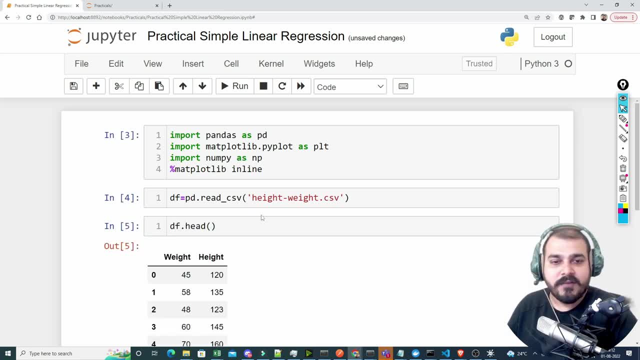 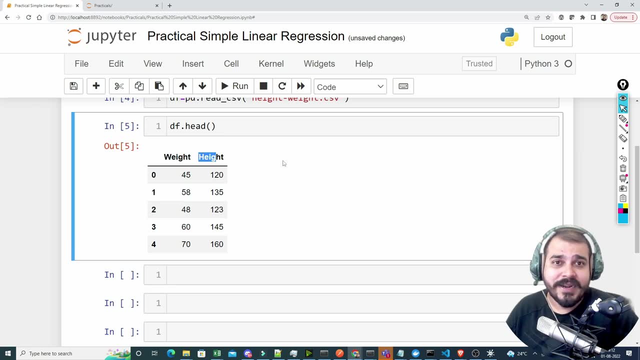 get something called as dfhead. If I see dfhead here, you'll be able to see here. you'll be able to see two: one inputs and one output. that is, weight and height. So these are my two features that I'm going to use, And I'm going to use this one here And I'm going to use this one here. 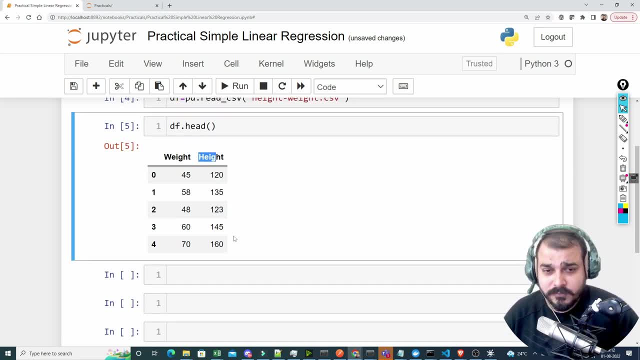 Probably create a simple linear regression. Now, first of all, one thing that you really need to understand: what is the relationship between weight and height? Whenever you are probably creating a simple linear regression, it is very much important to actually check how your 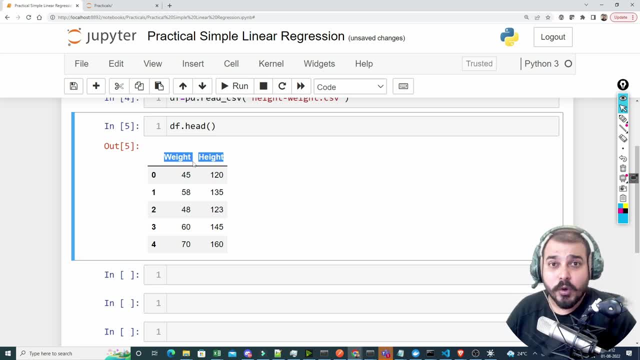 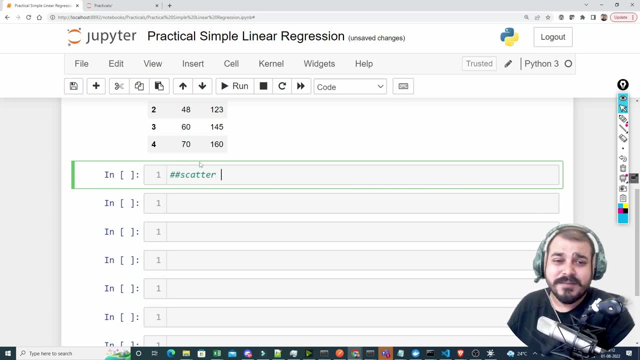 independent and your dependent features are related, whether they are correlated properly or not. Okay, So one way is that I can use some scatter plots. Okay, And here I've taken a simple dataset. guys, You may be thinking: Krish, why are you not doing scatter plots? Well, 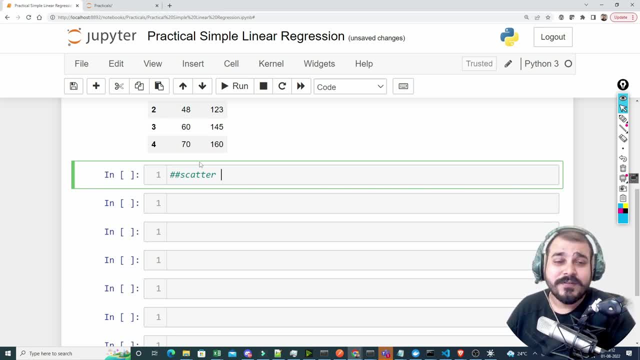 I'm doing feature engineering. Is there any NAND values you have to check or not? Yes, obviously you need to check, but I know in my dataset I don't have any other problem. And this is the first simple project. So I really want to go ahead and show you most of the important steps. 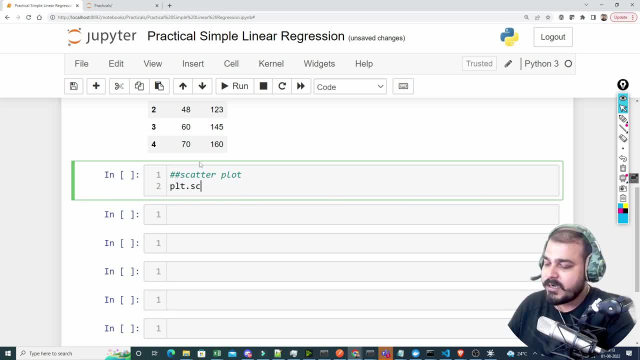 So first of all, I will go ahead with scatter plot. In scatter plot I will be using pltc scatter. So scatter is a function which will actually help you to project your data points with respect to X and Y axis, That is, your weight and height. So I just want to see. 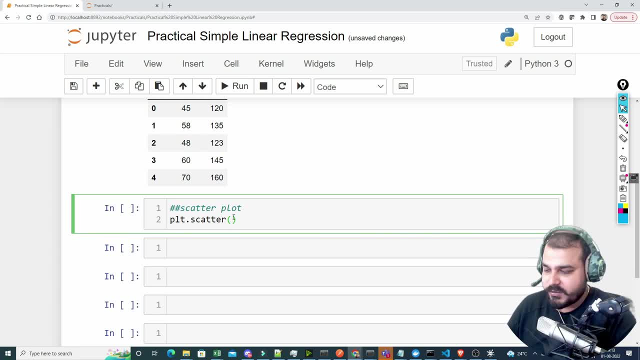 how? what kind of relationship is there? And we scatter the data points. So here I'm going to use df of weight And then I'm also going to use df of height. right, So height, I think it is capital. So height Now, when I display this, 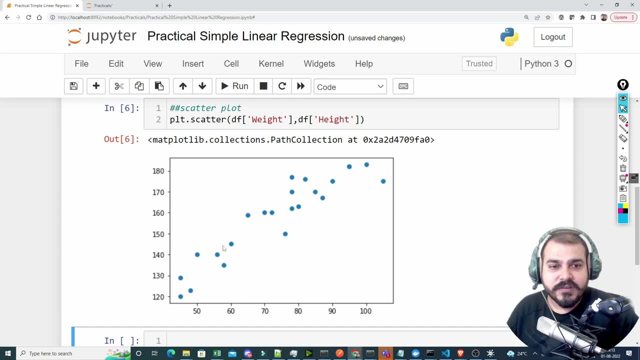 you can see that over here right In this. if you see the specific plot here, you can see on the X axis I've taken df of height right On the Y axis I've taken df of- sorry, in the X axis. 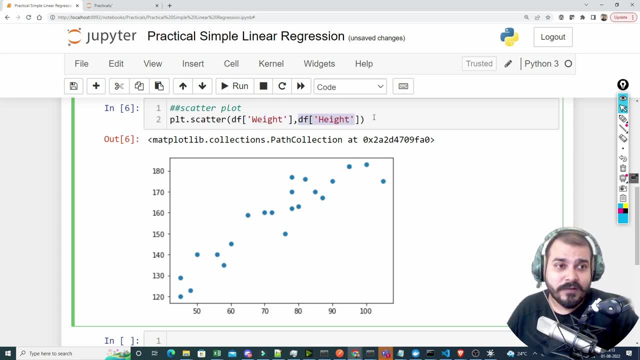 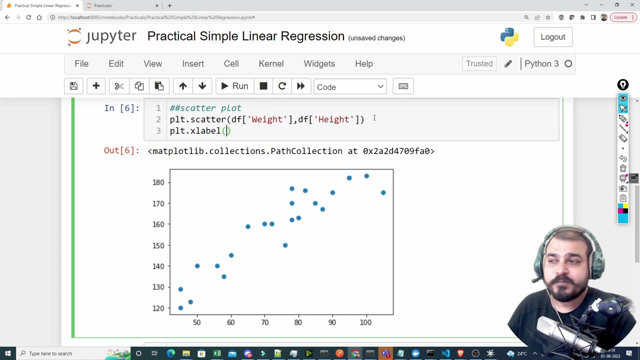 I've actually taken df of weight On the Y axis. I've actually taken df of height. Now let me just put some axis also, So I'll write pltxlabel, Okay, And here I'm basically going to put it as weight. Well, I'm just labeling the X. 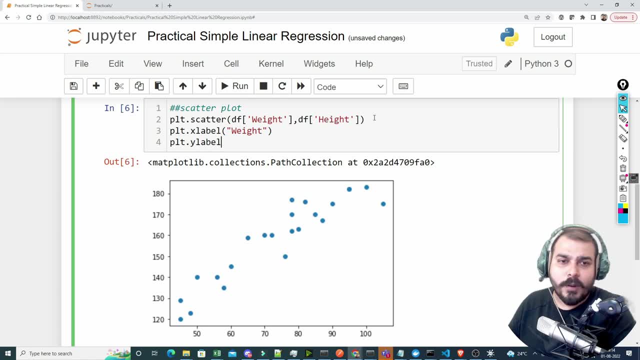 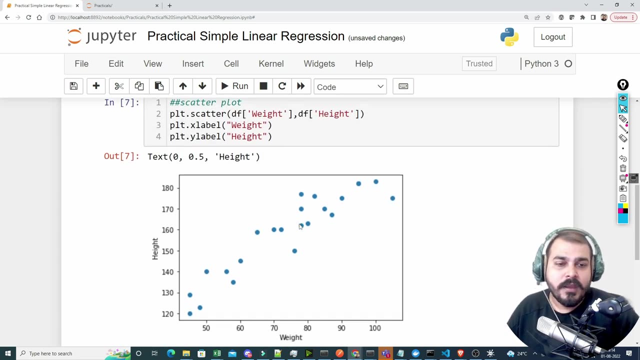 and Y label, So that it'll look better for you. pltylabel. And here is specifically my height. Okay, Let's go ahead and plot it Now. here you can see that in the X axis you are able to see weight and here you are able to see height. Okay, Now, this is perfect. Now, from this particular 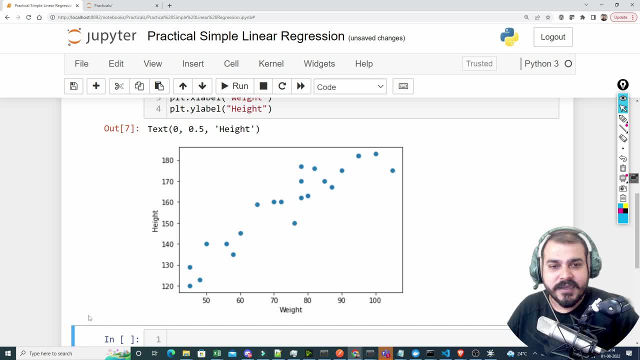 data point. you can obviously see that as the weight is increasing, right, Your height is also increasing. So this is a kind of linear relationship, right. And if you really want to find out whether this relationship is positive or negative, you can also use correlation right. 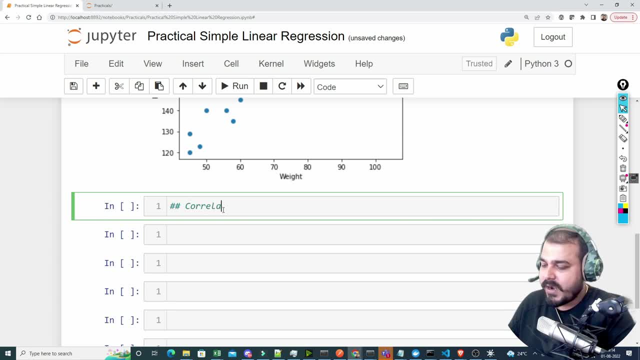 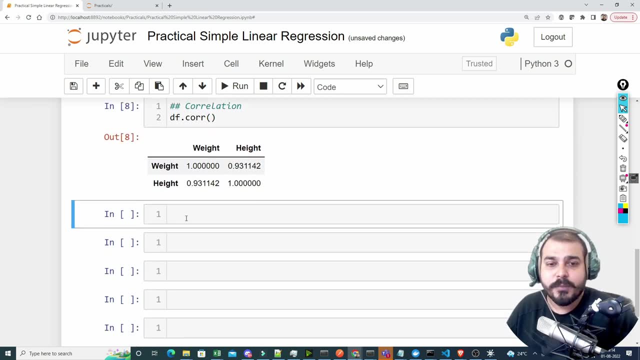 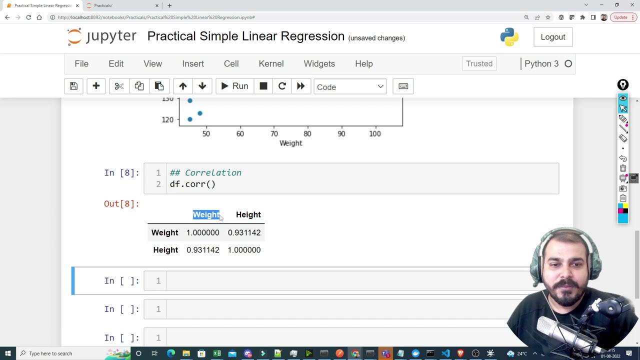 So what I will do? I will just write over here of finding correlation, right? So if I write, dfcorr basically means it will show you the correlation between your X and Y coordinates, that is, your weight and height. Now, here you can see within weight to weight, right, There will hardly be any. 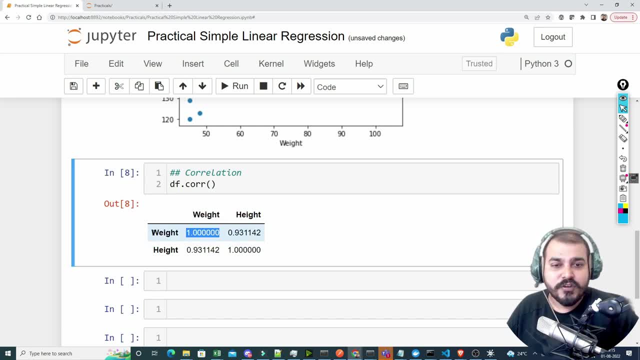 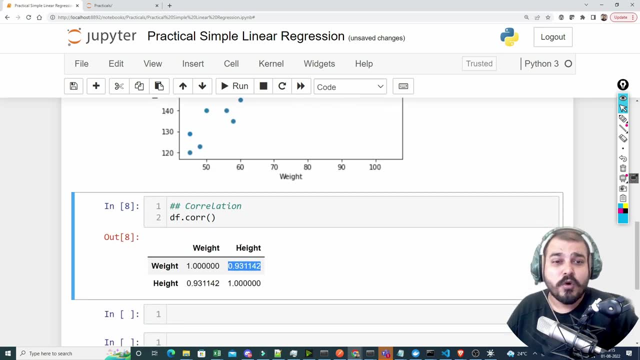 variance right If you try to compare. So this is 1.0. But if you see with respect to the relationship between weight and height, it is 0.93.. That basically means that it is highly positively correlated. because inside this correlation, if I go and press shift tab, the method that is used- 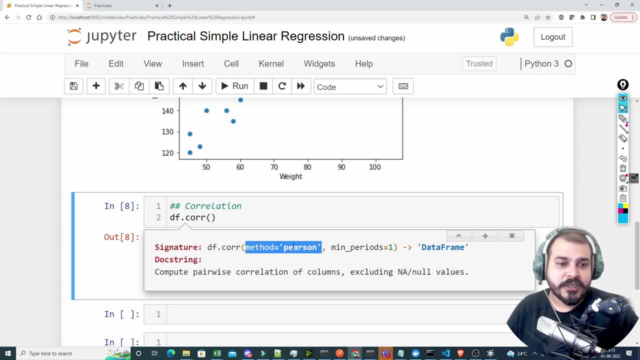 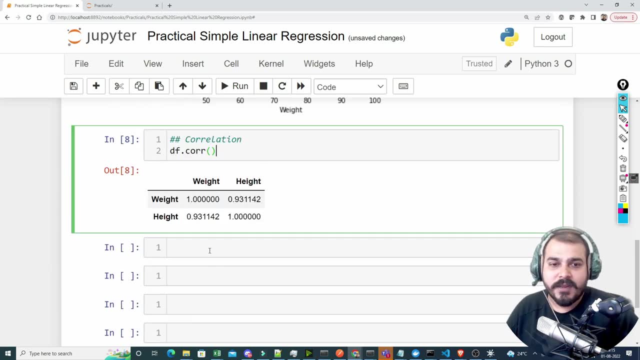 is something called as Pearson correlation. Okay, Pearson correlation, And this Pearson correlation basically finds all the relationship between your X and Y coordinates. Okay, Now, this is perfectly fine. You can also use one library, which is called as Seaborn, for visualization. So let me just show. 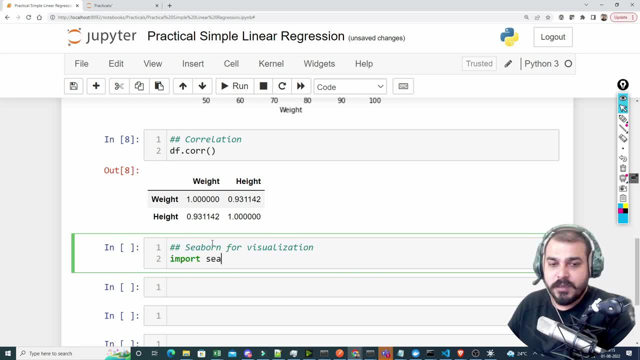 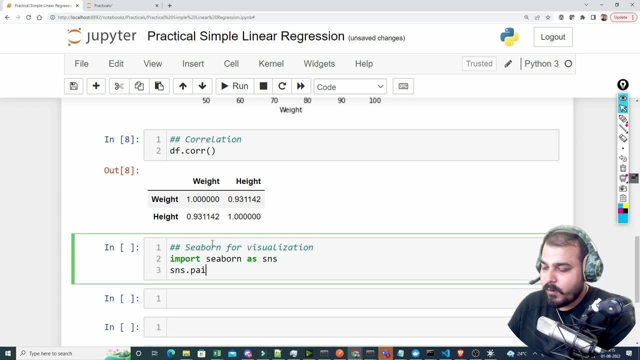 you that, First of all, what I'll do? I will import Seaborn as SNS, right, And here you can write snspairplot. Okay, Now this pairplot. what it will do is that, in a diagrammatically way, it will. 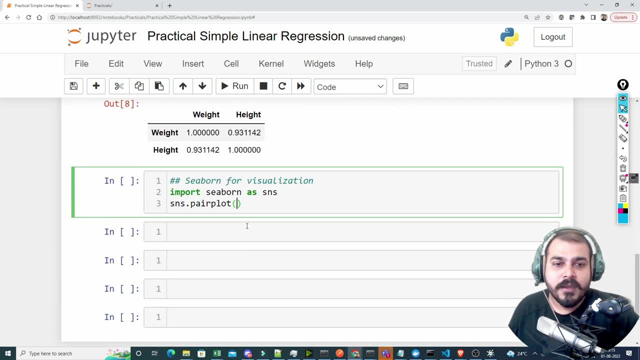 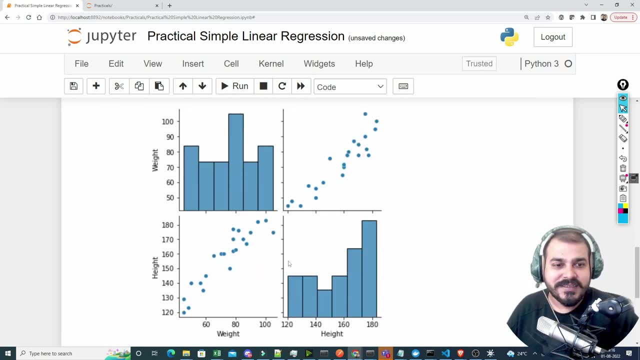 try to show you. it will try to display this pairplot So it will show you the value of the specific coordinates. Okay, So here I'm just going to write DF and just execute it. So here you'll be able to see. the same correlation is basically displayed over here, right And obviously. 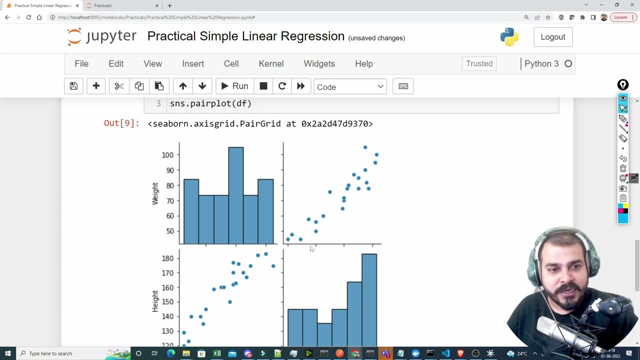 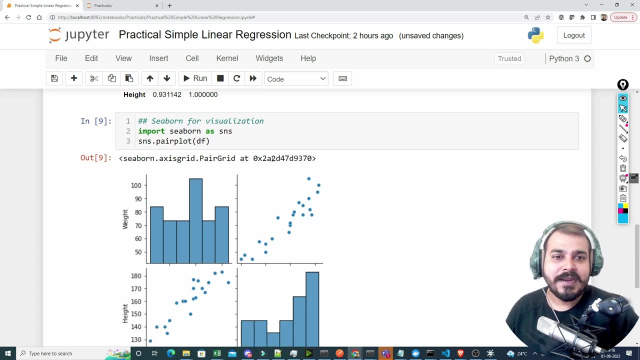 height and weight is positively correlated. It is in a linear correlation and this is also in a linear correlation. Now suppose, if you have something in linear correlation, you get a strong feeling that, yes, linear regression is going to work well. Yes, there may be other problems with. 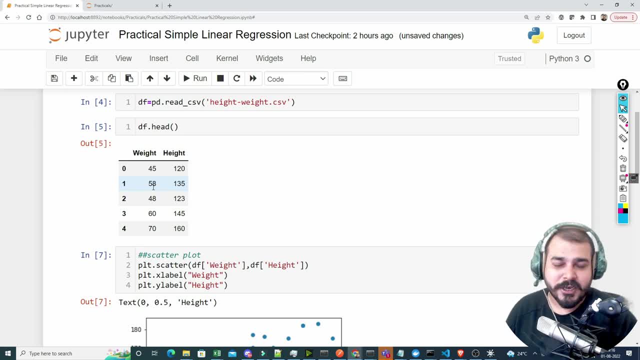 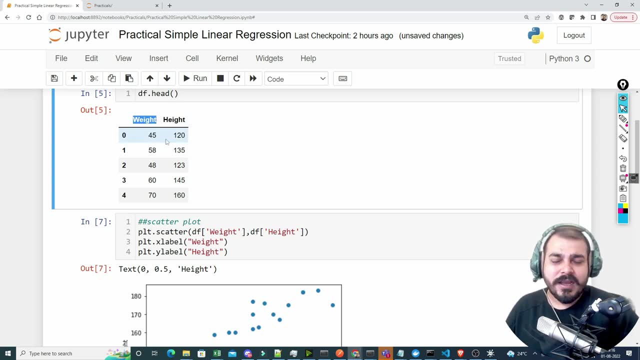 respect to the independent feature. Like usually, when we do multiple linear regression- right, We also check this relationship between the independent feature, right, But right now I just have one independent feature. We will get to know that: how to check multicollinearity and. 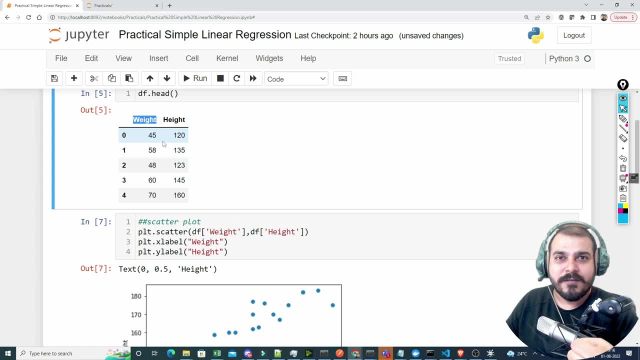 all. Multicollinearity is a scenario wherein if you have two to three independent feature and the correlation between those independent feature are high, then we can neglect those features which are highly correlated. Either of the feature we can basically take Okay, So here let's go ahead with 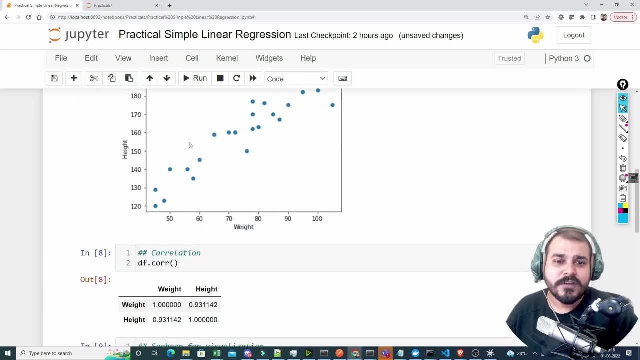 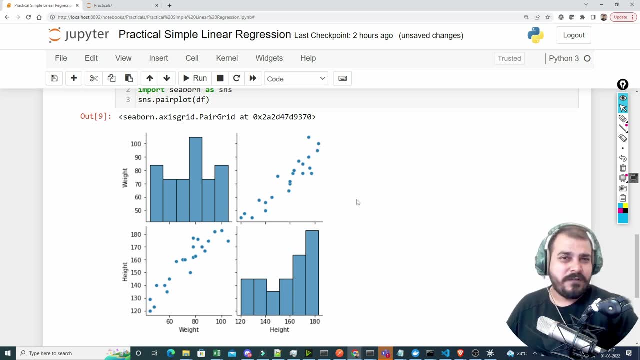 this one right now, because since in my independent feature I just have one, in the output feature I have one, So this is perfectly fine, And here you can see that, okay, it is linearly correlated, So you get a good feeling. 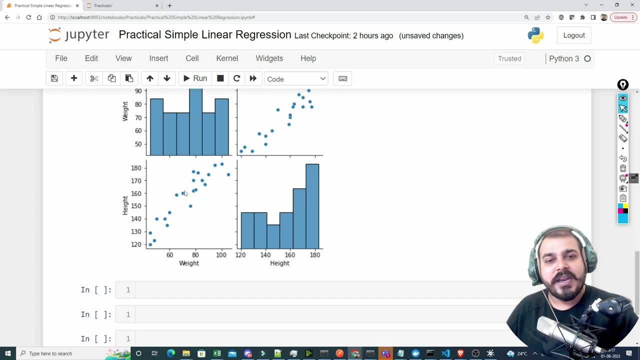 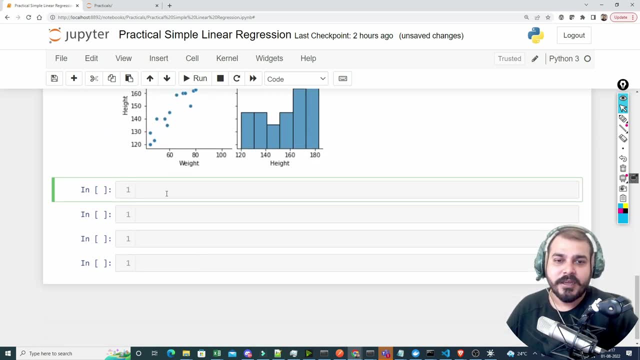 that simple linear regression will work well because at the end of the day, I have to create a best fit line through it. Okay, Now the first step that we probably start in: simple linear regression. Here I'm just going to divide my features into independent and dependent feature. 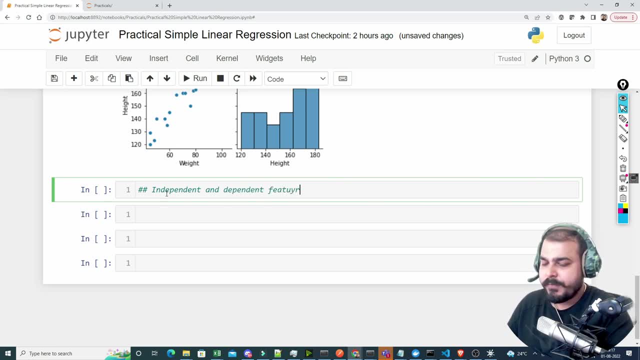 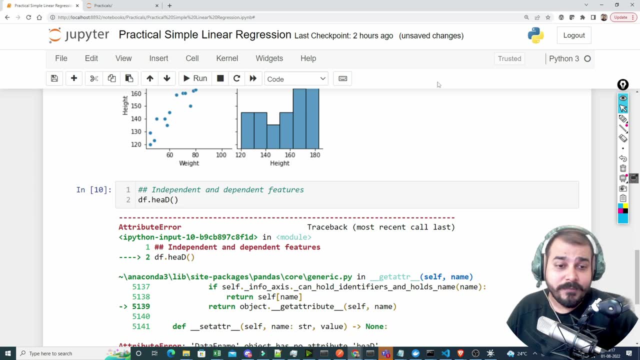 Super important whenever we basically start right Features. Now, if I probably go ahead and display dfhead here, you know that how many features I have Now see this error has come. So don't worry, because I know what is the error I made. So here you have. 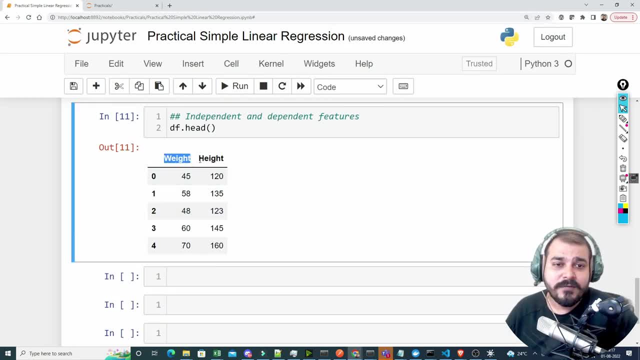 something like weight and height. Okay, Now, this weight is an independent feature and height is your dependent feature. So, in order to create your independent feature, I will just name it as x, just a naming convention. It is a good practice that we should use this kind of naming conventions. 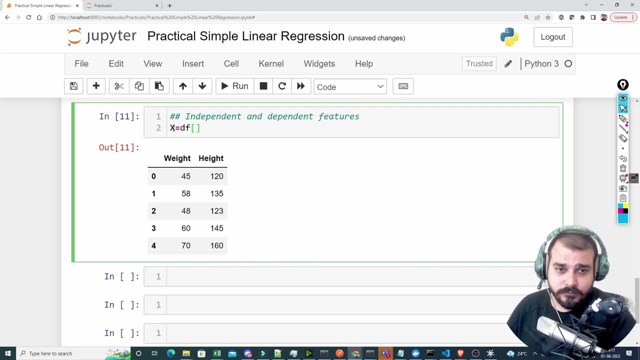 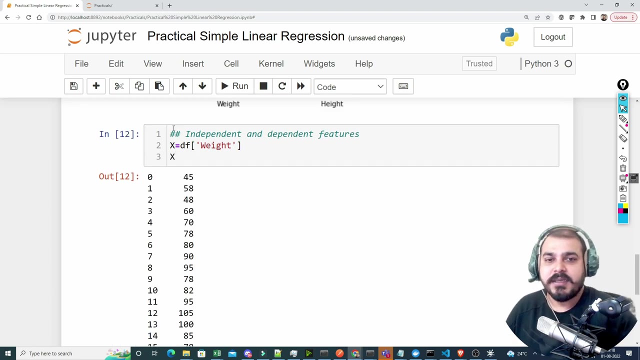 Okay, So x is equal to df of If I want all my weight feature in the x-axis, So I can first of all write like this right. If I probably write like this right, Then the x that is basically getting created is a series. 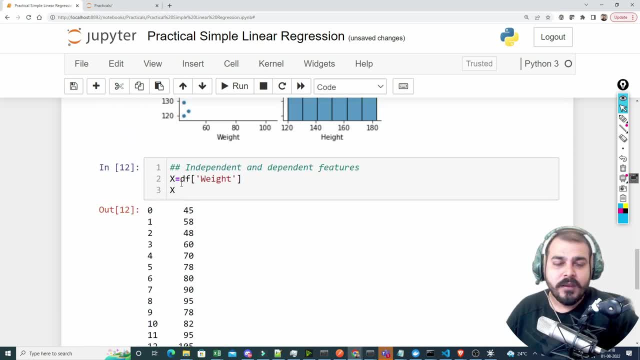 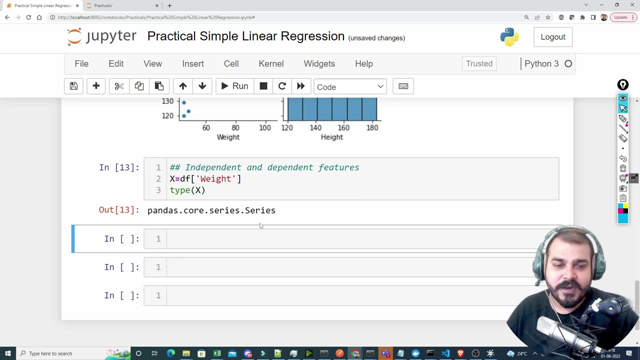 right. So obviously I get my weight value over here right. But understand, if I probably try to see the type of x here, you'll be able to see that it will be a series, not a data frames. right, Data series Now. but if I probably try to see type of df, it basically shows me. 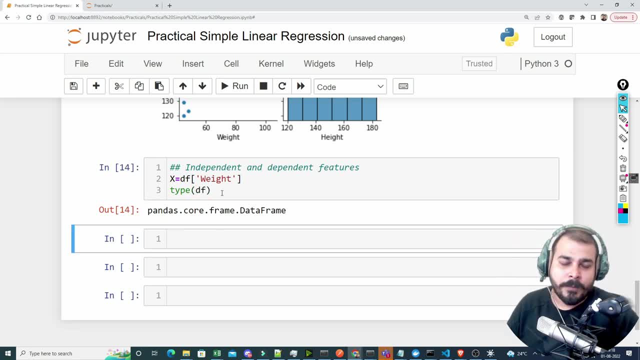 that it is data frame. Now, series basically means just a single record. You have to take care of one important thing, guys: Whenever you probably try to create independent feature, right, And if I use one additional bracket, then what will happen is that just see this okay. 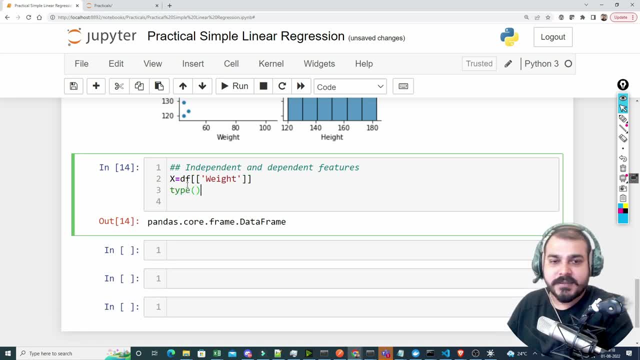 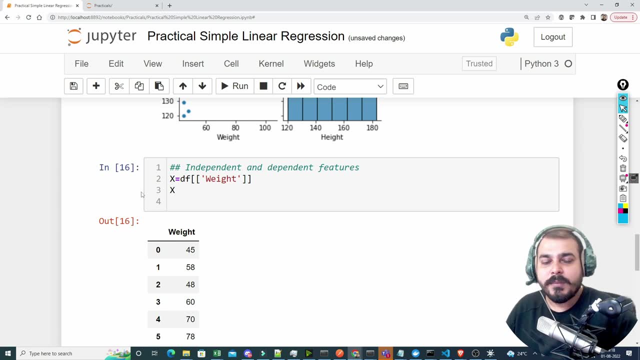 If I go and execute this like this and if I write type of x. now you know that we will try to get a data frame right And probably if I try to execute this here, you'll be able to see. 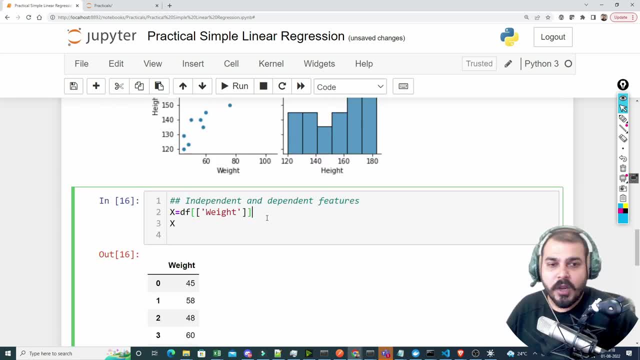 that I'm getting a data frame with column name. Always make sure that your independent feature right Should be in the form of data frame or two-dimensional array. okay, Independent. yeah, I'm writing it over here because this will be super important when you're training your model. 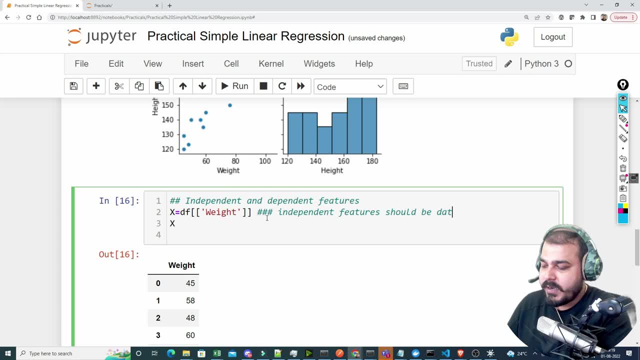 So your independent feature should be data frame or it can also be two-dimensional array. When I say two-dimensional array, what does this basically mean? This basically means I can have something like this: See, Suppose, if I write like this: okay, And now probably let's say, I'm going to write nparray. 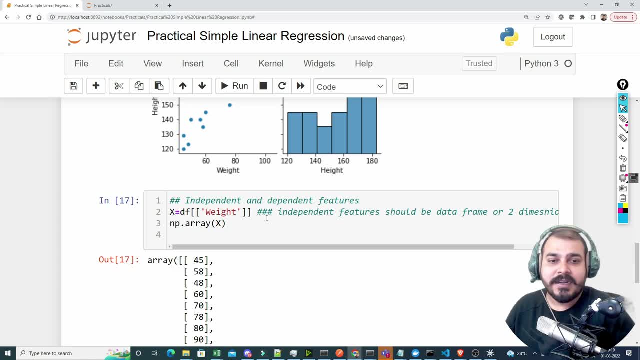 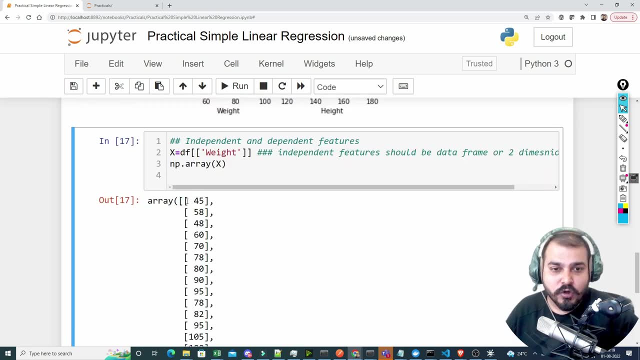 okay, And I'll probably write x. okay. Now, if I write like this here, you can see that it is a two-dimensional array. okay, Two-dimensional array, And this basically indicates that how many rows I have, I have one, two, three. Let's just see how many rows I have For seeing how many rows I can. 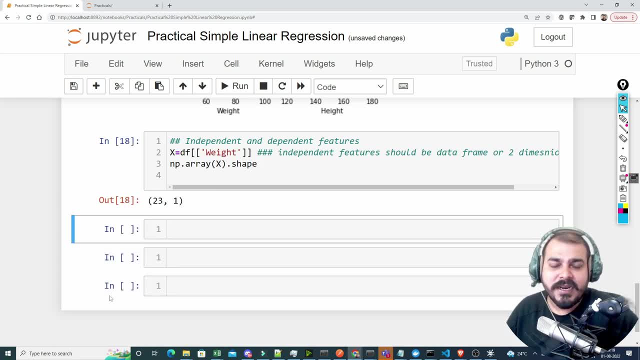 basically go and execute shape. So if I write dot shape here, you can see that it basically has 23 rows and one column. Okay, But in data frame what was happening? Let's see In data frame what used to happen. Suppose if I go. 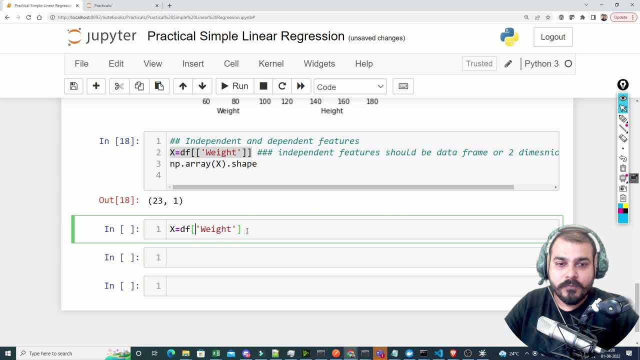 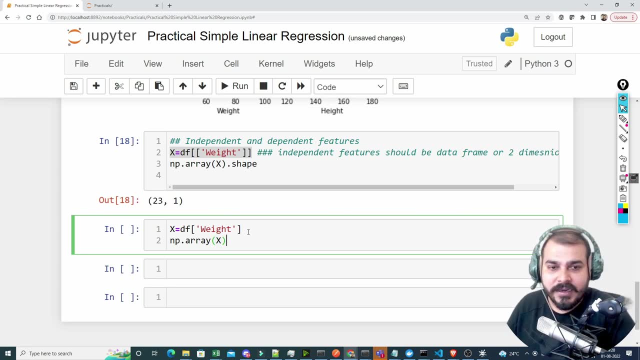 and execute like this and I remove this one bracket. okay, And probably, if I write nparray right, I'm probably just go and see x and then write dot shape. So here you'll be seeing that this will be a one-dimensional array. Here no information regarding the column is given, But 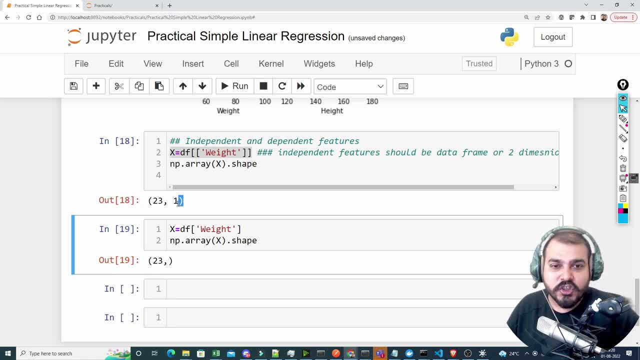 here importance should be given to the column right. So always make sure that, at the end of the day, either it should be a data frame or it should be a two-dimensional array. So here you'll be seeing a data frame which has one column, or it can be a two-dimensional array, also with number of. 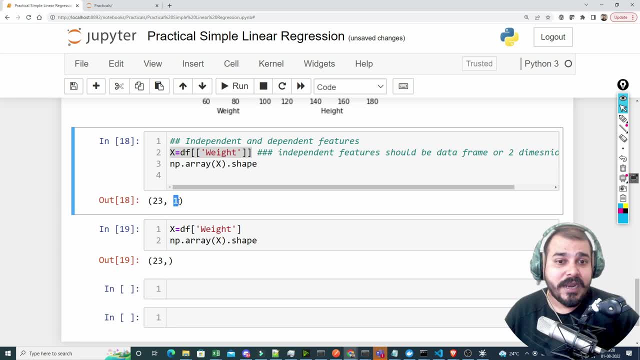 rows and some specific columns. right Now, in multilinear regression. what will happen? These columns will increase. okay, Never keep in this particular format, because what will happen I'll tell you. okay, Let me just say that I am just writing this as x underscore series. I will try to train with this and 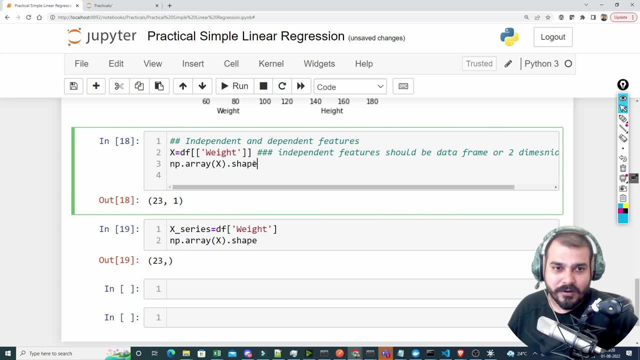 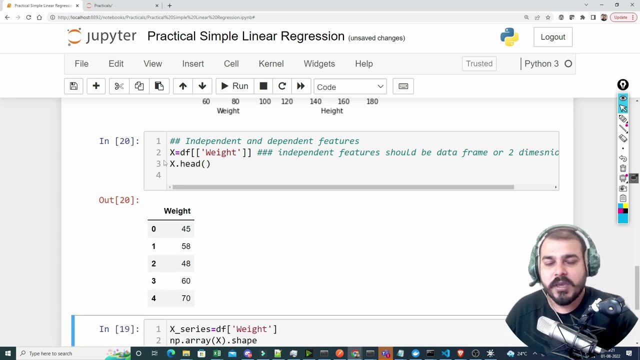 also. I'll try to train with that also And let's see where we'll get an error. okay, So over here now this is my x. Obviously I've taken this as a two-dimensional Data frame which has one column, And then, if I probably go and write x dot head, you'll be able to see I will be getting this specific value, okay. 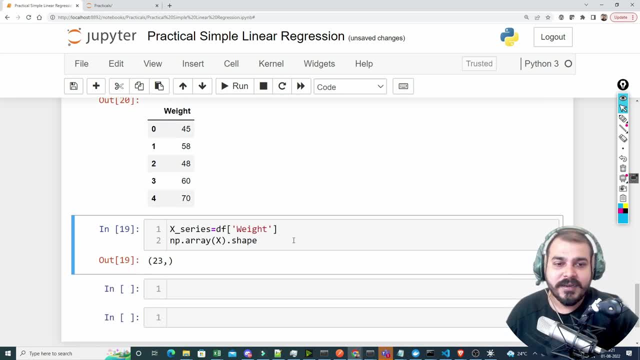 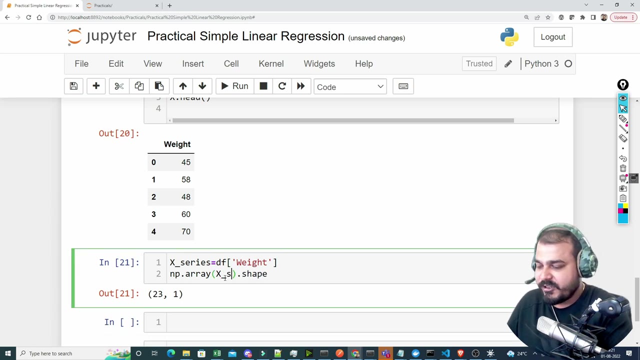 So this is my x Perfect. Now, till here we have executed and let's go ahead and execute this also. And you know that probably, if I also see, okay, df of weight, what happened np dot array? Oh, I have to check it in x underscore series. okay, Now, here you can see it is one-dimension. 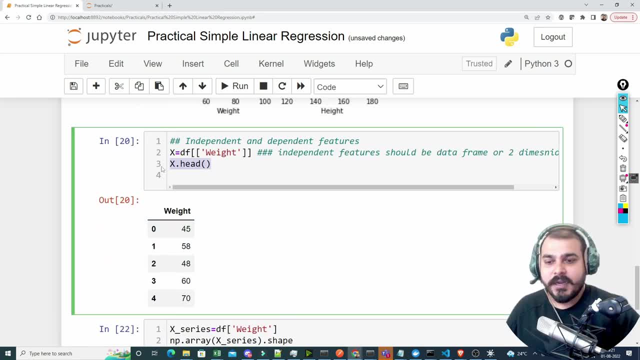 Perfect, This is done. Now the next thing is that, after creating an independent feature, I have to create dependent feature. Now, in the case of dependent feature, I can have it as a series. okay, Because dependent feature will only be one column values. right, We don't have to worry much. 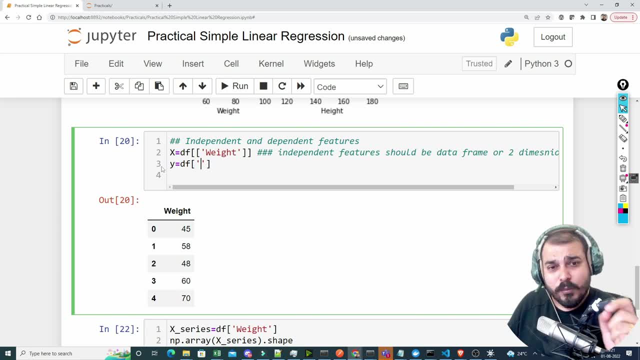 about that, but we do not have to make it two-dimension okay. One-dimension is properly fine in this, because we will have only one dependent feature in a specific problem statement, and this is a regression problem statement. Why do we say: 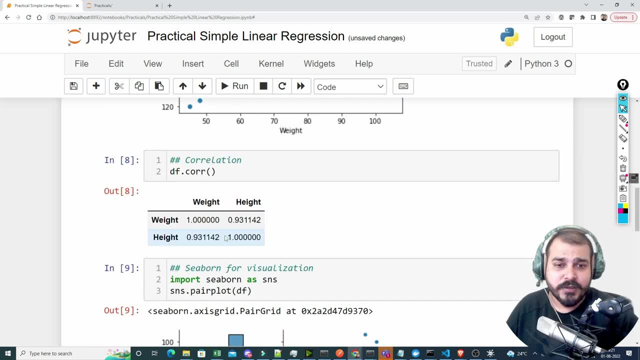 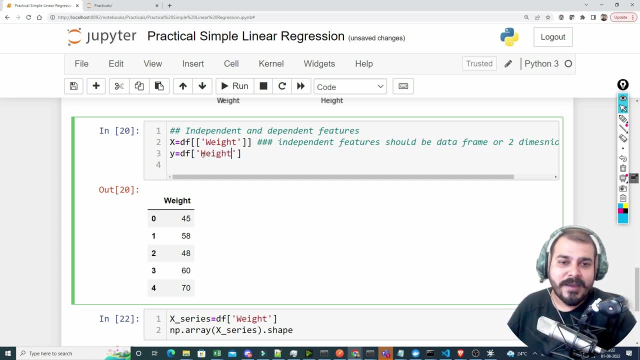 this as a regression problem statement, Because here my output value is continuous. okay, Super important point. Now, here I am going to basically write df of height. Now, this is my y and this is my x. Let's go ahead and execute Now. if you want to see your y, 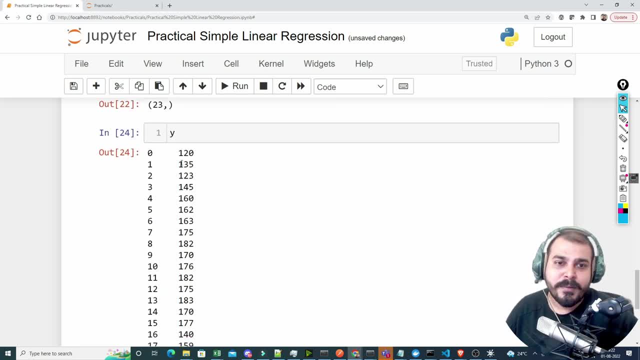 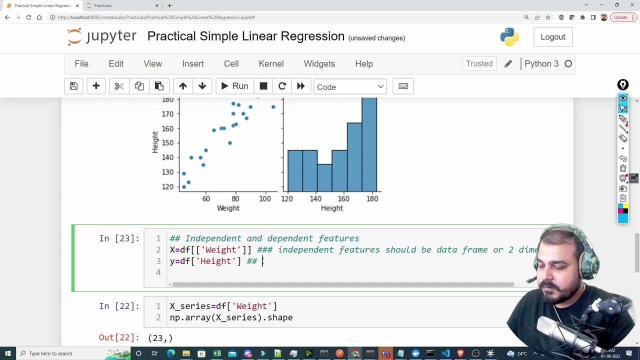 here is my output feature. right With respect to this, And always remember this needs to be in series or it can be in one-dimension. okay, So here I am going to write it down over here: This variable can be in series. 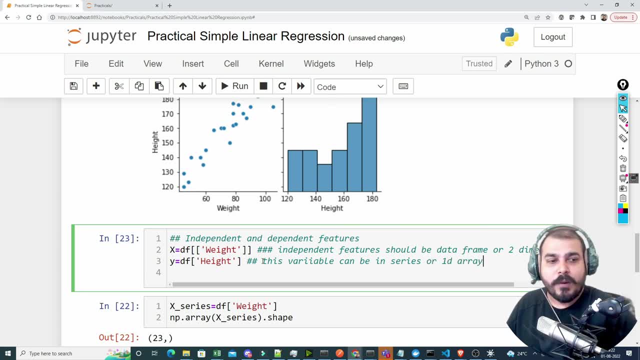 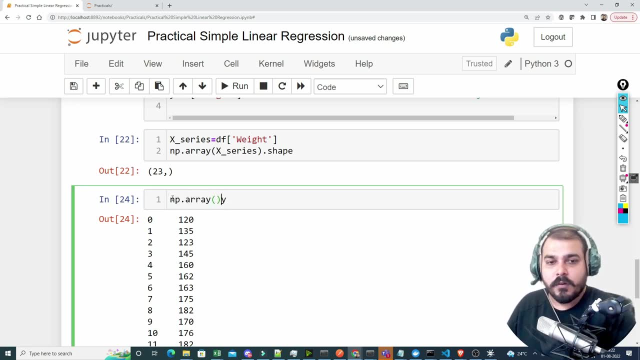 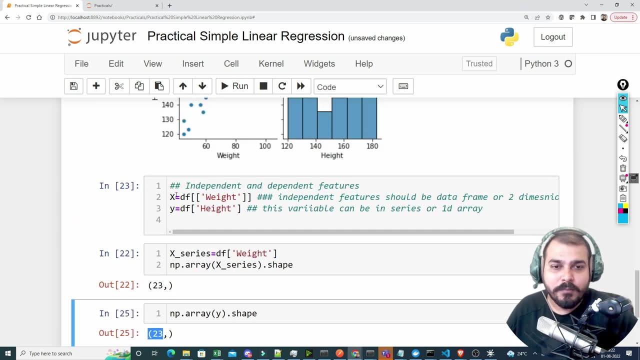 form or one-dimension d array: okay, 1d array basically means, if i probably write np dot array of y, okay, dot shape. here you'll be able to see only one array, so obviously 23. since you have 23 inputs, you have 23 outputs, right? so this is super important. so, and this is very much important, guys, otherwise, 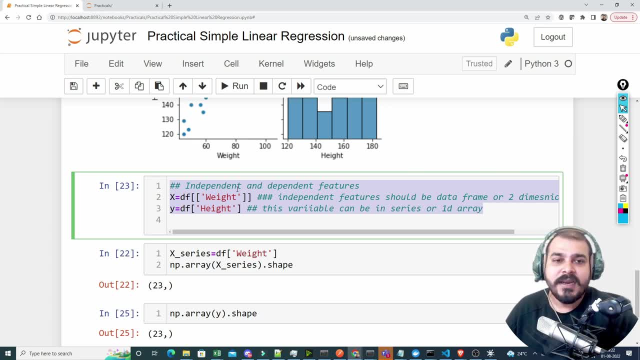 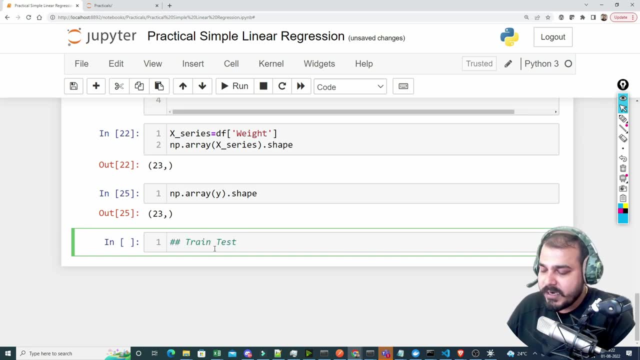 at the last you'll face some issues, okay. so here i've actually done my independent dependent feature. the next step: we specifically have to do something called as train test split, and i have already explained why you need to do train test split. this is for the overfitting. 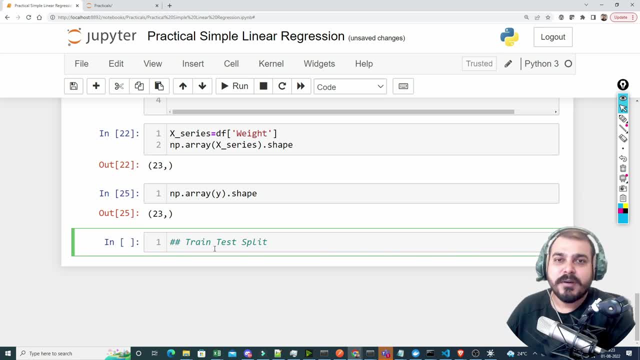 underfitting condition. the train data only will be using for training purpose and the test data will just be used for checking how the model is predicting for the new data point. so for this we will be using a library from sklearn dot action. so i'm going to import train test split. 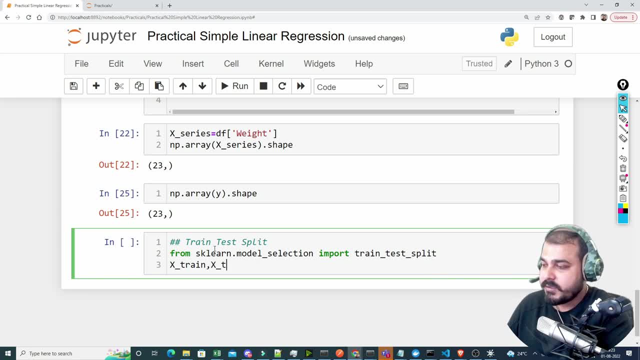 and here i'm going to use x train or x test, y train, y test. that basically means i'm creating a train data and with respect to that particular train data, see train and test. so training data will use the model for training that specific data, for testing that model or for seeing that. 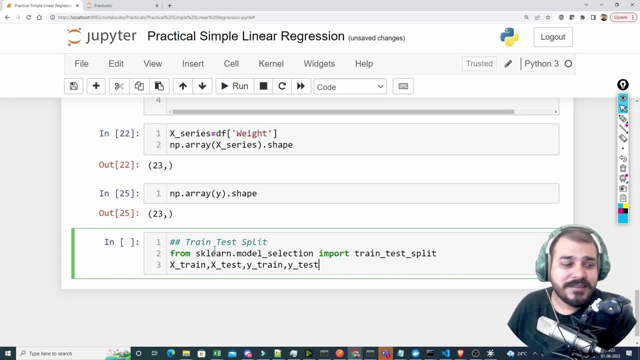 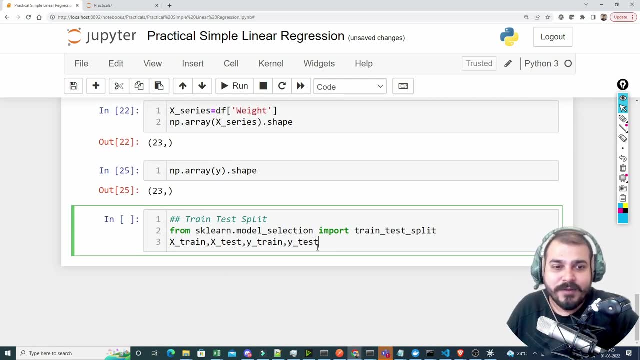 how the model is performing, for the new data will only use test data, so that is the reason we are creating these four components. initially we just had two components. one is x and y, but obviously we need to create x train, x test, y train, y test with respect to the output of x train. it will be: 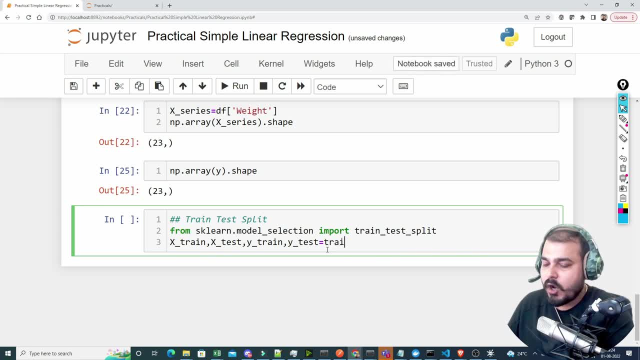 present in y train. okay, so this four parameters will get called when we use the strain test split and internally we'll give x comma y. let's say i'm giving my test size as 25. okay, so in order to give test size as 25, i will write 0.25. now how do you think i've got to know all these things? just go. 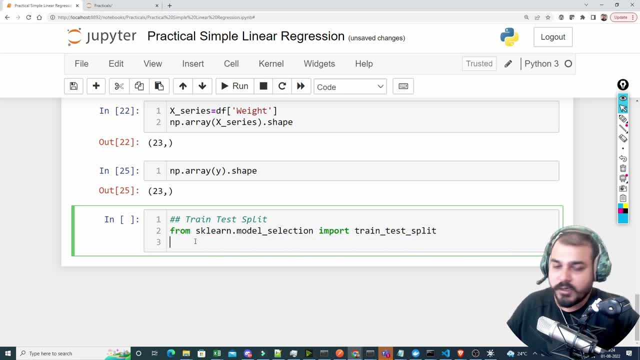 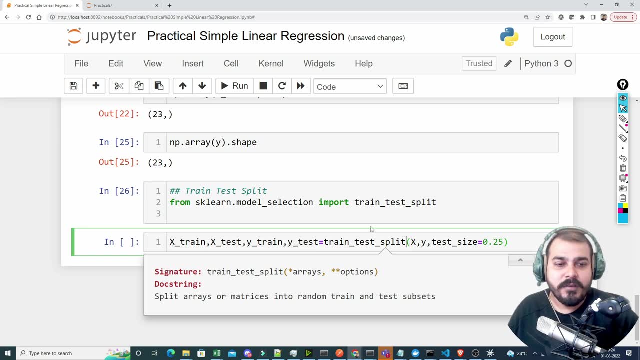 and press shift tab. okay, so here this, then only you'll be able to see it. okay, so here you'll be able to see. i have just imported this and now, if i press shift tab, here you'll be able to see. or the arrays: uh, over here you. 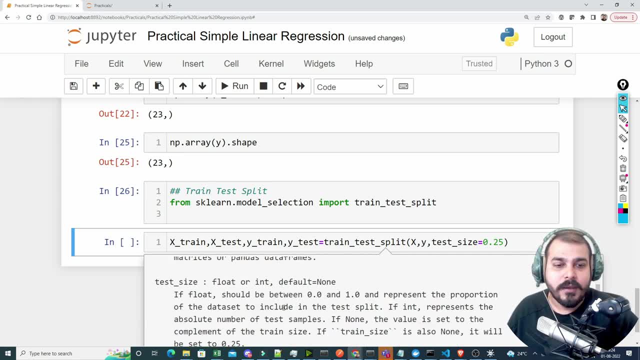 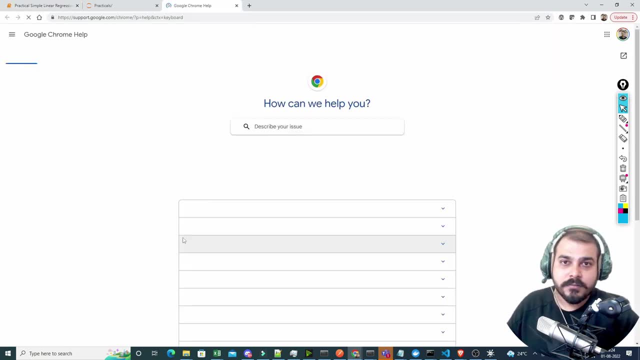 can see test size. i've given the arrays basically means x and y array, train size also you can give, and there is also something called as random state. but before this let me make some cells. just a second i pressed f1, that should not happen. now let me just go and make more cells. 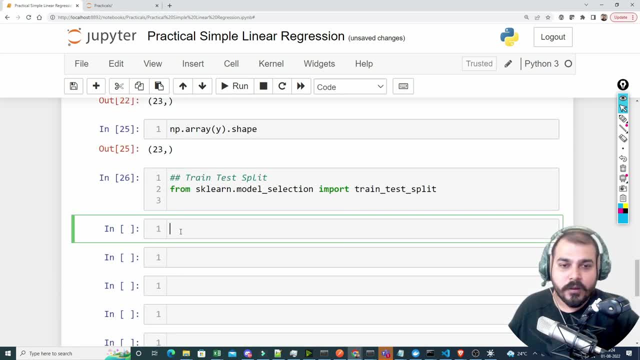 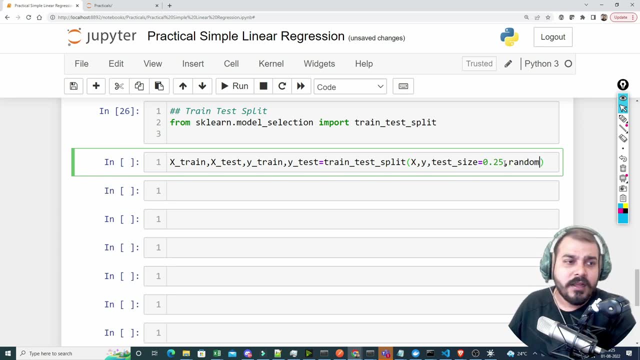 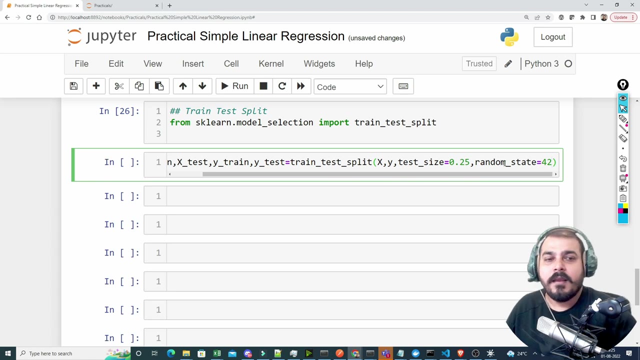 so i'll just copy this entire thing and i'll put it over here. okay, perfect. now understand one thing over here, guys, there is something called as random state. now see, usually when we basically take this random state- let's say, i'm going to take 42, the type of train test plate- if you don't put this, 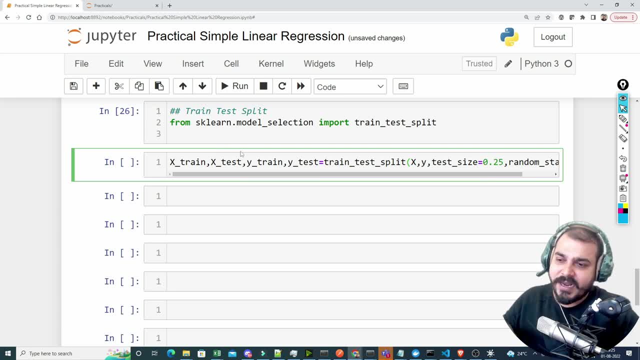 random state right for everybody. it will be a different kind of train test plate. we can randomly put, pick up the record, 75 percent of the record, and put that in the training data set. and we can put: we can randomly pick up the 25 percentage of the record and put in the test data set right. 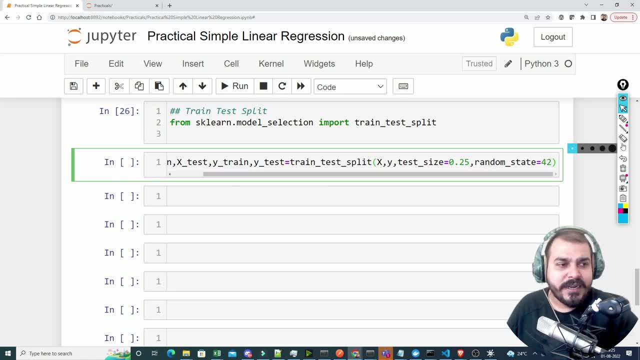 so that is what usually basically happens in this case. so if you write a random state as 42, so whatever way it is basically taking me, like taking my data and putting in the training data set, similarly for you also, that training data reset will get selected. so once i execute it, 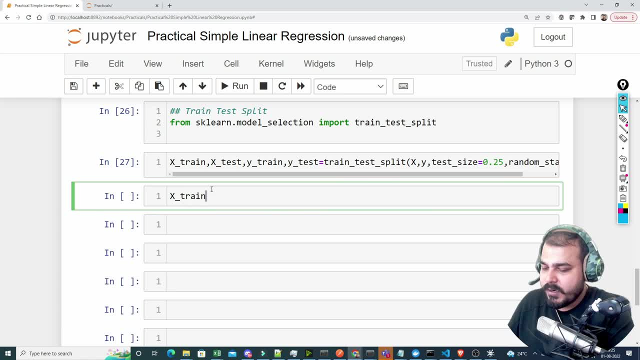 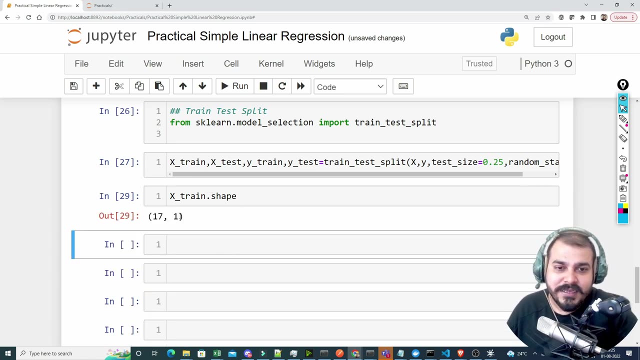 so, here you can see, now i will be able to see my x twin and i will just print the shape also and obviously remember the shape should be two dimension, okay, okay. two dimension, okay, extreme dot shape. sorry, i don't have to use this. and since, here you can see, this is two dimension, right, that basically means this one is because of: 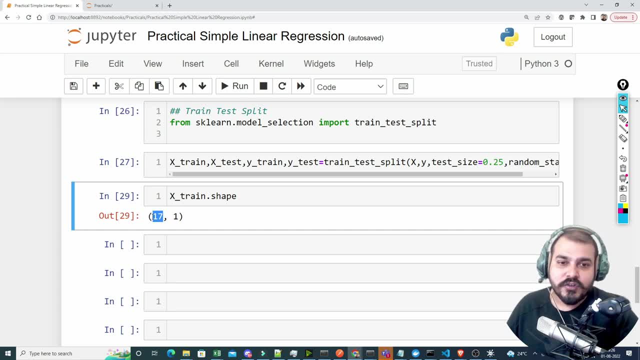 i have one feature and these are 17 rows, right, so 17 rows and one feature. similarly, if you have five feature, then this will become five features. okay, like that it will happen. okay, but at the end of the day, you will be getting a two dimension. perfect, now let's go ahead and let's uh discuss. 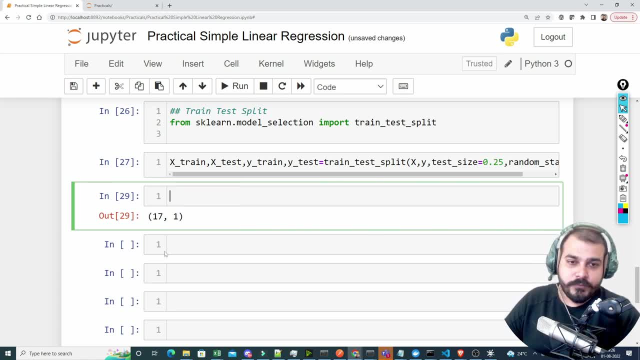 what we have to do after this. okay, now we have to perform a very important step, which is called as standardization- standardization- why it is basically required. now, just understand, guys. i'm also going to write in front of you. let's say i have two features, x and y. let's say x is calculated. 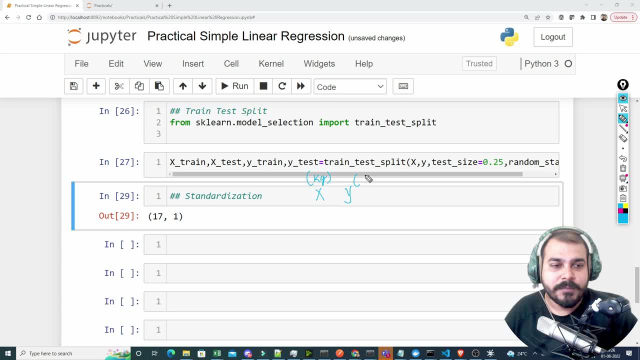 based on kg units. y is calculated based on some other units, let's say over here. in this particular case, since this is height, i'm going to use centimeter. okay, now, it's going to be a straight line. so what i'm going to do is just 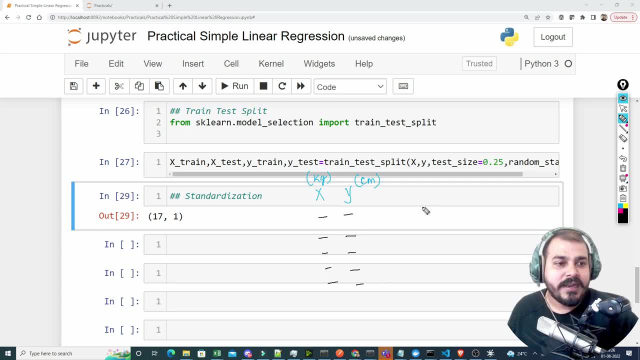 i'm going to use a gradient descent to solve this problem. you have to understand one thing: whatever values you get over here, right, these are of different units and you know that in linear regression when we use a scalar, we use something called as gradient descent. so obviously, based on this unit, if this value is higher, to come to the global minima right. 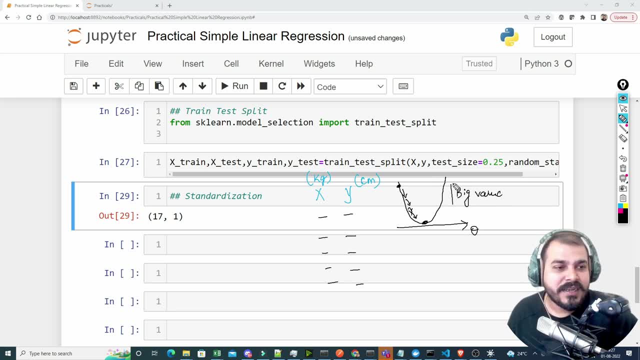 it is going to take time, right, because i have a bigger value and all the maths equation that is getting applied. it will get applied to a big value, right, which is again not a suitable solution. okay, and obviously for the optimization problem will not be a problem because you will use it be a bigger value, right? so whatever values you decide, it will not be a problem. 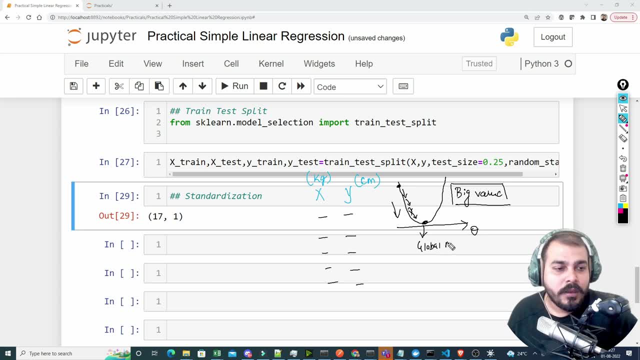 take long time to reach the global minimum. okay, so what we do is that? a very good approach is that we take up each feature, not the output feature. we take up each independent feature and we apply a simple formula which is called as z score, and this formula will basically be converting all your 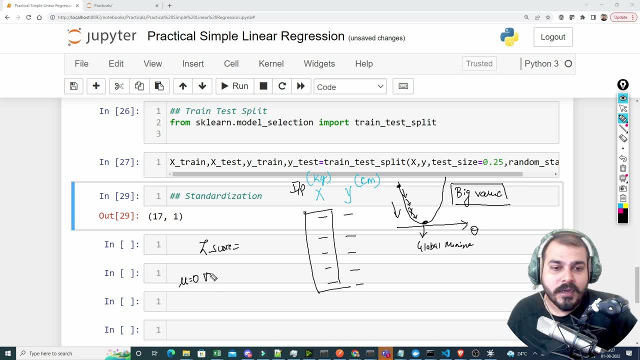 values with mean is equal to 0 and standard deviation equal to 1. okay, that basically means if i take up all these data points, i will write x of i minus mu divided by standard division. only this formula gets applied to all data points. so at the end of the day, what will happen is that 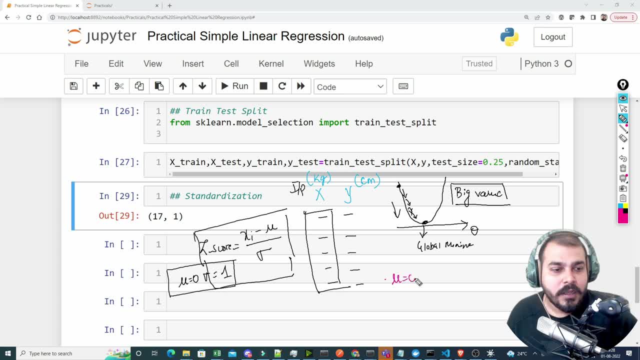 my mean, all these data points will get converted with. mean is equal to 0 and standard deviation equal to 1.. super, super important, okay, so please make sure that you remember this. uh, and this is a very good step with respect to standardization. in the upcoming future, i will also talk about 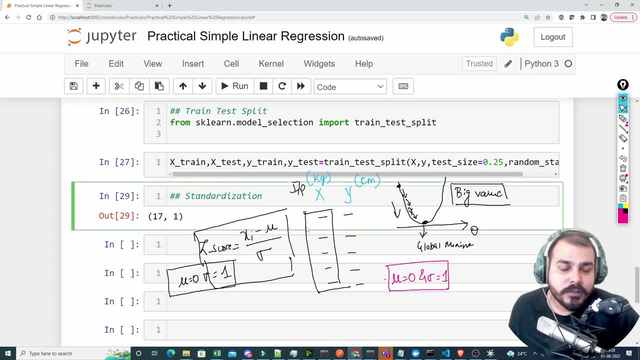 which all algorithm you not apply feature. uh, you, you need not apply standardization. okay, that part also. i will try to discuss. okay, now, what i'm actually going to do and rub this and let's apply standardization. now for standardization again, we will be using an sklearn library. see, guys, every. 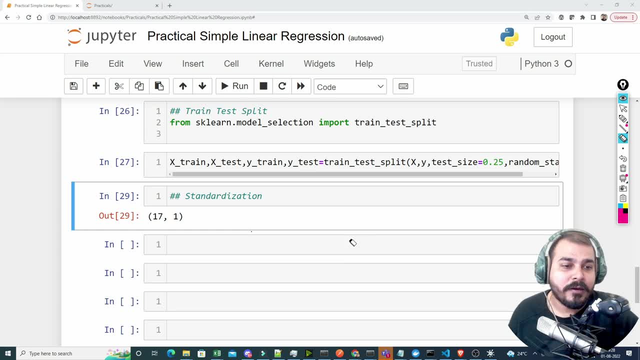 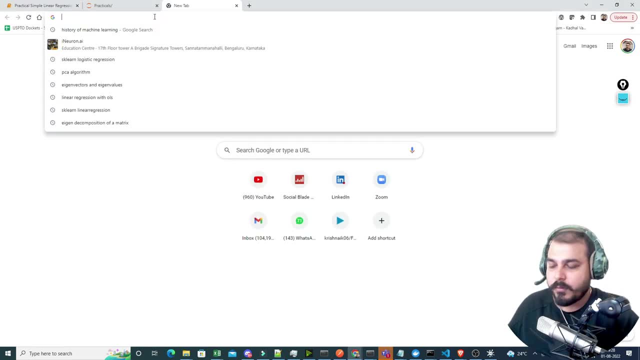 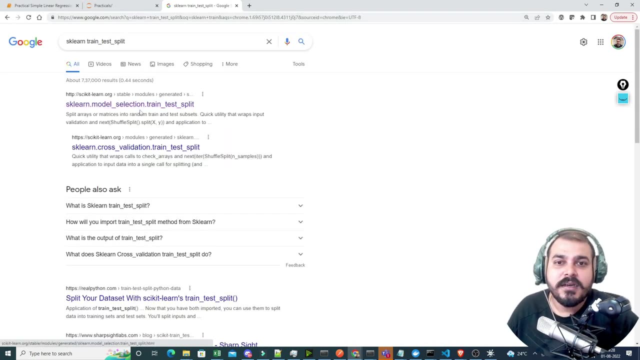 library that we are going to use, you will be able to get it in sklearn, okay. so, uh, if i probably show you one case, right, let's say i have used train test split. so if you go and probably search for sklearn train test split here, you will be able to see that this is the algorithm that is specifically used. 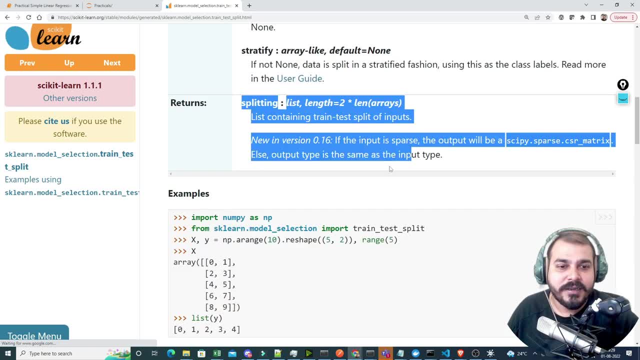 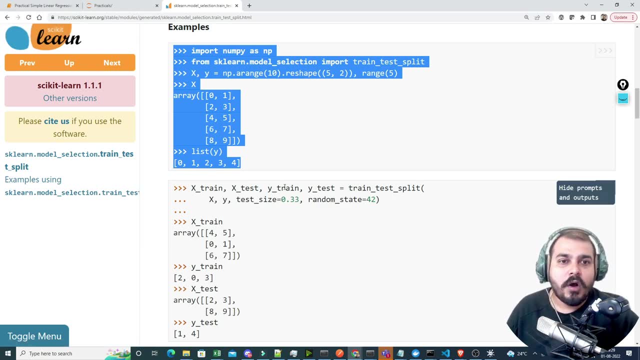 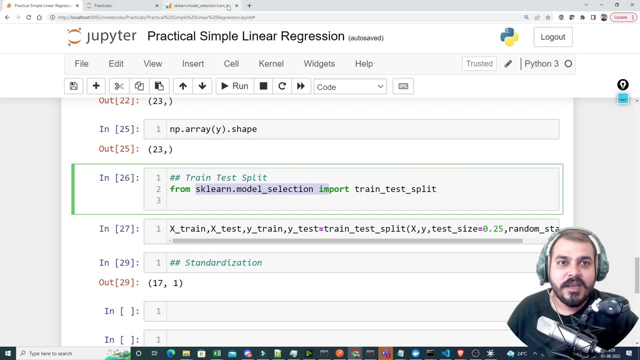 so here you can see all the parameters, what parameter, what it returns, and you can also see some of the examples, right? so all the time, suppose, if you don't understand where this library exists, all you can do is that search the google for that specific library. so that is the reason i am able to write from sklearnmodel selection import train test split. 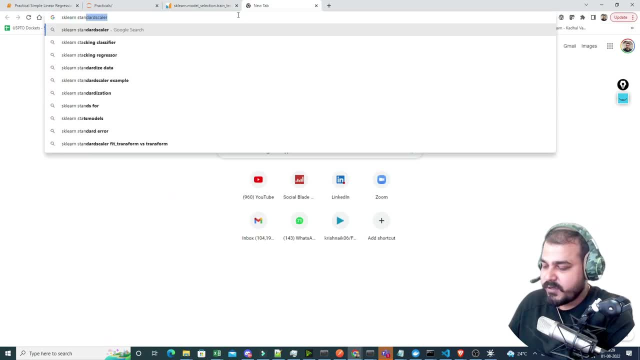 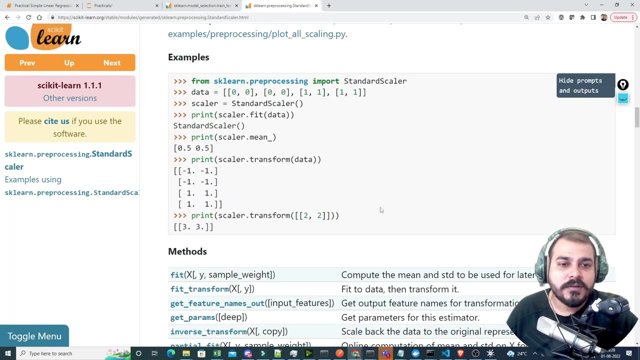 similarly, here you will be able to see sklearn. standardization is there, which we call it as standard scalar. okay, now, if i probably search this and if i probably see this here, you will be able to see that, uh, you are getting all the values over here, right, so perfect. 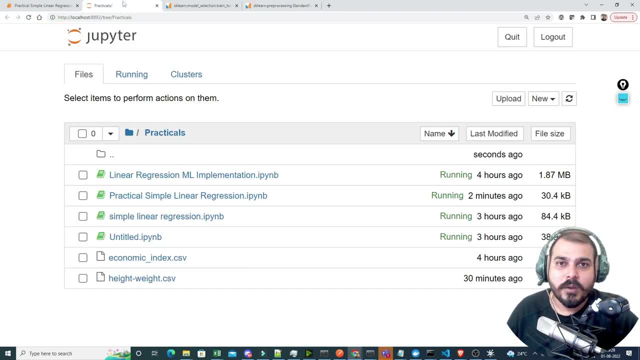 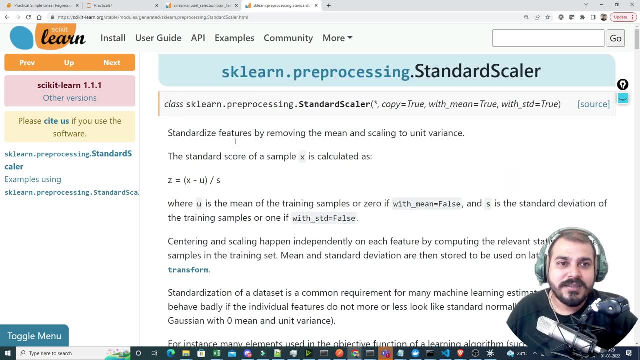 we are very much in sync and we are able to understand. okay, now the next thing that we are going to do over here is perform standardization. so, from standardization, what is the, what is the library from sklearnpreprocessing? okay, so here i'm basically going to write from: 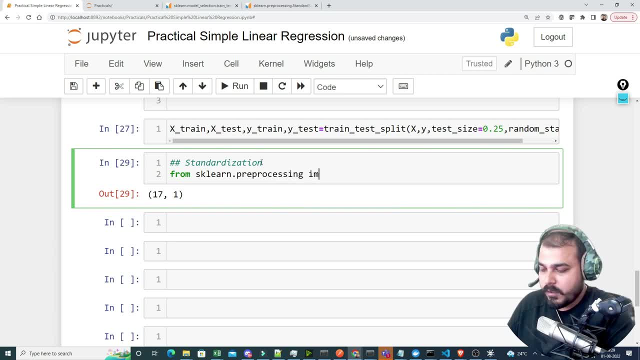 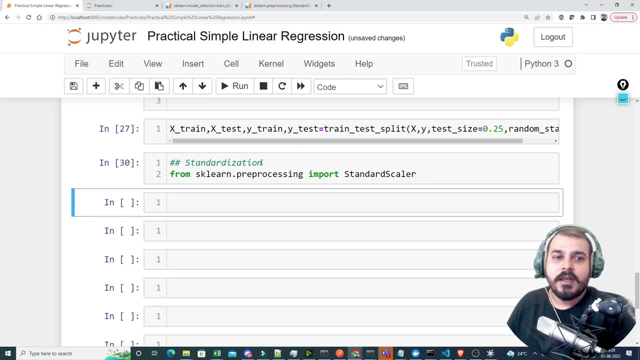 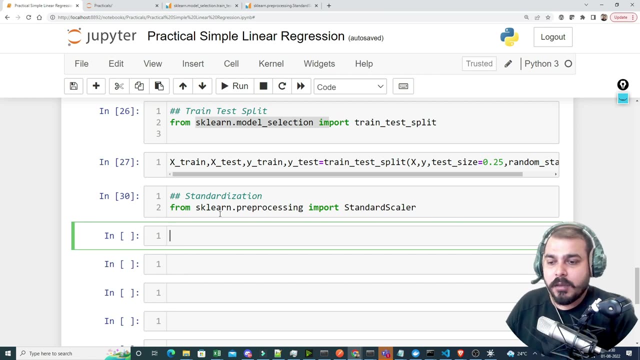 sklearnpreprocessing: okay. import standard scalar: okay. so once we do this, let me just execute it. and here now we are going to standardize my input feature, not the output feature. we do not have to standardize the output feature because our gradient descent gets applied into the independent features, right? 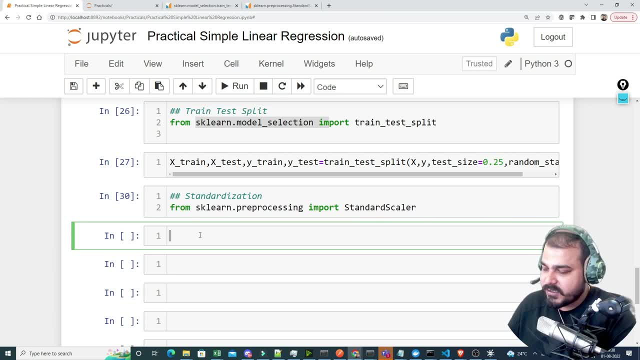 so, uh, what i'm going to do over here is that i'll just say i'll initialize standardized. so let's say i'm using standard scalar, so this will initialize with that formula, and okay. so here's the first step, right, and i've written: z is equal to x of i. 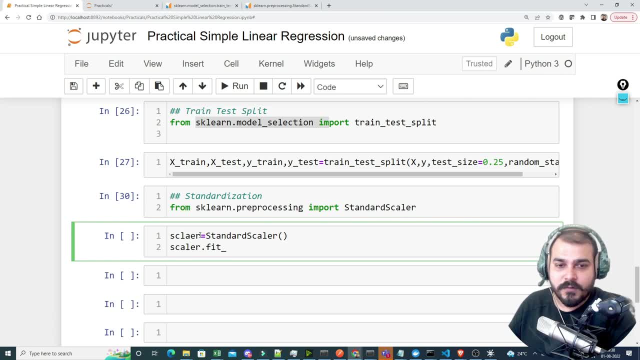 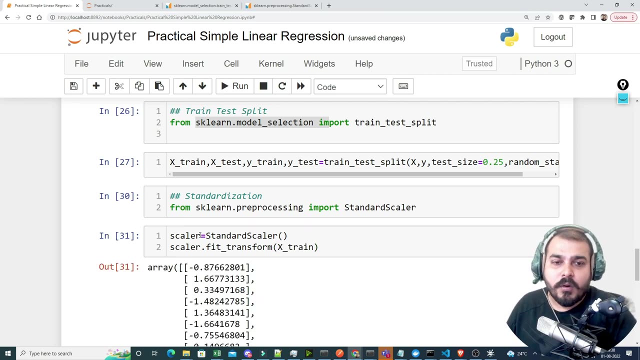 minus mu divided by standard deviation. okay, then, after this it is just going to write: scalar dot fit underscore transform. so let me give this formula again: scalar dot fit underscore tar transform. and here i'm just going to give my extreme. okay, now what will happen for all my 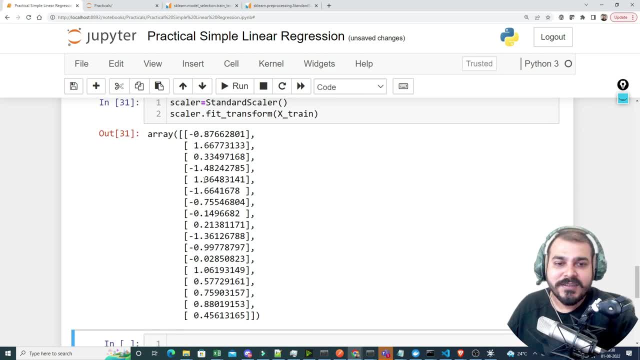 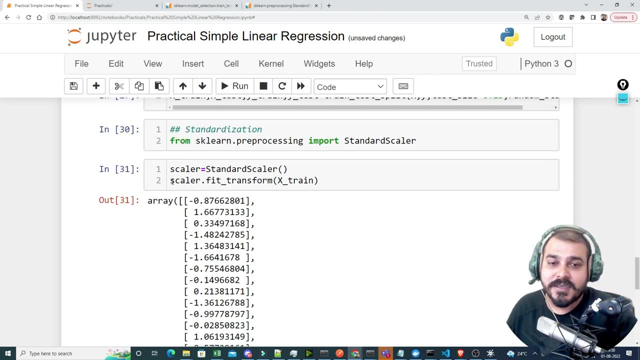 extreme. this transformation will get applied now. here you can see all the data that i use here. all the data points over here mean will be 0 and standard deviation will equal to 1 then that basically means all your data points will be transformed in this scale and this i will assign. 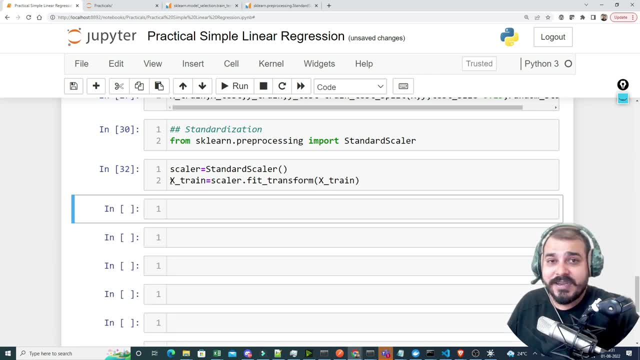 it to x train. now the same thing i need to do for test data also. right, but always remember, in test data we do not apply fit underscore transform. see, the difference between fit underscore transform and transform is that initially, whatever data that i have, let's say whatever data i have in train, 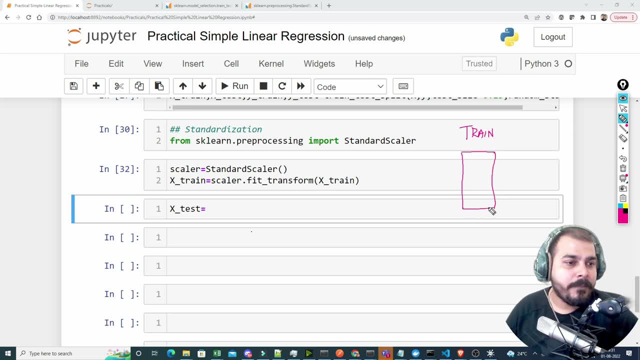 i'm going to use the same mean. let's say the formula is like this: x of i minus mu divided by standard deviation. i'm going to use this main mean and standard deviation only of this training data set and i'll apply the same formula in the test data set, right in the test data set. so for: 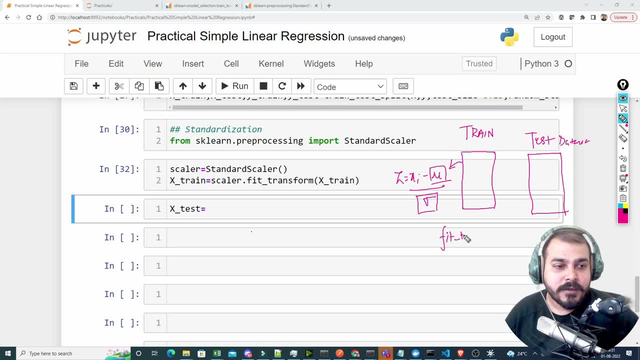 this particular case, what i do: in training i say fit, underscore, transform, and in the test i just say transform. when i say transform, that basically means i'm going to use the same formula in the training data set- mean and standard deviation- and use it over here, okay, and apply the same formula. 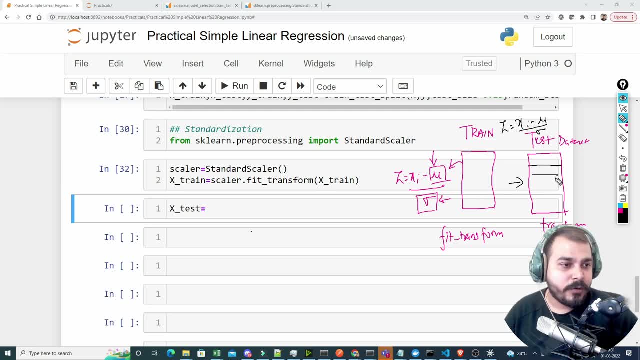 like x of i minus mu divided by standard deviation for all these data points. i'll be using this mean and standard deviation only if i use transform. if i use fit transform, then again mean or standard deviation will get calculated for this data. i don't want that. and why do we do this? because 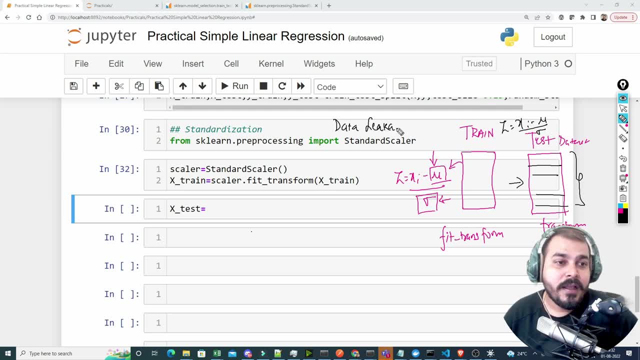 there is a important concept which is called as data leakage. i don't want my training data to know any info about test data. okay, i don't want that thing to happen. you know my, my model that is created. this should be the truth value. okay, this should be the information that should only be known right and when my model sees. 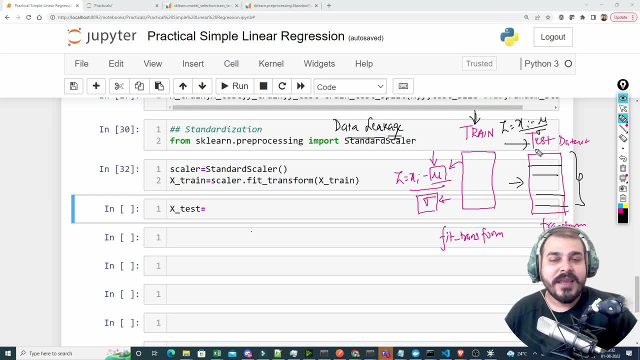 this. it should always see this as a new data, so that then only we'll be able to understand whether our model is performing well or not. okay, super important data leakage: fit, underscore, transform and transform. so this is a very important interview question. okay, why do we use fit? 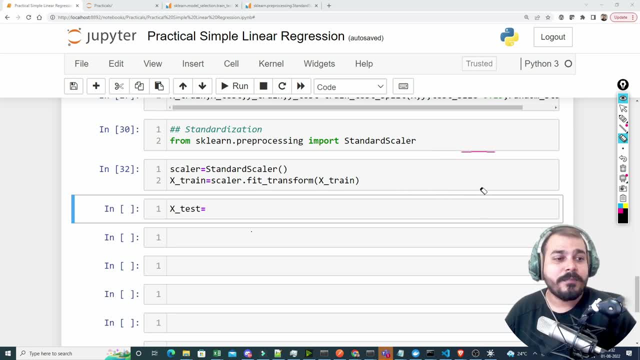 underscore transform, and this we will also be doing in pca. that is principal component analysis. okay, now let's go ahead and let's continue. so here what i'm actually going to do here for the test data, i'm writing: scalar dot transform- okay. scalar dot transform- okay. 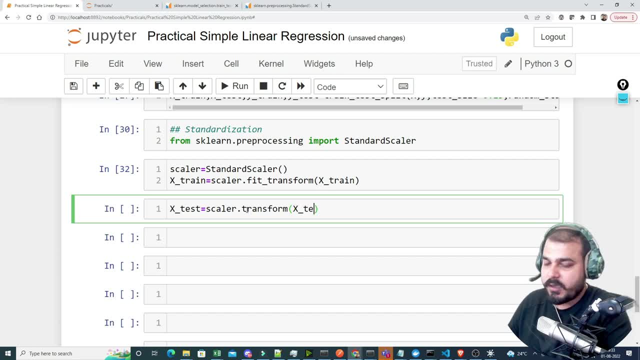 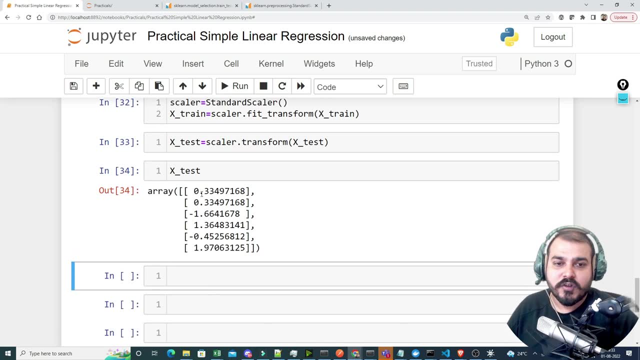 and then i will basically write this on my x test data: let's see whether we'll get any error. so here again, this is perfectly done. now, if you probably go and see your x test, you are going to get this. so this is my test data and this is how it has got transformed. this is perfect. 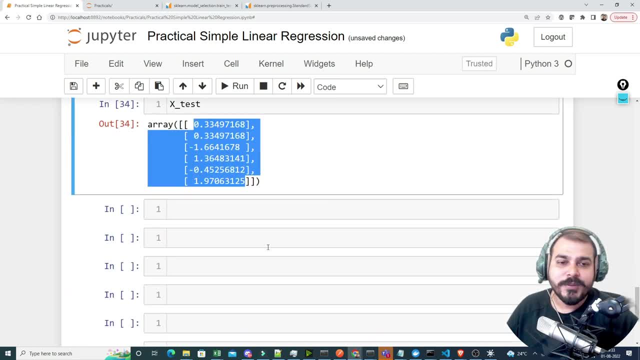 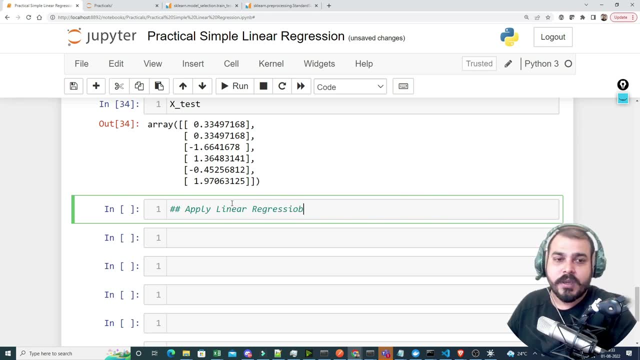 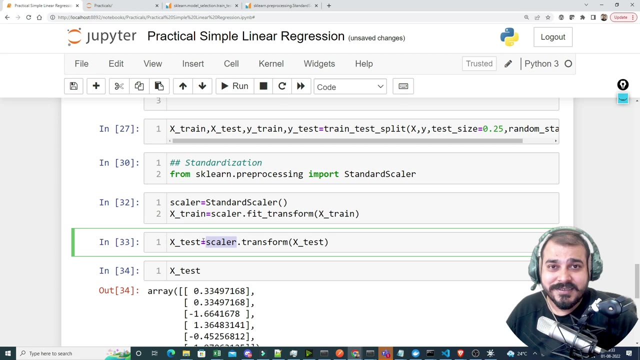 till here. now, the next step that we are probably going to do is that: apply machine learning algorithm, that is, linear regression. apply linear regression. okay, and this is super important, I will again be using this. this particular scalar value, okay, this, true, this will be again used for the new data also. any, 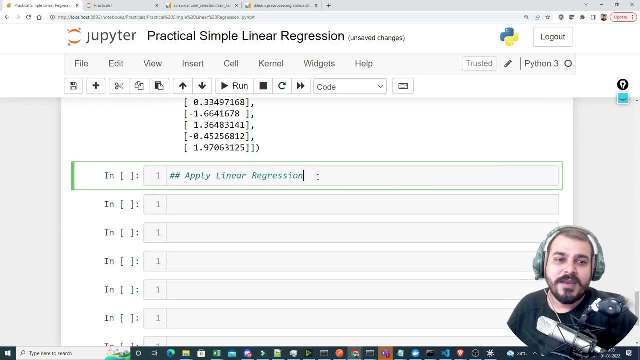 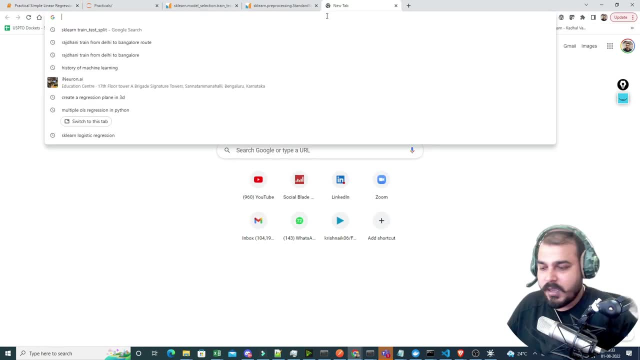 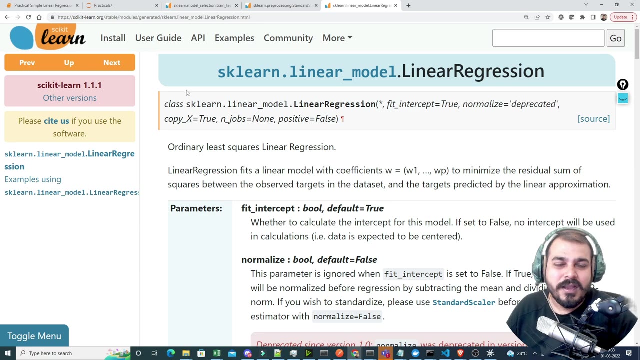 specific new data that has come will again transform them. okay, now I will apply simple linear regression. now, in order to apply, will again learn and in this scalar I will search for simple linear regression. so here you will be able to see something called as linear regression. so this is the model that we 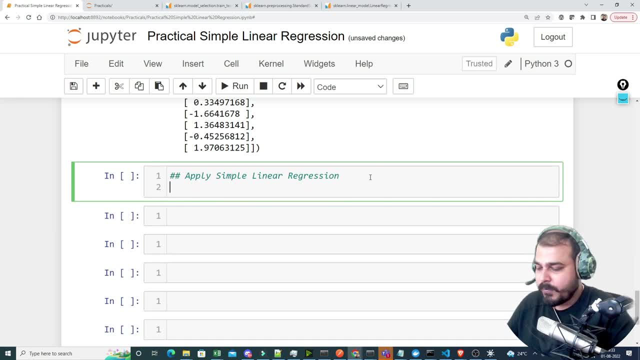 are going to apply. so let's go ahead and let's write form a scalar dot, linear model, import, linear regression. okay, now here you will be able to see. the first thing that we are going to do is that we are going to apply simple linear regression. that I will do again: initialize the object whenever we are using any any. 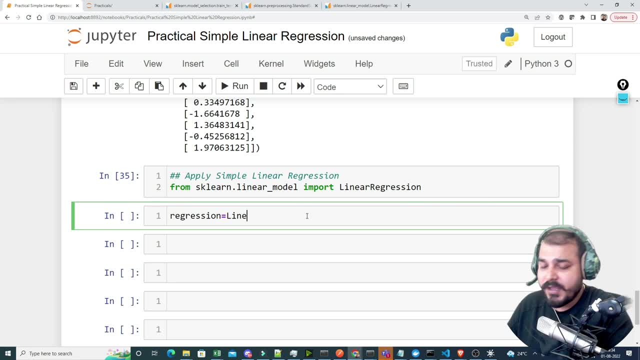 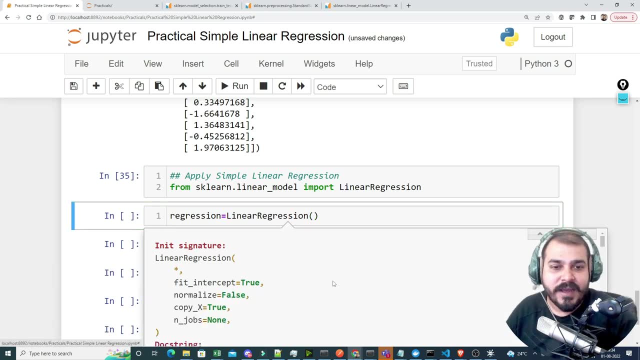 libraries from a scalar. first of all, we need to initialize that object. okay, so here I'm going to initialize linear regression by default. the parameters, what all things are there? so there is a first parameter which is called as fit underscore intercept. now, this fit underscore intercept is nothing but it. 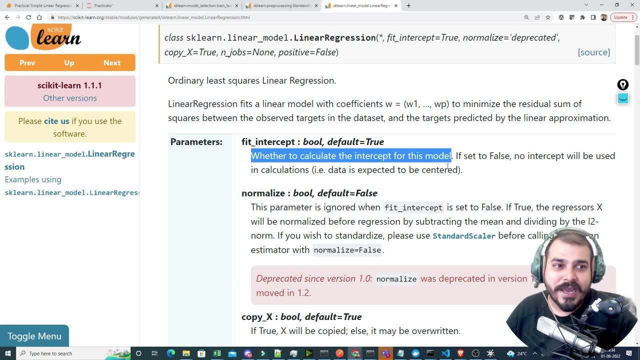 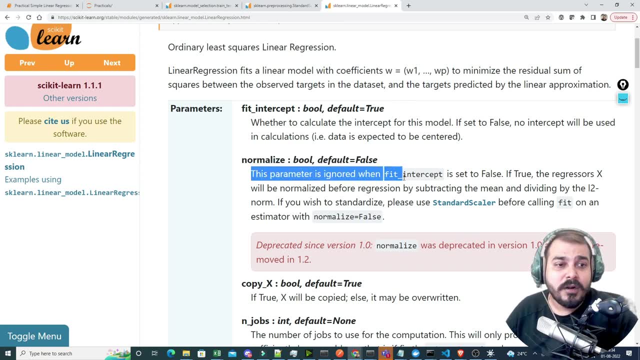 will say that, whether to calculate the intercept for this model or not, obviously I want to calculate this, so by default, whatever true it is, I'm going to keep it as true. now, this normalized function is there. this parameter is ignored when fit underscore intercept. intercept is set to false. if true, the regressor s will be normalized and this process we have. 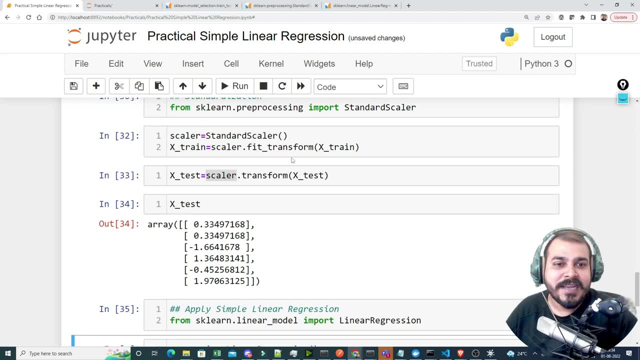 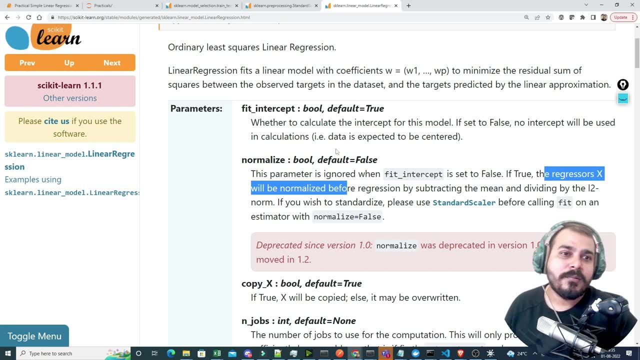 already done this right. we have normalized here. we are standardized this by using standard scalar. we have already done that. so whatever will be the default value will keep. if you are not that, done that step. normally you could have kept this as true. okay, then you have n underscore jobs. this n. 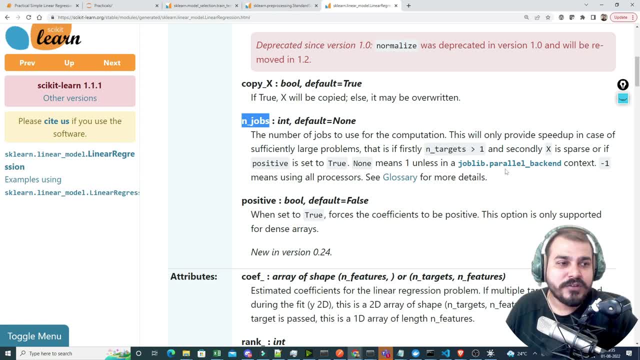 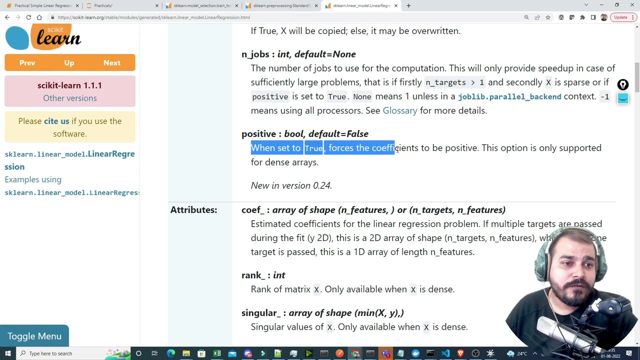 underscore jobs is a very important parameter because if you set this as minus one, it is going to use all the processors that are there in your system with with the help of them, it will try to converge and it will try to do the training okay and positive. basically says that when set to true forces, the 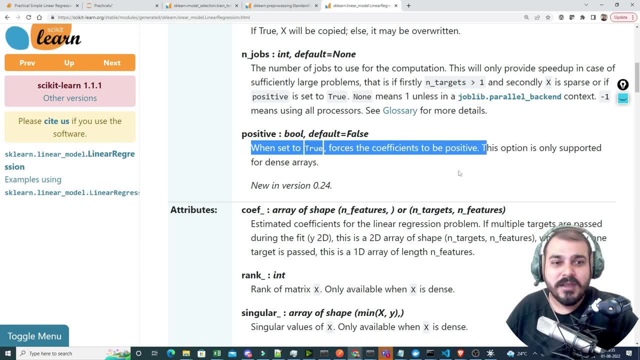 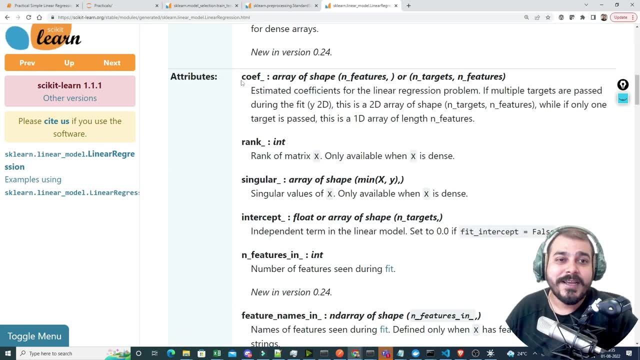 coefficient to be positive. so I don't want this specific thing to happen, because some of my coefficients can be negative. then in return, what all things you'll be getting if you apply this algorithm here? you'll be getting coefficients, rank, rank of matrix, singular, singular value of X and 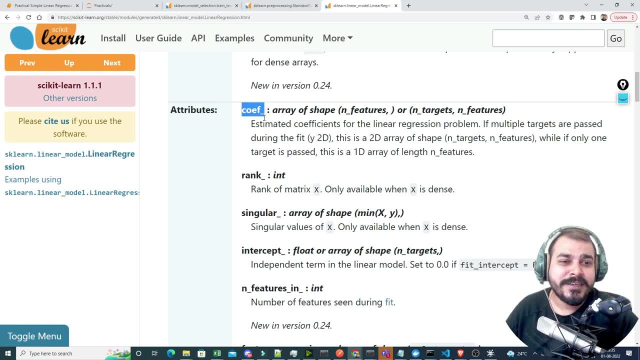 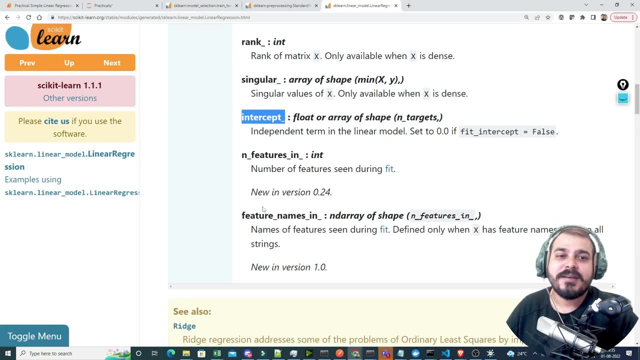 intercept. but out of all these things right, the most important thing is coefficient and intercept, and we'll try to see that: how many, how many, what is the coefficient intercept and what is the relationship with respect to the final output? we'll see that there is also a feature that will get returned, that is: 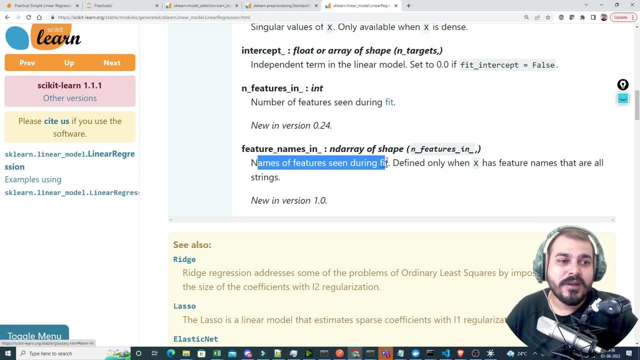 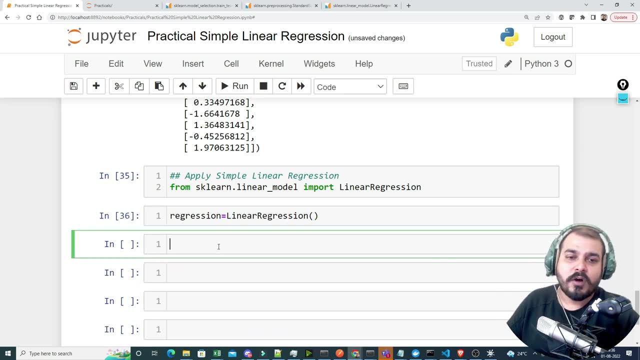 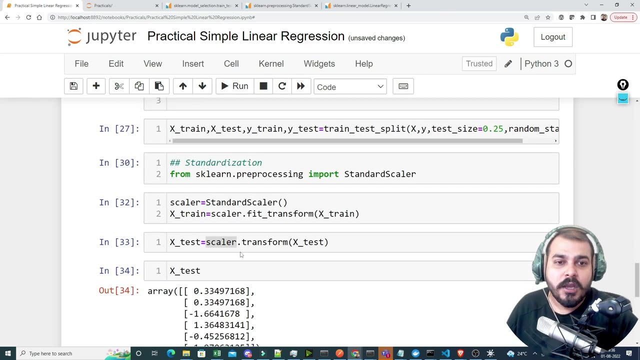 called as feature underscore names. underscore in name of feature seen during fit. that also it will show. we'll try to see this, okay. so here I have applied linear regression. let me just go and execute with all the default parameters and I'll say a regression dot fit. now I want to fit this regression model to our training data right. so all. 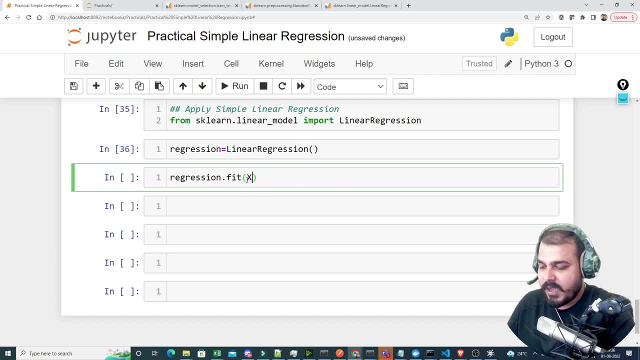 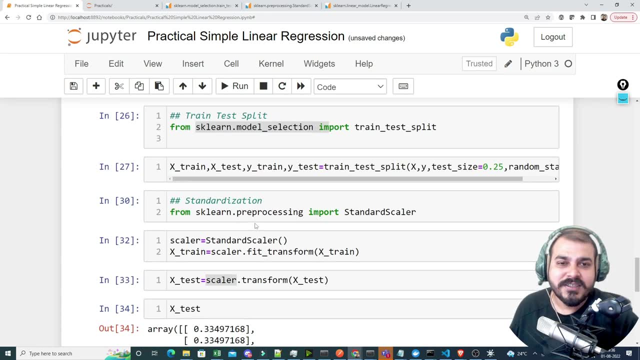 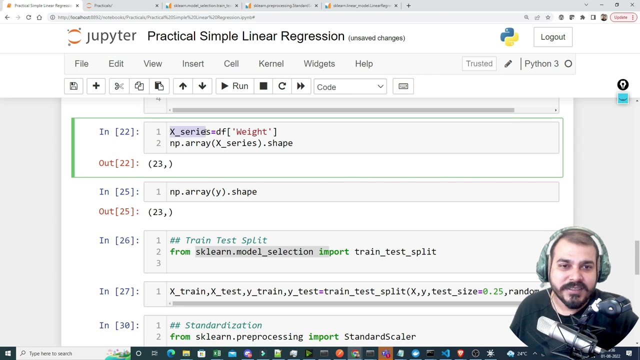 we will do is that we will go ahead and assign this and we'll assign it to X underscore train. now, understand, guys? let's say with, before giving this X underscore train, let's say I created one more variable, right, and that specific variable was called as X underscore series, right, and you know that this is. 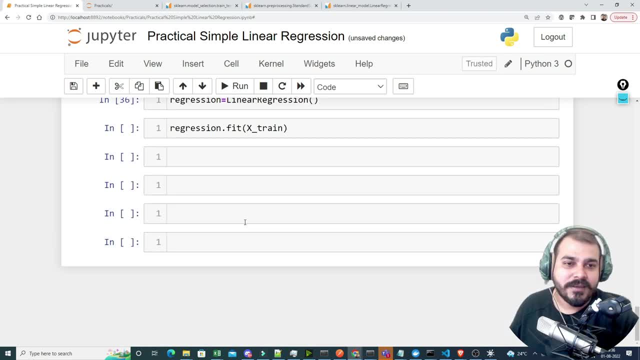 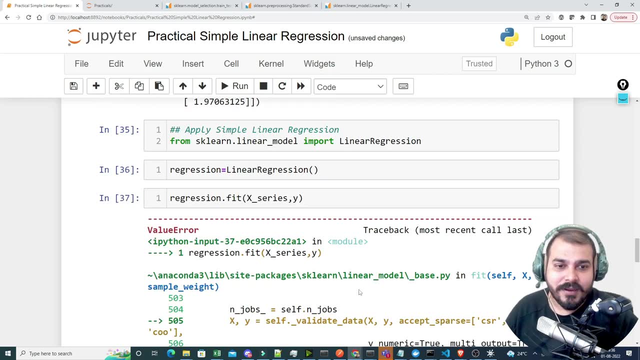 one dimension now instead of X underscore train. if I give this, what will happen? see, let's say, if I'm giving this and I'm giving Y because this had all the data, now see what will happen. it will give us an error. why? because it is saying that: 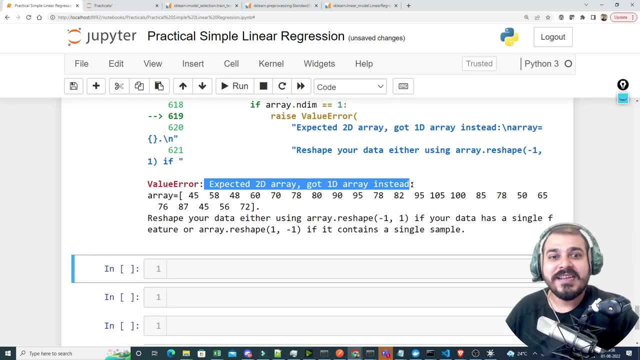 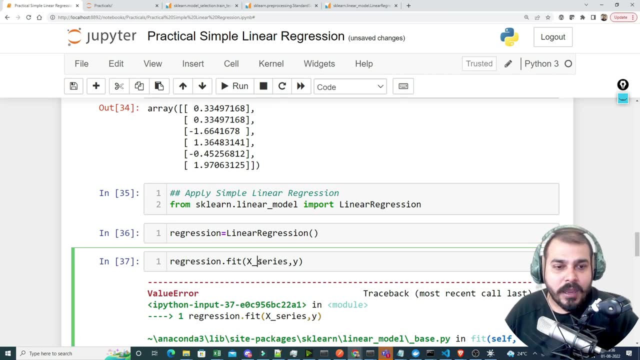 excepted 2d array right. got 1d array instead, right, and this was a 1d array, right. so always remember any algorithm that you'll be seeing in the fit and whatever training data I am giving, it should always have a 2d array in the. 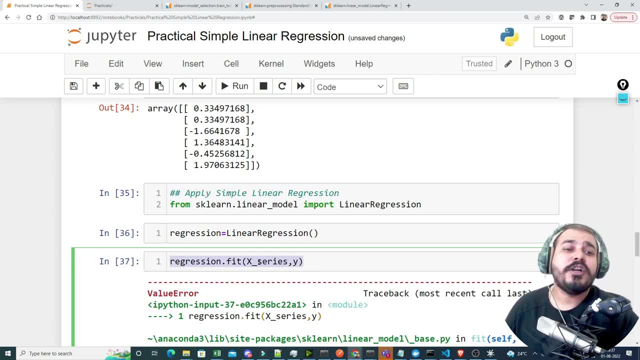 output. if you have 1d array, that is fine, not a problem. but here you need to give it as a 2d array, okay. so here what I'm going to do is I'm going to give it a 2d array here, so I might give a source: j pass no, you'll give no, do a bar. 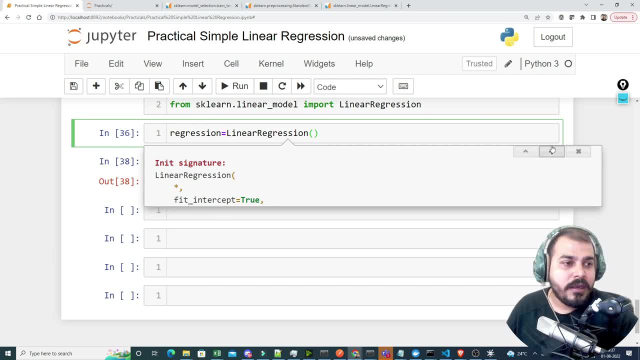 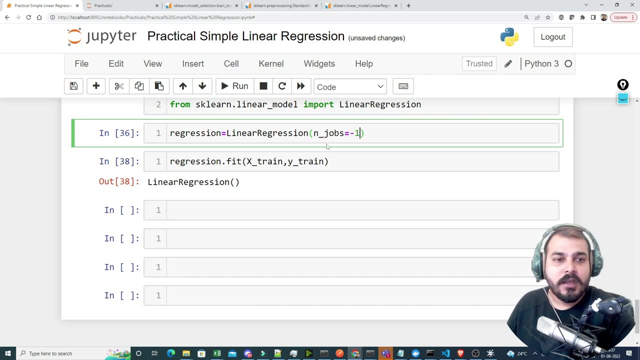 returned, NOT a vote. and here let's copy 2d array, and I'm going to test this, So I don't even have the scene baby. so we should give non extra comma Y train Now. we will go and do the fit Now. once we go and do the fit now. 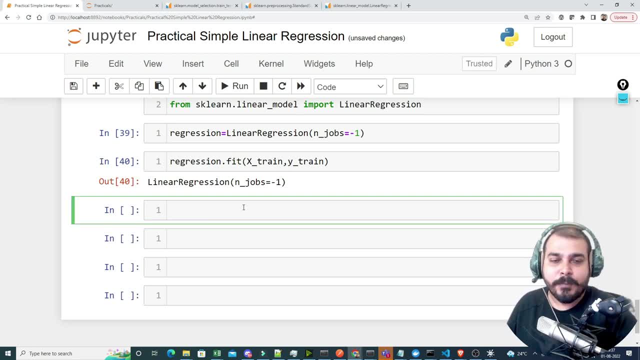 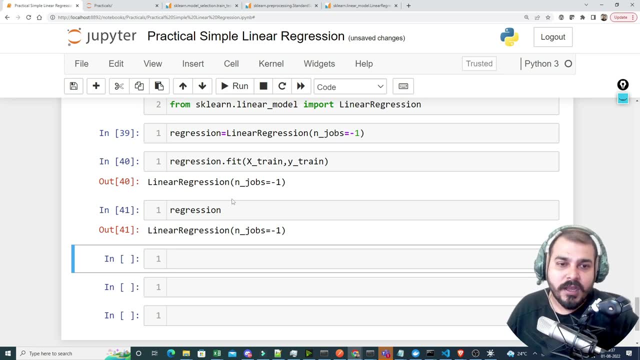 Let's see over here to minus one. yes, you cannot see that because it is happening within the system right now. if i probably go and see my regression now, it is basically showing linear regression. now, all i have to do is that in order to predict, or in order to predict my test data. how do i do it? so there, 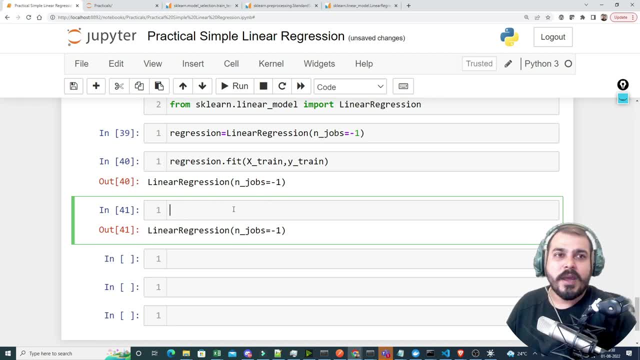 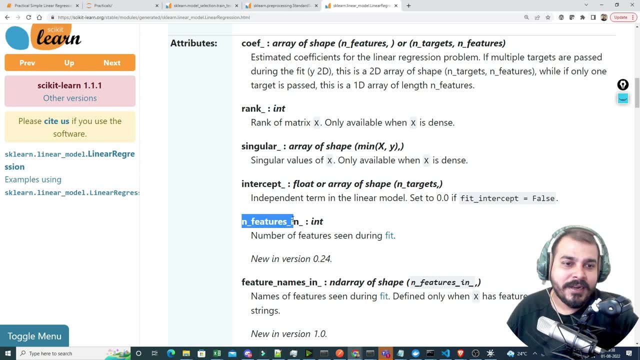 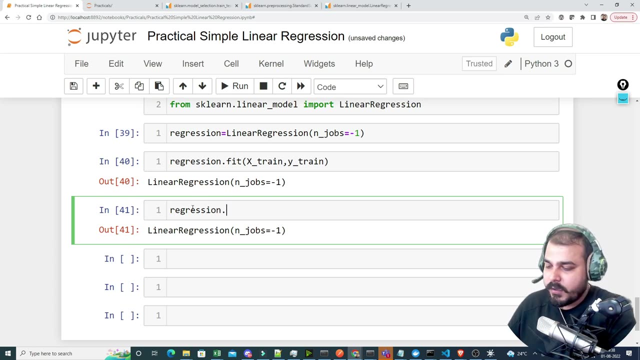 will be a function which is called as predict, but before this i already told you that how many different types of parameter it is running coefficient. coefficient basically means slope, intercept and underscore features. rank and singular will not focus much into it, so let's go ahead and write the night regression dot here. i will say coefficient. now, if i go and execute this, 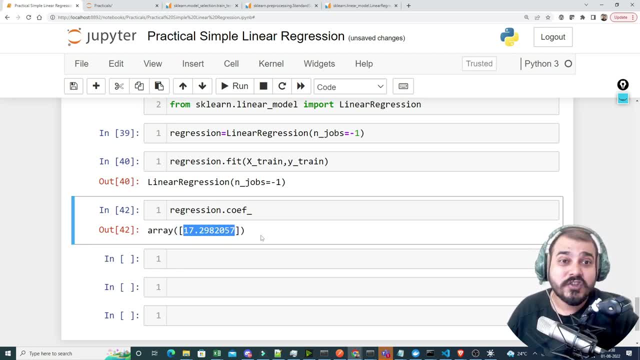 here i'm going to get the coefficient. now this coefficient is the slope. and why only one? because i just have one independent feature. now, if you remember the entire equation, if i have one independent feature, so my equation will become: y is equal to or y hat is equal to, beta zero plus. 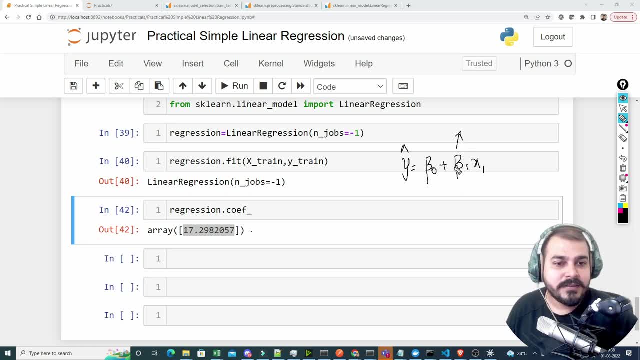 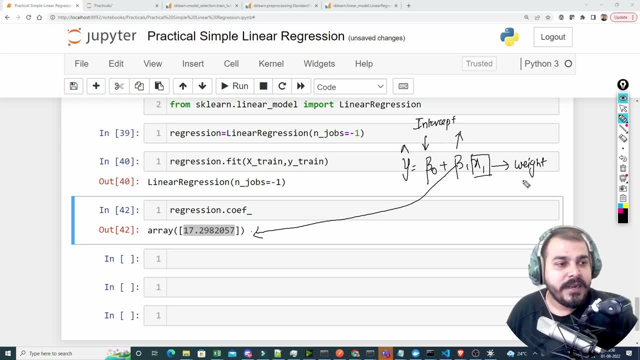 points. in this particular case, these data points are nothing but weight, right. so this data points are weight. this we have calculated beta one intercept we will be able to get when we are writing regression dot intercept underscore. okay, so here let me remove this quickly and let me 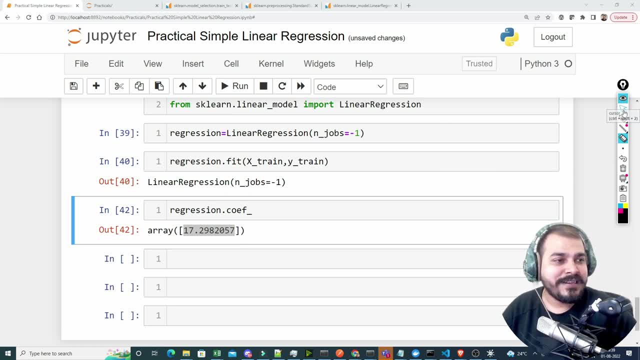 show you, to you, the reason why i'm using this, so that i write anything in front of you so you'll be able to understand. okay, so here now, this is my coefficient, so let me print my coefficient. so here i'm just going to say coefficients, or slope is nothing, but is this specific value, comma, regression coefficient? okay, 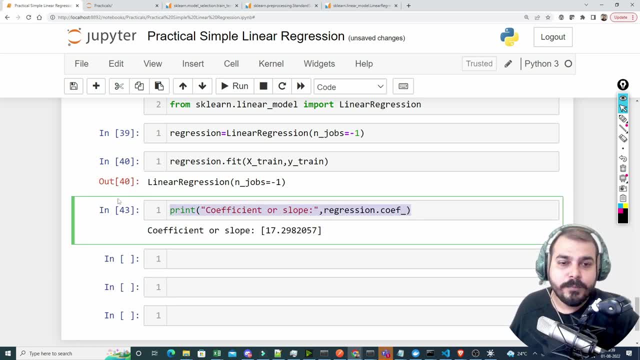 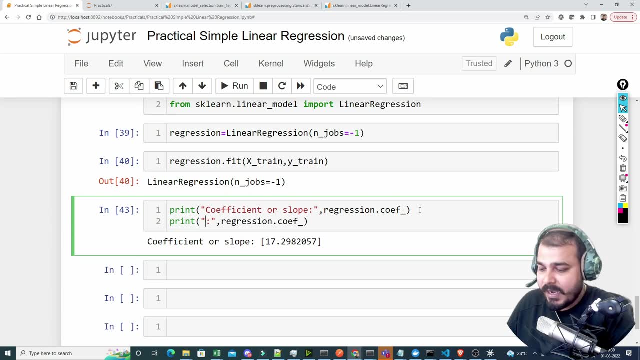 so here i have just printed it. okay, similarly, i can also print intercept, so i'm just going to copy this and write print over here intercept and i'll talk about this. what is the meaning of this? also, intercept is equal to, so this will nothing be. i will just write intercept underscore. so this is my intercept and this is my. 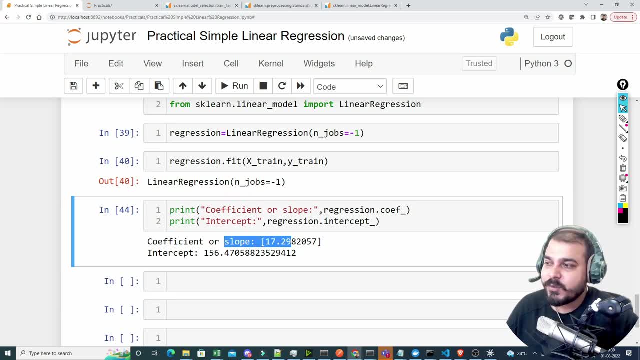 slope. now, what does this basically? uh, with respect to this, okay, now, super, super important. that basically means one unit movement in the weight value, let's say one unit movement in the weight value that leads to seventeen point two, nine unit movements in the higher value of the weight value. 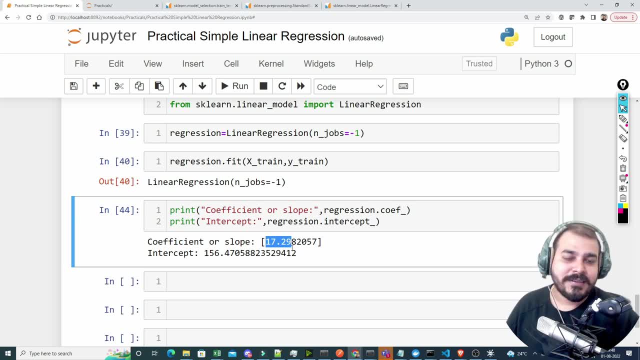 value. that is what it basically says. this coefficient again understand, guys? one unit movement. okay, let me just draw it again in front of you. suppose this is my x and y, this is my weight and this is my height. right, this is my height. it basically says that: one unit movement. 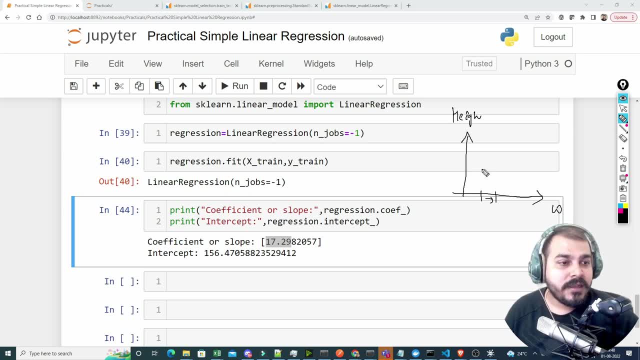 with respect to the y the axis, it leads to 17.29 unit movement. so, from here to here, basically this is 17.29 unit movement. okay, with respect to the y axis. so this is what this probably will look like- my slope. okay, so this is what we are doing and the next point is that: what is this? 156, 156 says. 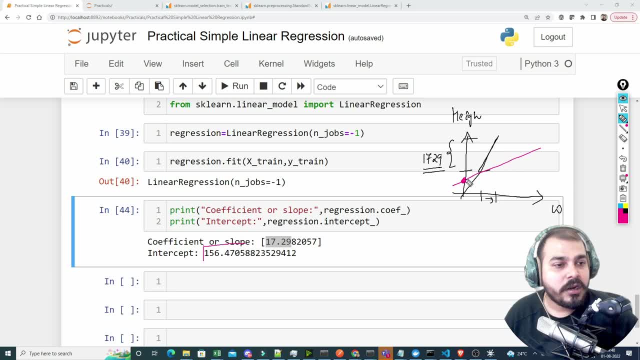 that when your weight value is zero, when, at what point your line is meeting in the y axis? so this particular point is nothing but 156.47. so i hope you have got an idea about it. okay, the importance of coefficient and slope, okay, and uh, let me do one thing apart from this. uh, now you have got your coefficient and intercept. 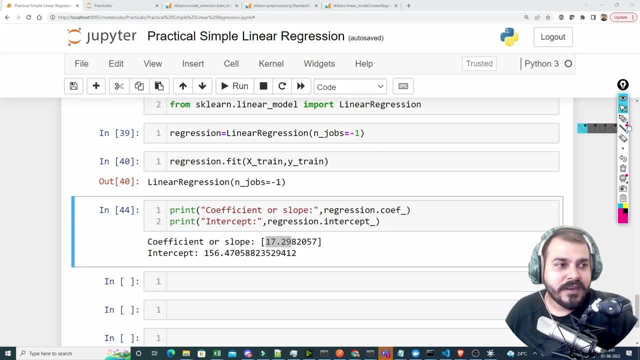 now you may be thinking: krish, okay, fine, we have created this. can we see some kind of line? so suppose, if these are my data points, can we see some kind of line which i can say it as a best fit? answer is yes, and i'll show you that. so let's go ahead and plot this particular points. 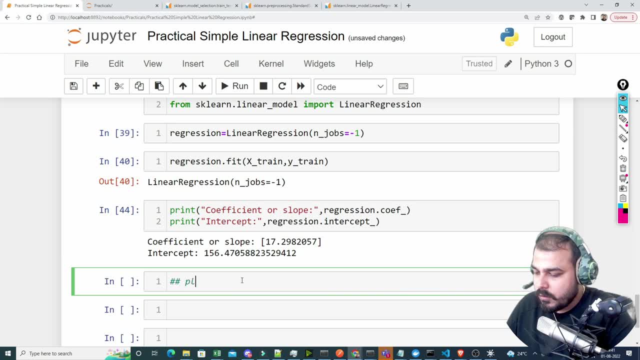 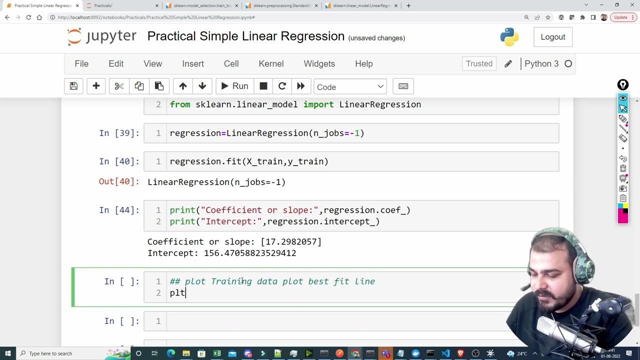 right. so here i'm going to plot the training with respect to training data. i'm going to plot, plot best fit line. okay, so here let's go ahead and plot it. so first of all i will say plt, dot, scatter. and here i'm going to scatter my x train and y train data. okay, so what will happen if i plot? 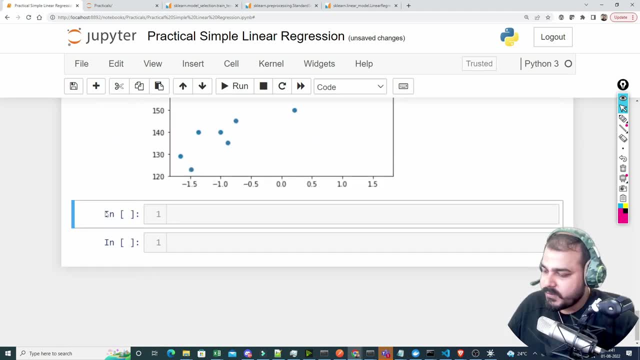 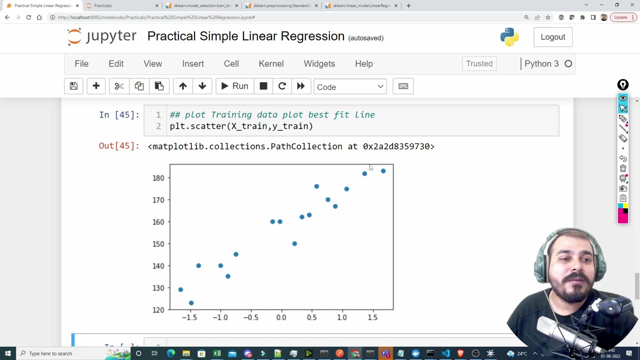 this. here you'll be able to see this kind of plot. okay, let me make some more fields, okay, so here you can definitely see some plotting happen right on the top of it. now you want to see how our best fit line is created? then what do i do? i will go and. 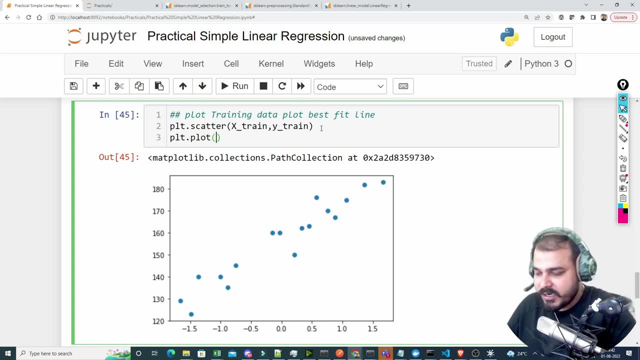 write plt, dot arrow, t plot. this plot is also used, and here i will be taking x drain, and we know that- how to find out our predicted value. right now, in order to find out the predicted value, all i will be doing is that i'll take this model. okay, this model is regression. 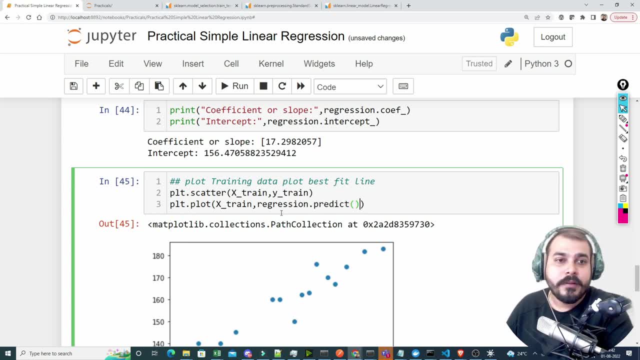 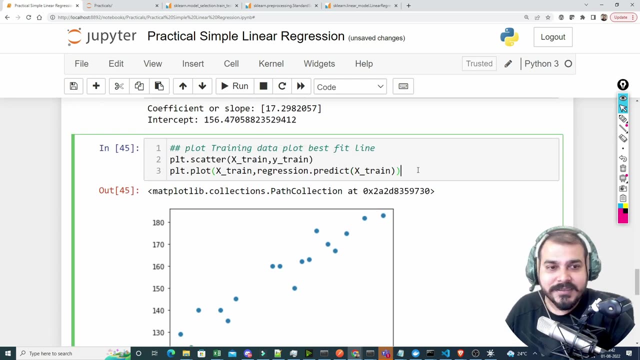 so here i'll write regression dot predict, okay, and here i'm specifically giving what value over here. see, If I write regressionpredict, here I'm going to predict for x train, So this will basically give my predicted value, along with the straight line. Now, if I go ahead and execute this now, see, this is the best fit line that has got created in the specific data set, right? 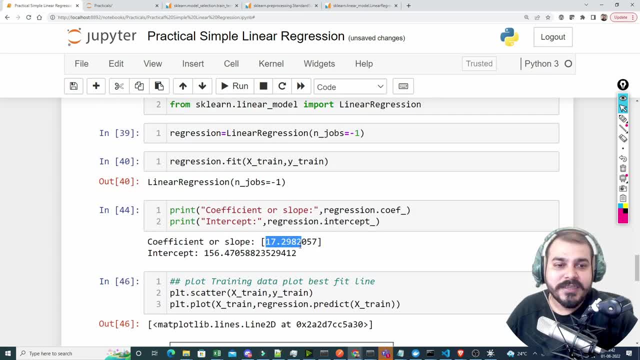 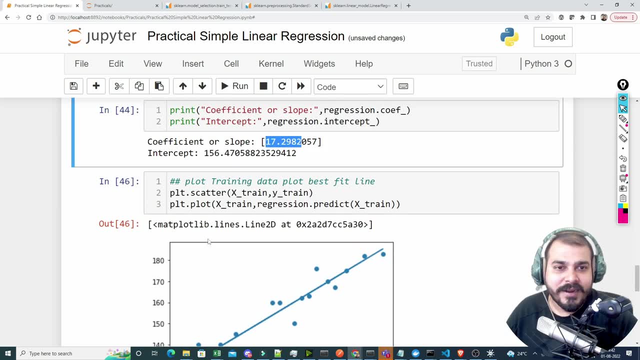 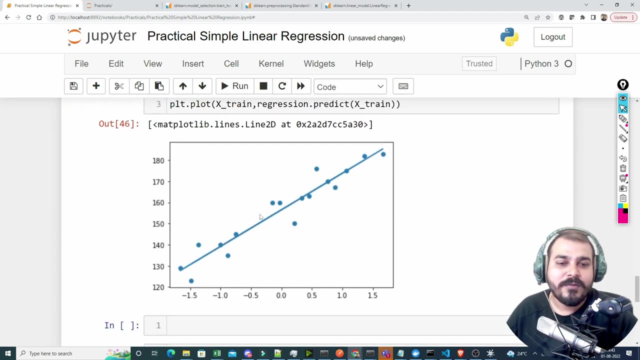 And this best fit line will have a coefficient of 17.29 and intercept of 156. Because see if I probably try to, you know, make sure that, or extend this when my value is 0, then we are actually going to get an intercept of 156, okay. 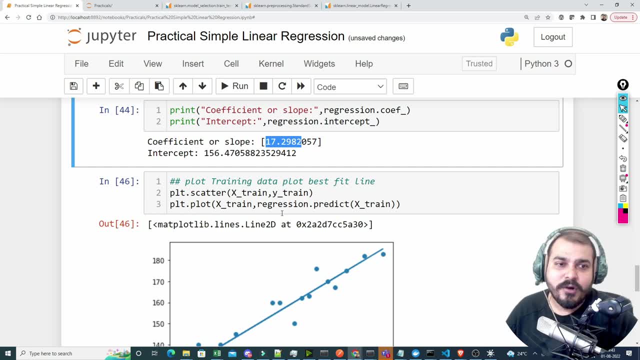 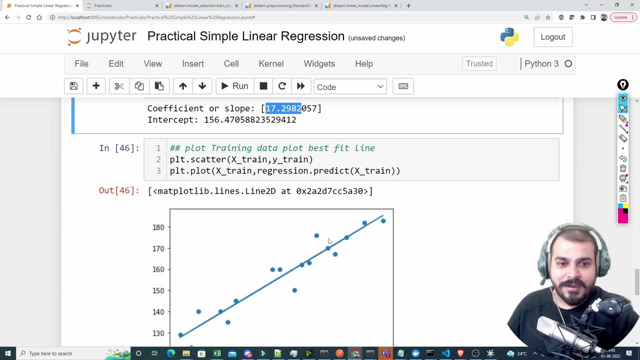 So this is what it basically says with respect to this. okay, So now here you can see I've got my best fit line. And with respect to this particular best fit line, we are able to see that. okay, the error also looks very less right. 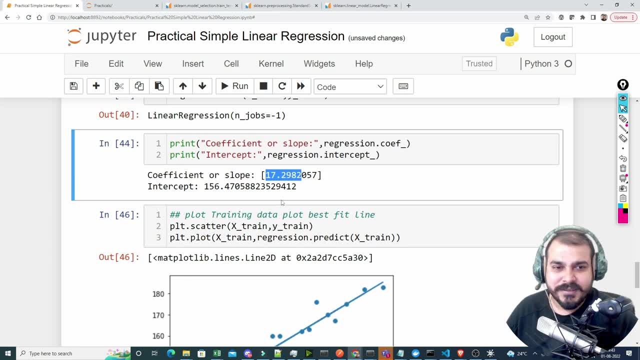 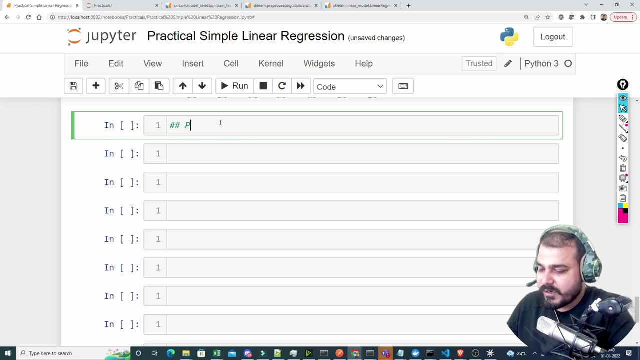 Here you can definitely see the error is also very, very less. Now let's go ahead And let's go to the next step. Now we need to do the prediction for the test data Now in order to do the prediction for the test data. prediction for test data. 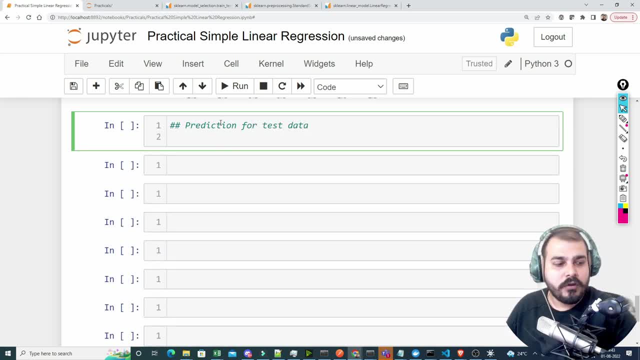 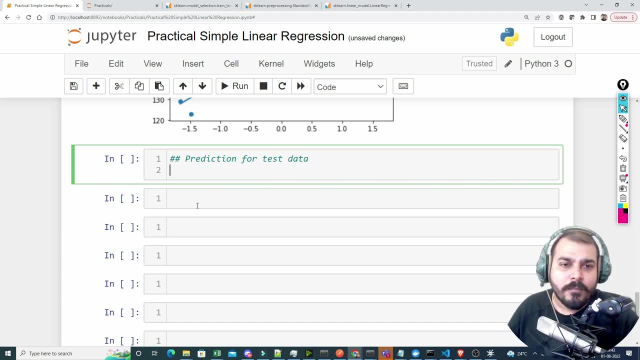 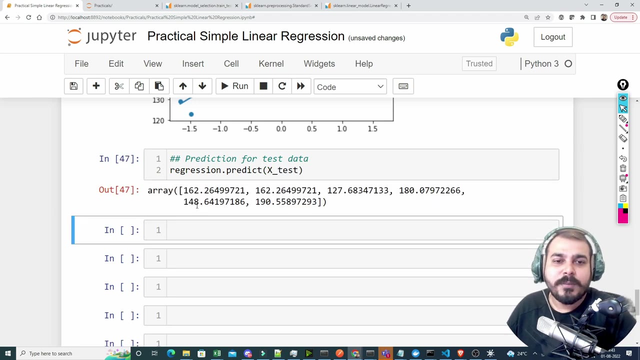 how do I do for the prediction for test data. So here you'll be able to see I will be using plotscatter or no need to use plotscatter also. So my model is something called as regressionpredict on my x test. Now here, when I do the prediction, this is my predicted value. 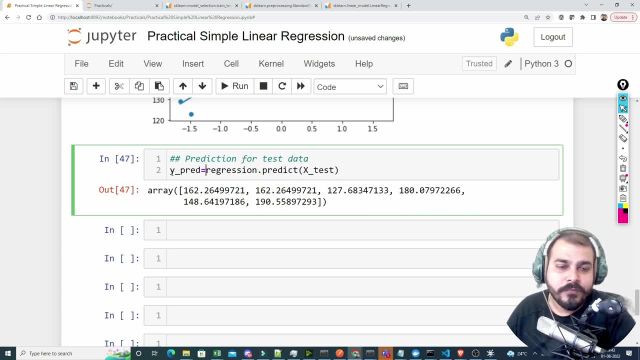 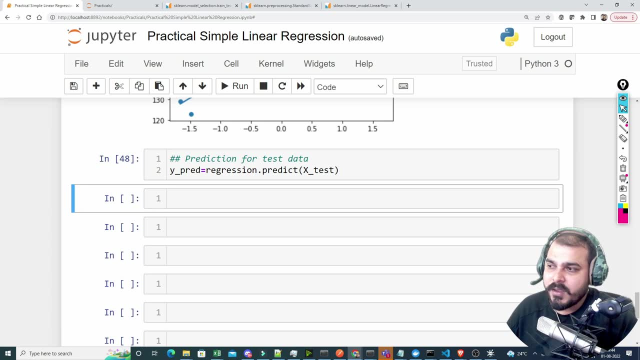 So this will basically become my y underscore print. okay, So let me just execute it Perfect Now in order to see how the result is. you know how the result is. we will try to now check with some of the performance metrics. 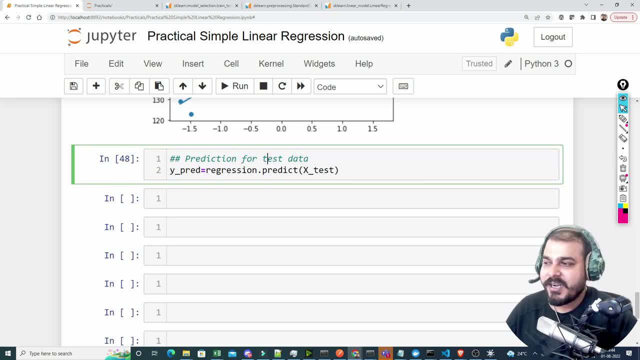 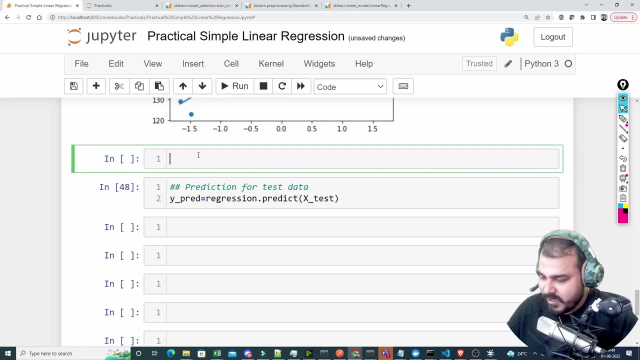 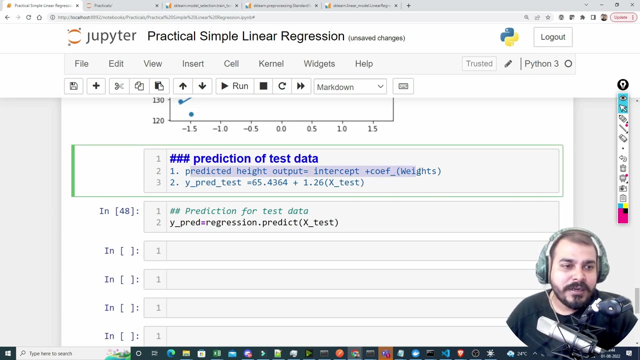 But before that, if whenever I do prediction for test data, right, I will just go and copy this thing. okay, Just let's see. I hope everybody will understand it. Let's say I'm keeping a markdown over here. Here you can see the predicted height. output will be intercept plus coefficient multiplied by weights, right? 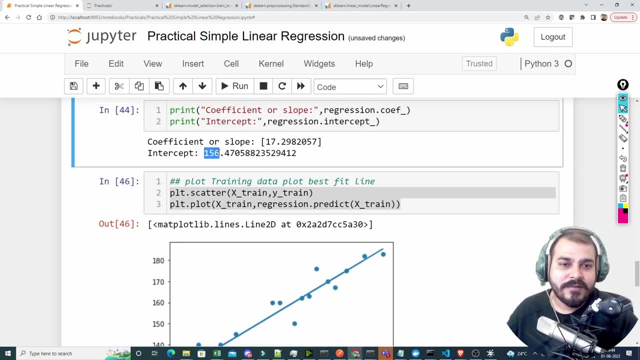 So right now, what is my intercept? My intercept is nothing but 156,. okay, Let's say, this is my value, okay, So I'm just going to copy it over here: And my coefficient is nothing but 17.29.. 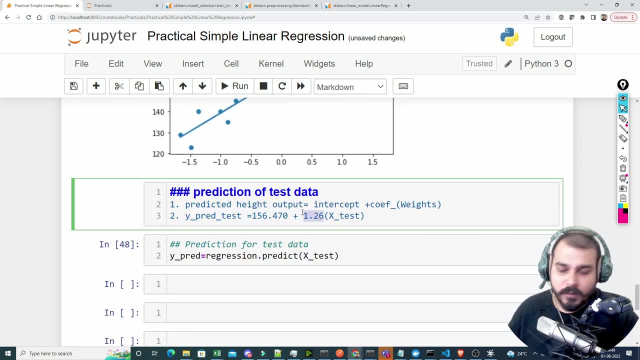 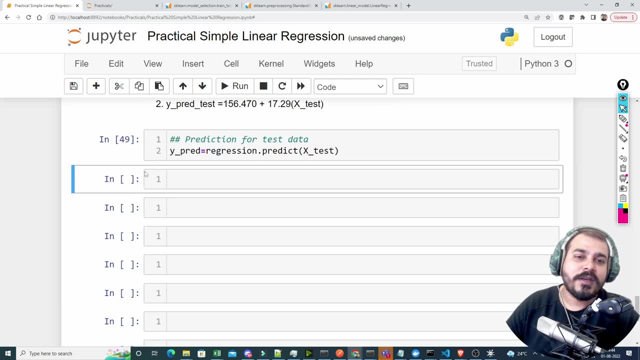 So I'm just going to copy this and paste it over here, okay, So this is what is basically happening in order to find out all my y print. okay, So here I'm just going, I'm just going to execute it so that it will give you an idea, okay. 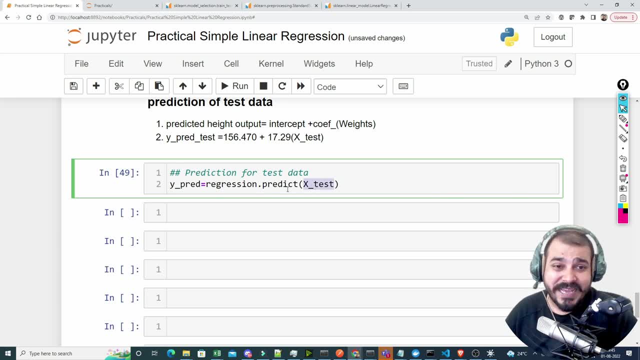 So I hope everybody is able to understand this Already. this understand. X-test data is already transformed also. okay, if you don't know Now, let's go ahead and do some more things in this. Fine, we have done the prediction. 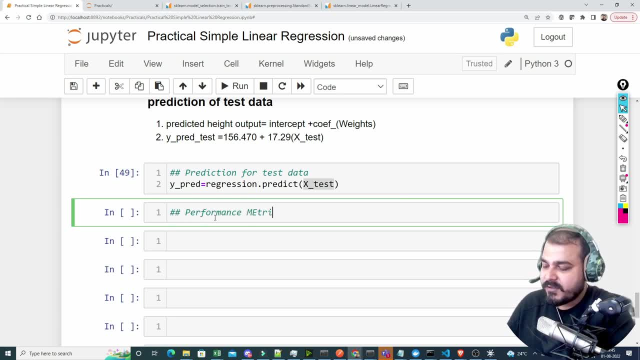 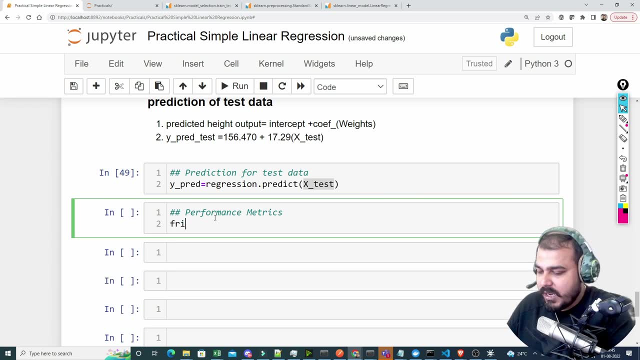 Now we'll focus more on the performance Now, which all performance metrics we have already discussed that we are going to see. So in this I'm just going to write the performance metrics that I have actually discussed. I'll write from sklearn: 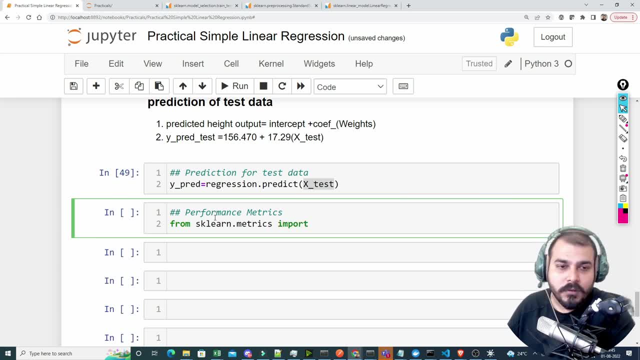 metrics I'm going to import. the library that I'm going to import is something called as mean squared error. So here you have: mean absolute error, mean mean squared error. okay, And there are also many, many other performance metrics which you can also use, right. 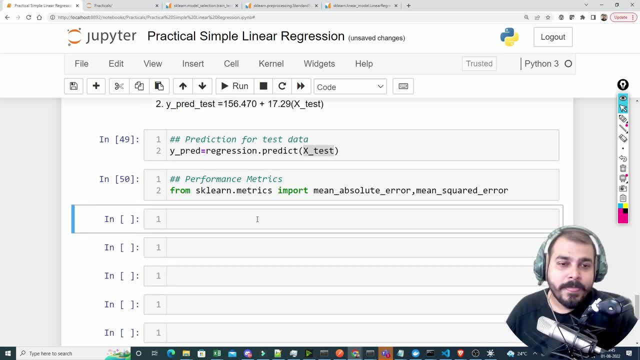 For right now I'll just use this because we have learned about this, okay, And then what I'll do? I will basically calculate my MSE mean squared error. So here I'm going to write Mean squared error And here I'm going to give my y underscore test comma. y underscore print. 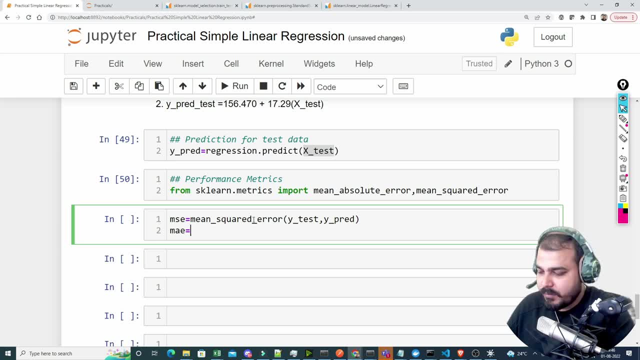 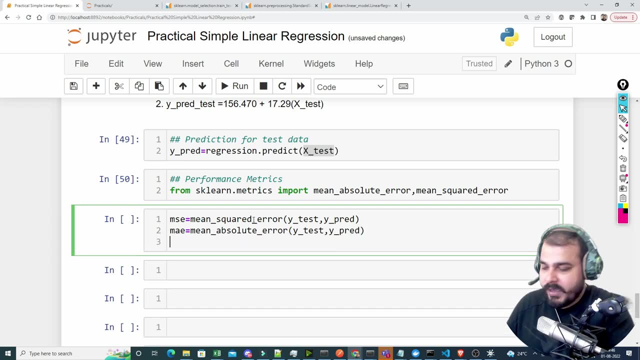 So this will basically give my MSE. Similarly, MAE is nothing but mean absolute error, And this will basically give my y underscore test comma, y underscore print And finally, root mean squared error, which is nothing but NP dot square root right of MSE. 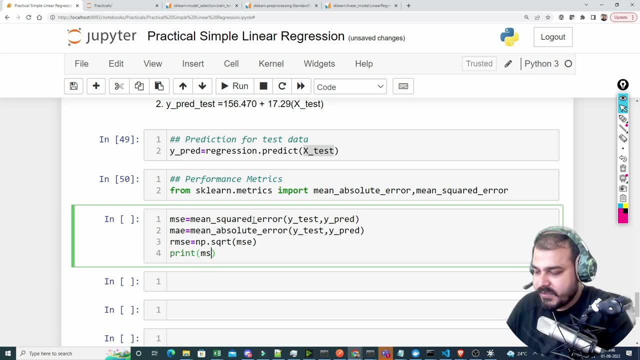 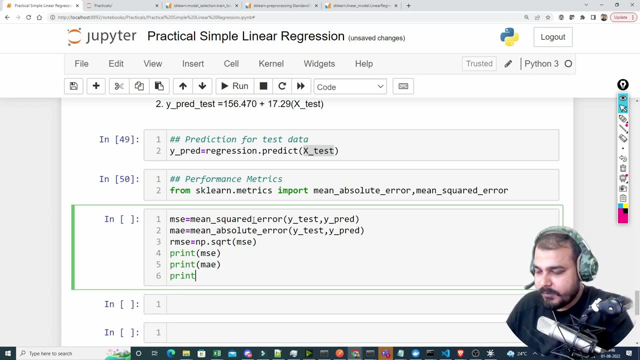 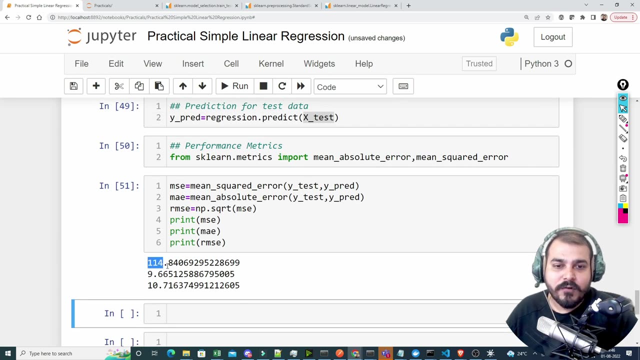 Then I'm just going to print MSE, Print MAE And then print RMSE, As I said that we really need to check all the parameters over here Now, here you can definitely see that 114.84 is your mean squared error. 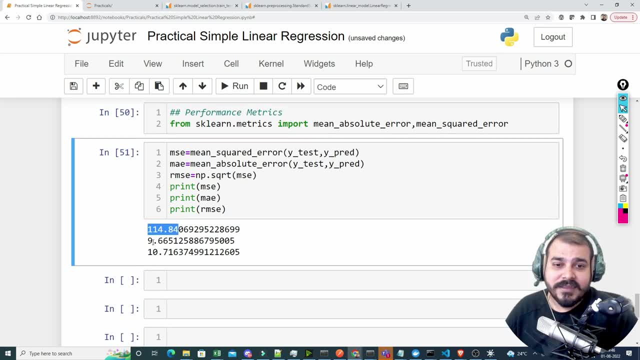 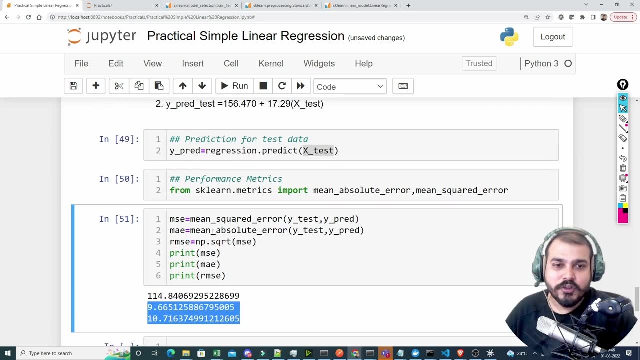 Definitely it has penalized a lot of outliers, you know, Whereas in this case- here you can see it's almost nearby- by using mean absolute error and all okay. So here this is what we have actually got with respect to our performance: error metrics. 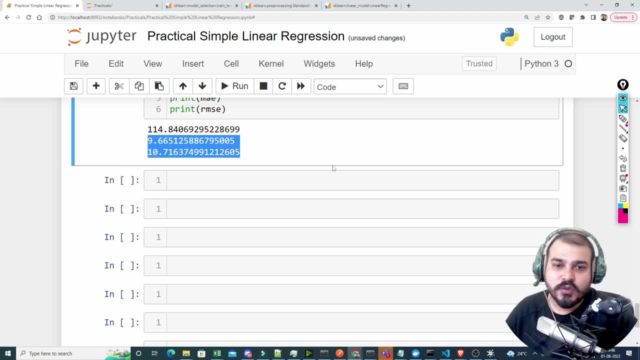 Now the next thing is that we are going to use is something called as R square also, So R square. if you remember the formula for R square, how we are going to use the R square, So here I'm just going to copy and paste the entire formula for you. 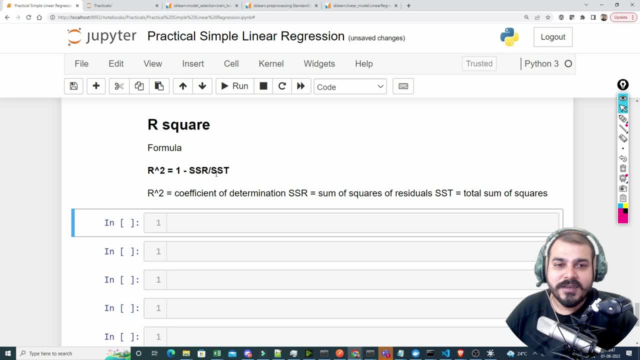 We have already discussed about this. There's nothing but 1 minus sum of square residual divided by sum of square total right? So here, this is the formula that we'll apply. In order to apply also. we can also use this from my library. 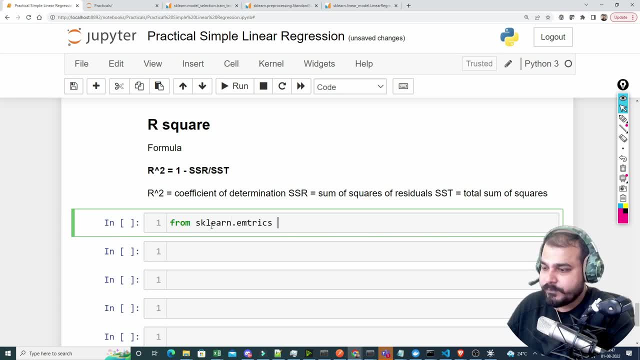 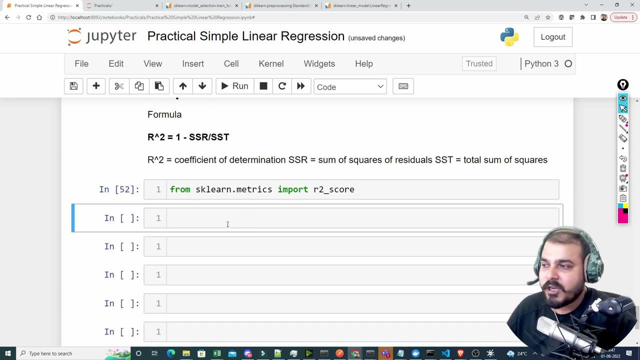 So I'll write from sklearn dot matrix: import: R2 score: R2 score right, So it should be matrix okay. So this also will look good because now overall we'll be able to get how our model is performing. So finally, my score will be equal to R2. underscore score is nothing but Y underscore test. 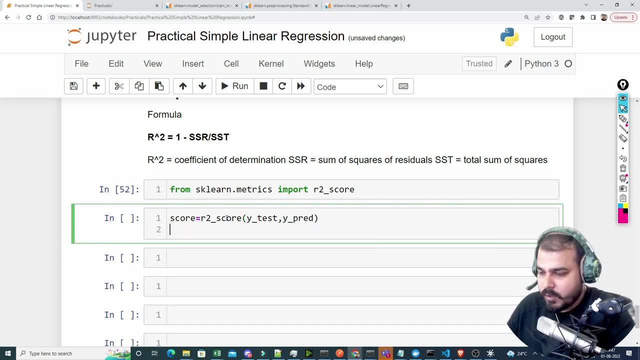 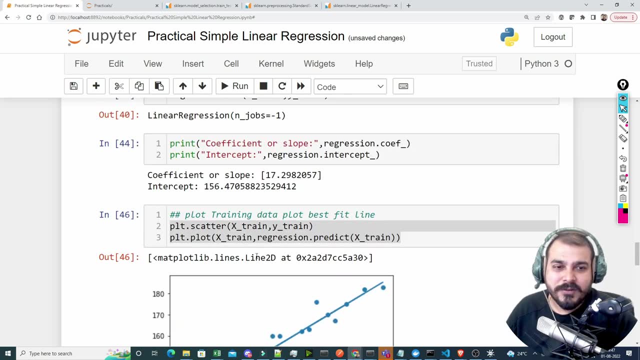 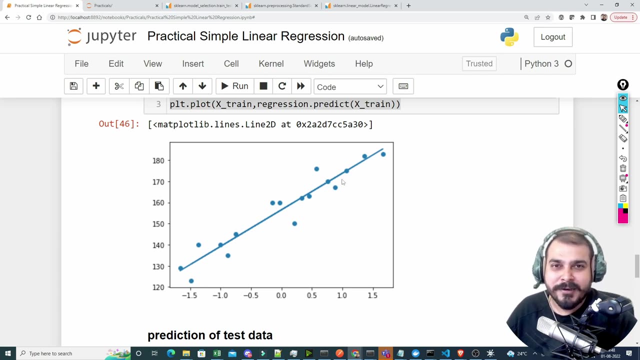 comma Y underscore pred right And if I probably print my score, this will be my R2 score and here I'm getting 73% And obviously you cannot get a perfect just by linear line. We'll be seeing how we can improve this by using some of the algorithms like polynomial linear regression, decision trees and all. 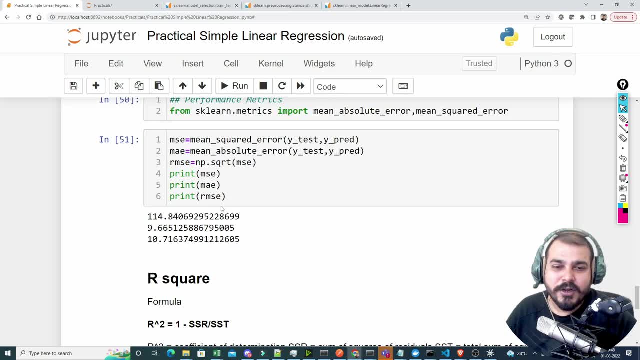 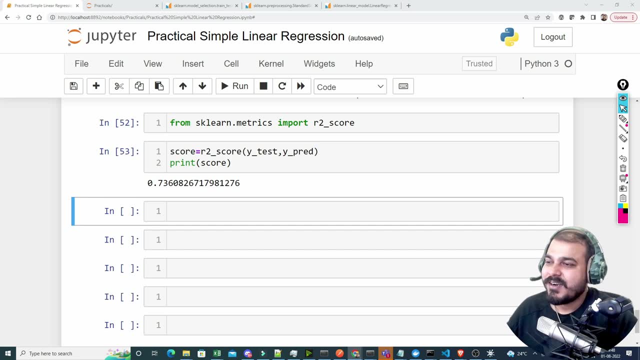 Many algorithms are going to come up in the further stages which will try to improve this particular accuracy, But right now I'm getting 0.73.. And obviously let's go and find out one more that is called adjusted R square. 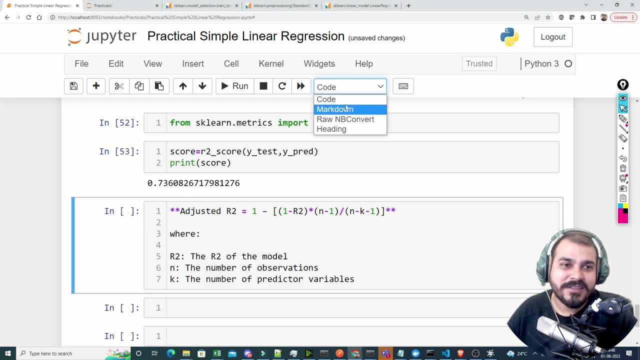 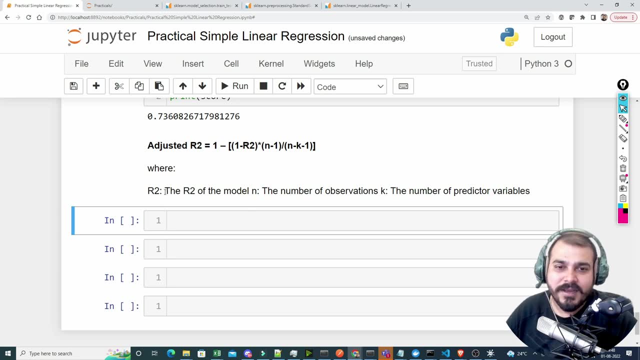 And, as you know, adjusted R square formula is this, which again I have discussed in my theory part right: It is nothing but 1 minus 1 minus R square multiplied by R2.. So it's going to be divided by N minus 1, divided by N minus K minus 1, right. 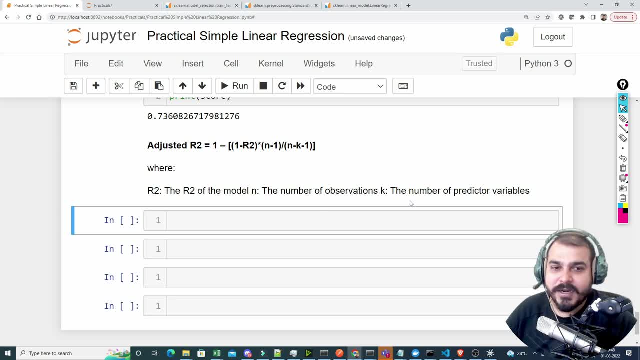 R2 is nothing but R2 score of the model, number of observation and number of predictor variables. right Right now I just have one predictor variable So I don't think so it will be such a big issue or big change in the score. 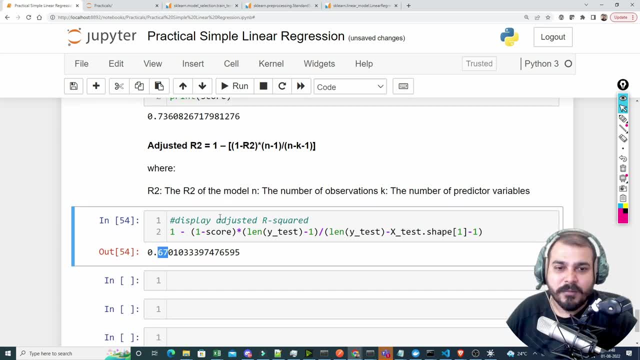 So if I probably go and see, it is like somewhere around 0.50, okay, So I've just applied this formula where I've written 1 minus score, length of Y test minus 1.. Y test is basically giving you the number of observation and all. 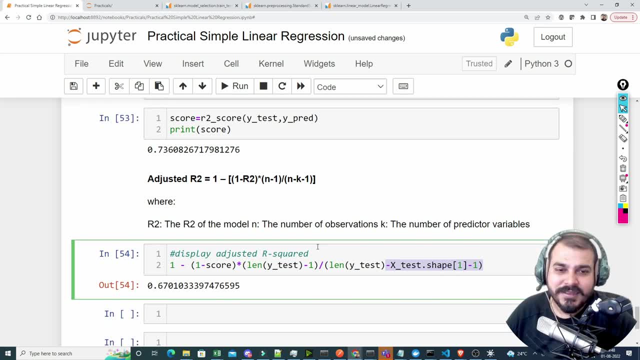 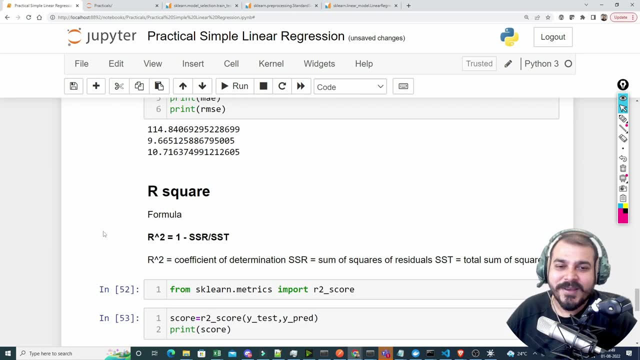 Y test, and this is your other thing, right? So, yes, I think I've covered all the most of the things over here. We have also seen that. okay, I've got 0.73, which is good. I've also seen all the performance metrics like: mean squared error, mean absolute error. root: mean squared error. 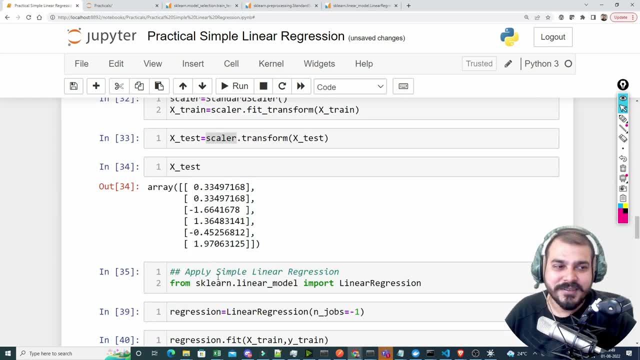 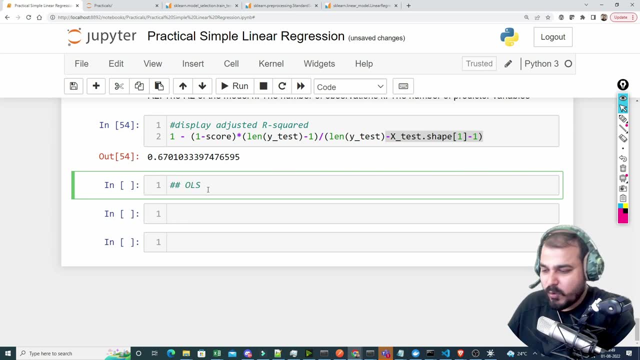 This is absolutely fine. We have done some kind of visualization, analysis and all. Now let's try to see one thing. Okay, let's try to do the same thing with OLS technique, OLS technique of linear regression. So can we get the same? because that formula that I derived right. 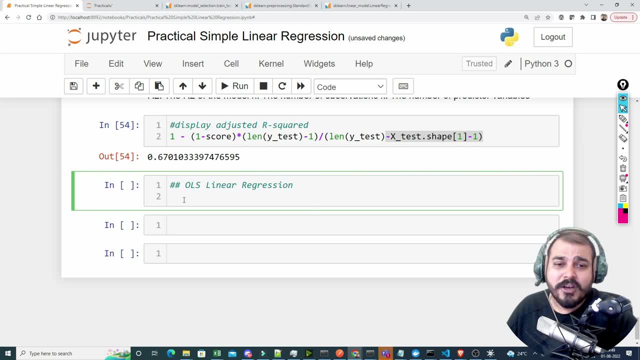 Can we get the same output that we are looking for? You know, in order to implement OLS, linear regression, I will say import stats models, dot API as SM. okay, And I'm going to execute it, And now I'll just use my model. is equal to this model? will this API that I'm actually using right? 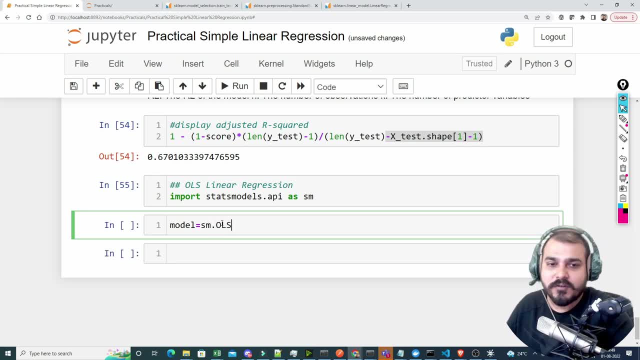 This library that I'm using, This has A library which is called as OLS, and you know, in OLS all we need to give is with respect to your training data. So if you probably go and see over here OLS, here you have something called as endog and exog, right? 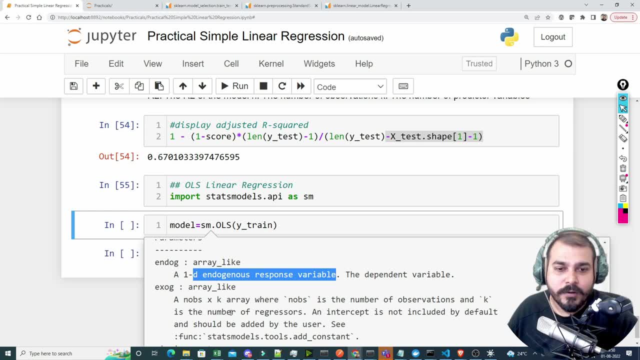 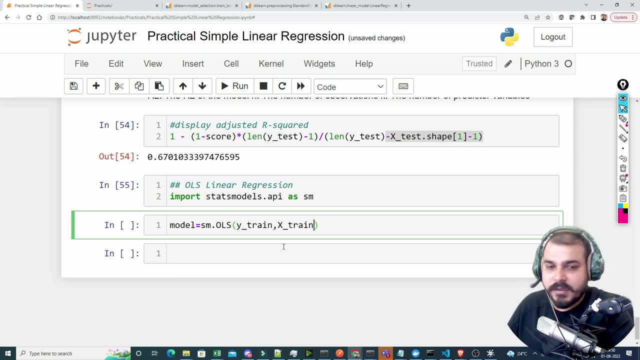 Endog basically means 1D- indigenous response variable. That is my output variable. Exog basically means my true input variable, right? So here I'm basically going to give my x-train and then I'm just going to do dot fit on this, like how we did for linear regression. 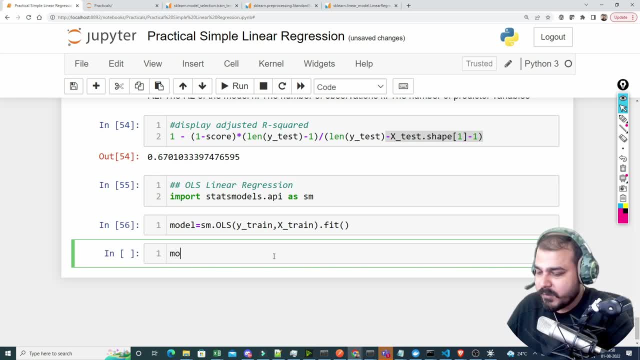 Once I do this, I will get my model and all I have to do for prediction. I will do model dot predict or x underscore test and this will basically give my prediction value right. This will give my prediction value. So if I probably execute this print prediction, you will be able to see the prediction also perfect. 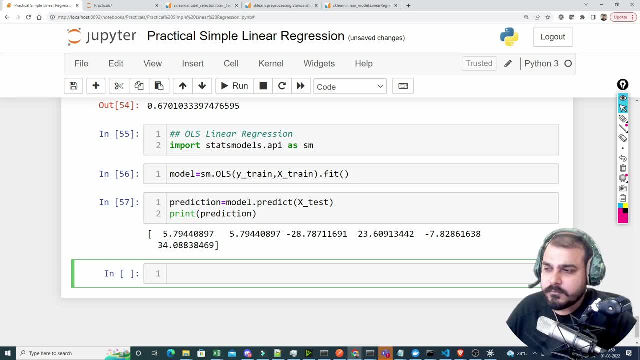 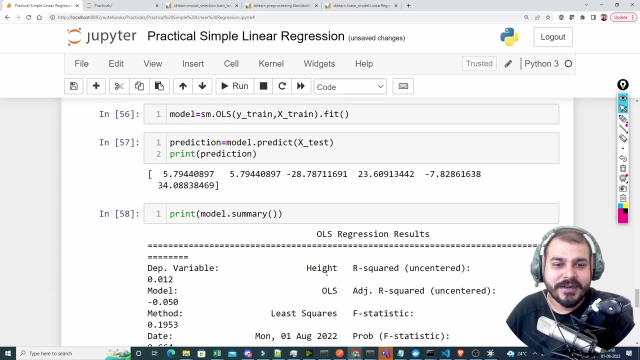 So these are my predictions. Now let's do one thing. Okay, I'm just going to print my model summary over here, Okay, Okay, In OLS and see whether I'm getting the same thing what I did with the help of linear regression using gradient descent. 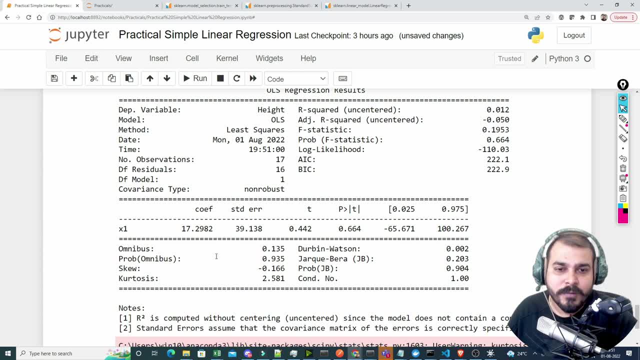 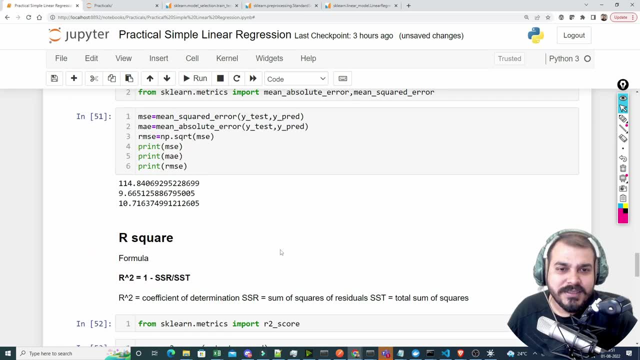 So again, I'm printing this now here. I'll just zoom out here. You can see that there is one feature x1 and it is having coefficient of 7.29. Now is this matching with this or not? We'll try to see. 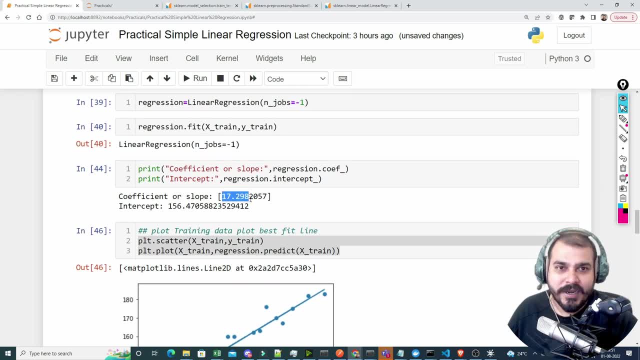 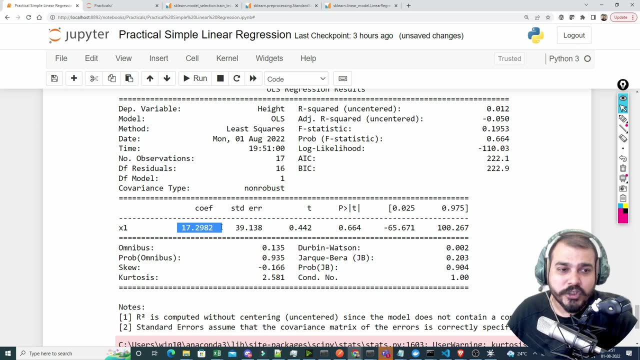 So if you go over here, here also I'm getting coefficient as 7.298, which is quite amazing. Now you can see The proof that, with the help of OLS also, I'm getting the same coefficient. And yes, there are some more parameters over here, right? 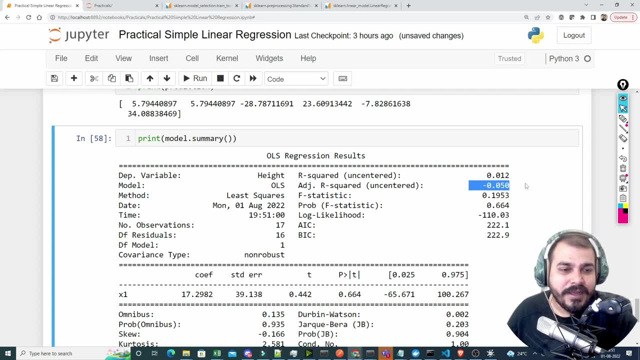 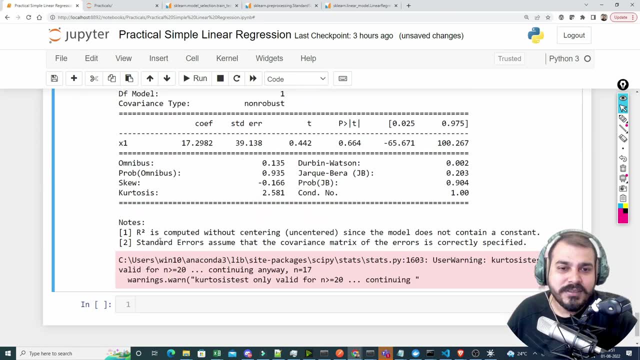 They are like R squared value, adjusted R squared value, right Statistics value, and this is specifically for uncentered centered data. It is not there, right? So all these things here. you can basically see that, but at the end of the day, we are getting a coefficient which is 17.29, right. 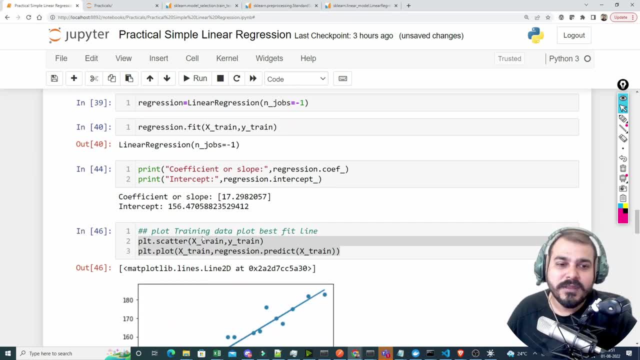 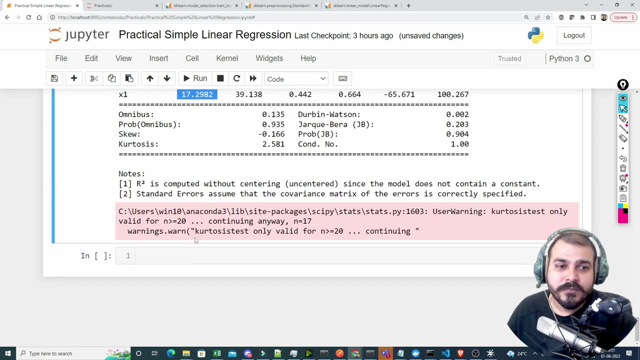 Which is approximately equal to this particular coefficient that we got with linear regression Okay. So this is the most important Point with respect to this. that basically means, with the help of OLS also, we are able to get some good values right. 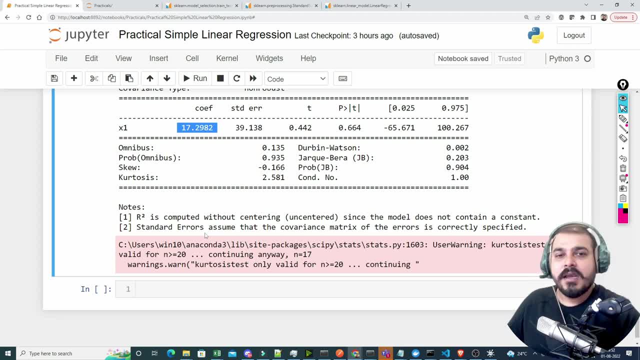 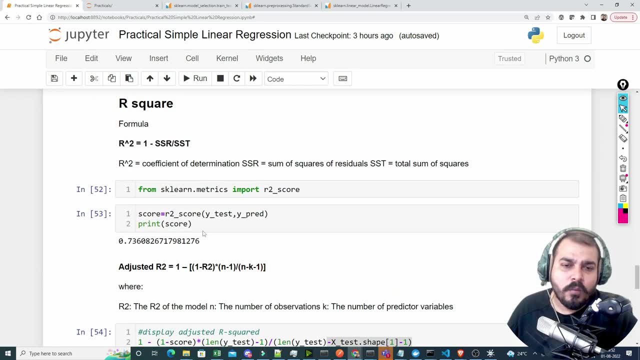 Good. good, because almost all OLS and this sklearn works in the same strategy. Okay, Now, till here, we have discussed about so many things right Now: what, how to do the prediction for the new data, So this is super, super important. 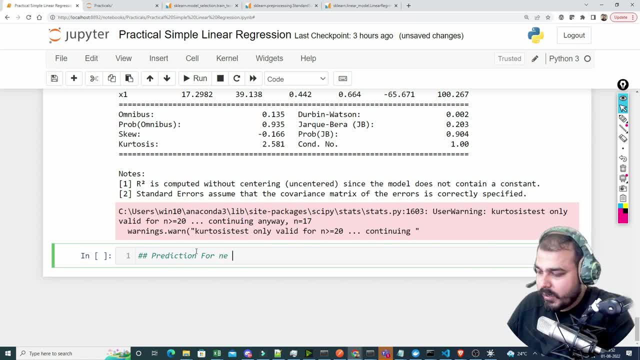 Prediction for new data. right Now, let's say that I get a new weight. Okay, let's say my weight value over here And in order to do the prediction, I will write regression dot, predict and my new weight value, My new weight value. always. make sure this you are providing in two dimension again, right? 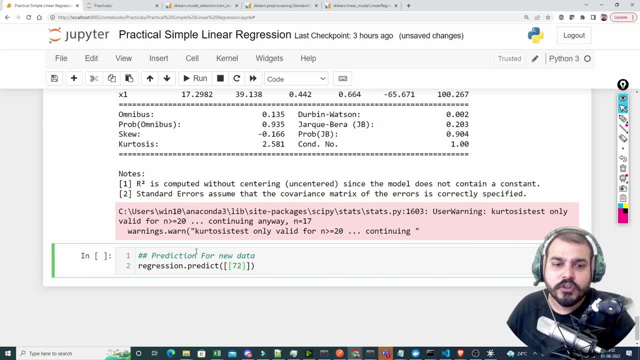 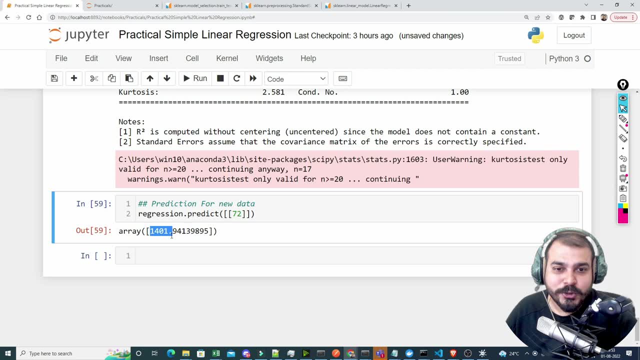 So it should be. let's say I want to predict it for 72 weight. What should be my output? So here you'll be able to see the output. Now, guys, here you can see that after prediction it is showing 1401.. 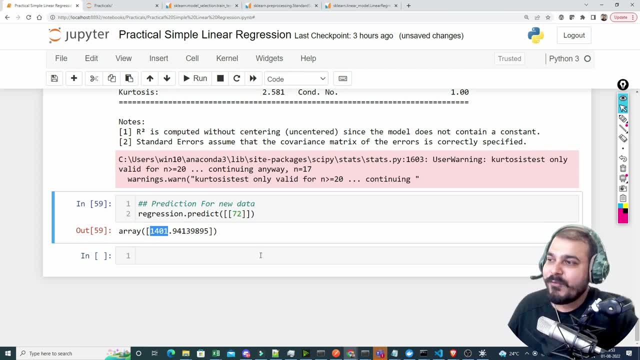 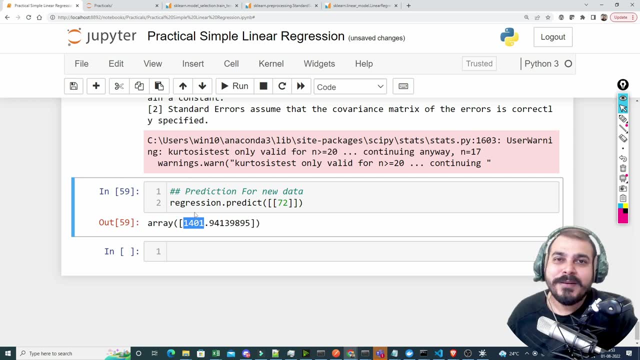 Oh my God. This basically means that a person who is having a weight of 72, is getting a height of 1401 centimeters. So what mistake did we? do You know why it is basically giving this kind of output? The answer is very simple, guys. 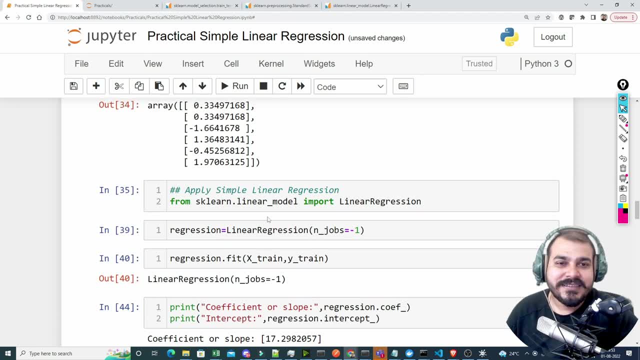 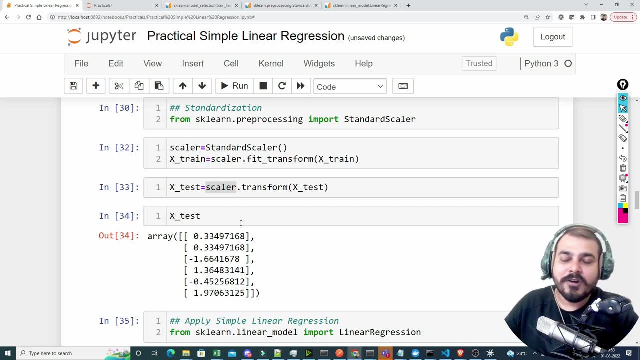 We missed a very important step, which is called as standardization. See, we did this standardization right, And right now, my data points are not, you know, standardized down or normalized in this particular range, right? So what do we do? 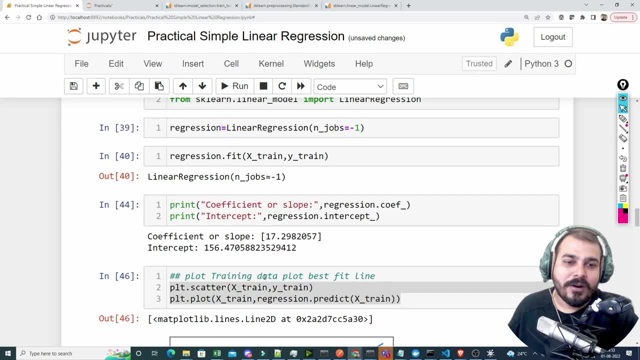 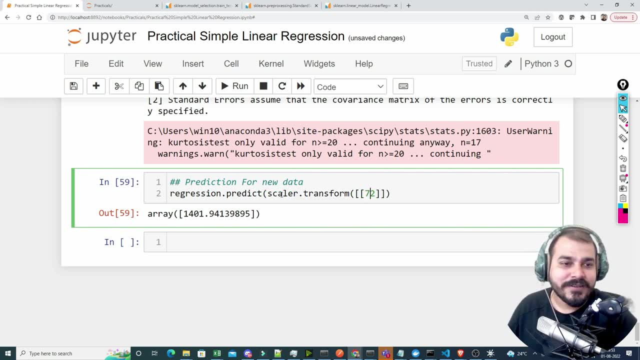 We will again use sklearn dot transform. So here I will just copy this and I will write over here: simple sklearn dot transform and I will give this value inside this. Now, once I give this value inside, then you will be able to see I will be getting a good value.